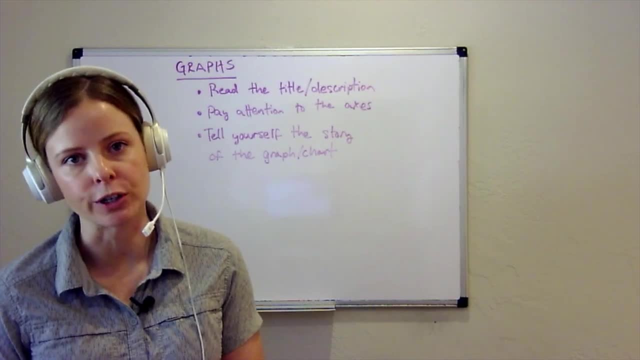 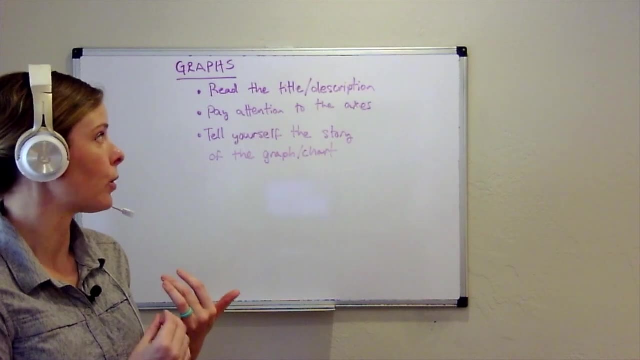 of time to orient yourself to that graphical information before you move on to the question, And what should you do with that time? A couple of things to consider. First is that it's important to read the title and description of the graph so you see what information 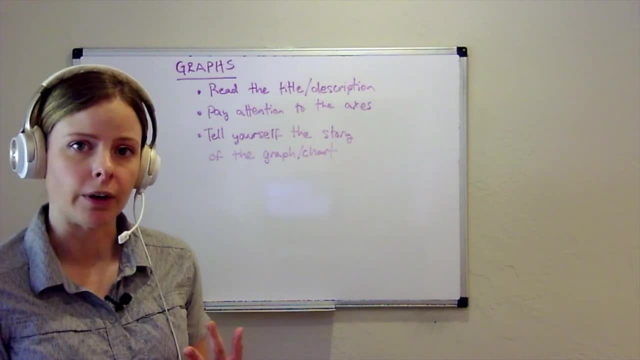 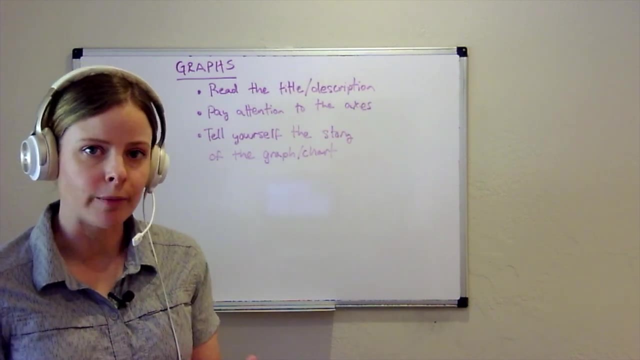 that gives you. Second, you want to pay attention to the axes and what exactly you're going to see is on each axis of the graph. And finally, you want to tell yourself the story of what information is presented on that graph. Give yourself a little bit of a narrative of okay. 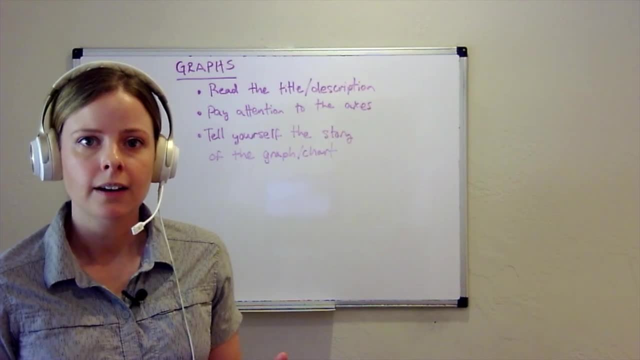 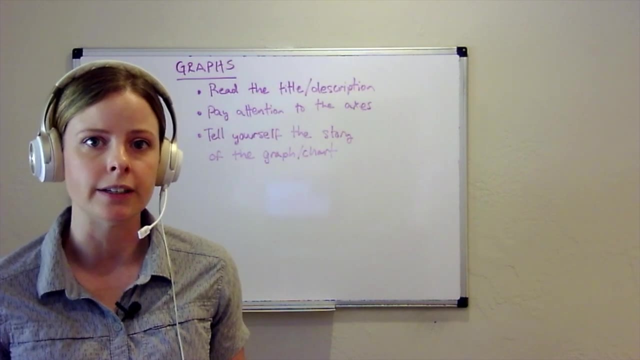 I see how this information all fits together, So we'll go ahead and give that a shot. What I will do is I'll put a line graph up on the board and I'll give you about 20 seconds to just do this. I won't put the actual questions themselves up, I just want you to orient yourself. 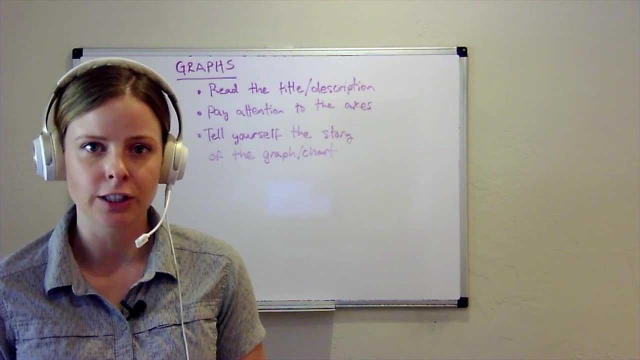 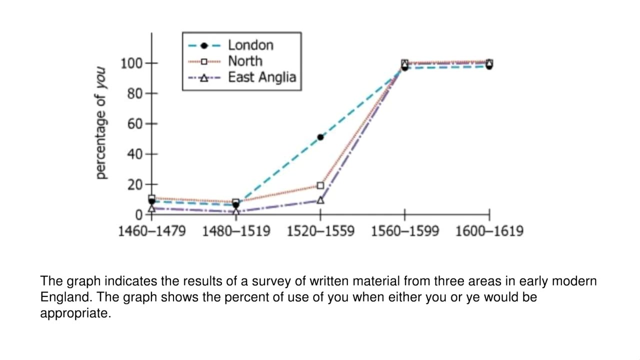 to that graph and see what information you can get from it. So I'll go ahead and pop that up right now. All right, so let's talk about this line graph Now. if you need more time, I'm going to go ahead and show you how to do that. I'm going 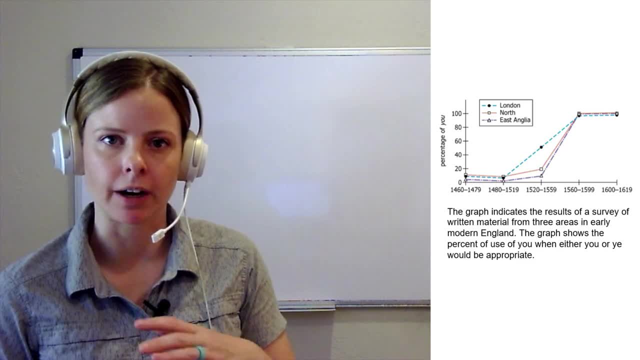 to go ahead and show you how to do that. All right, so let's talk about this line graph Now. if you need more time, you can always go back to that previous screen and pause for as long as you need to, But otherwise let's chat it through So you can tell that. 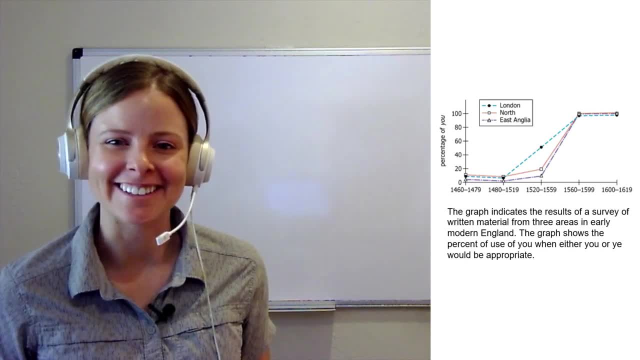 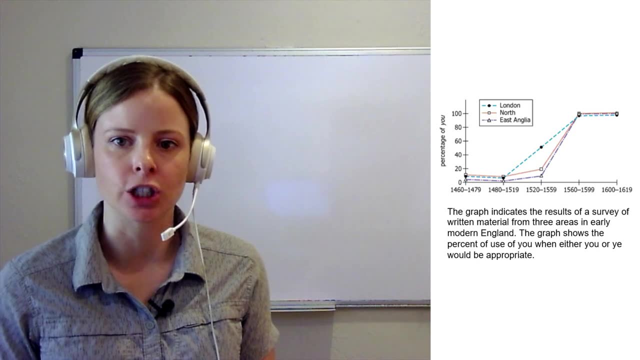 this is a line graph because it's got lines, so nothing too crazy going on there And here. if you look at the axes, we have some dates along the bottom That's pretty easy to interpret. We're just showing from kind of the mid-1400s going up to the early 1600s, something that's 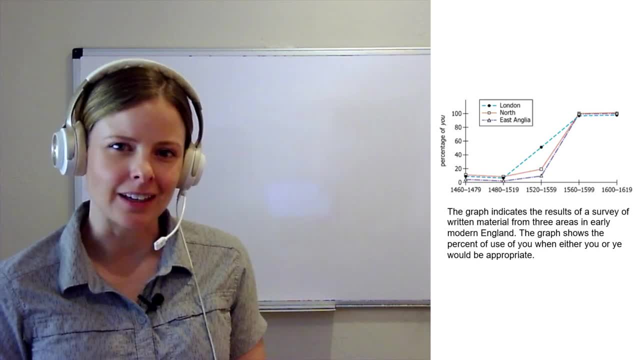 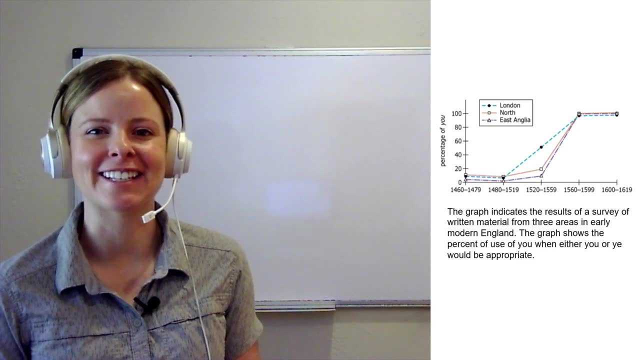 changing over that period of time. I think that the other axis is difficult to understand until you've read the description. So it says: percentage of you. What the heck? What does that mean? I don't really know. So let's go to the description of the graph to figure. 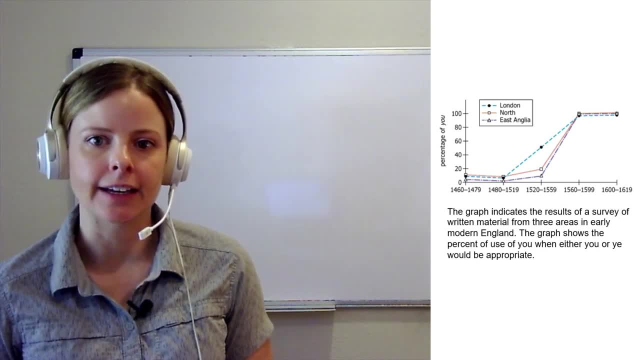 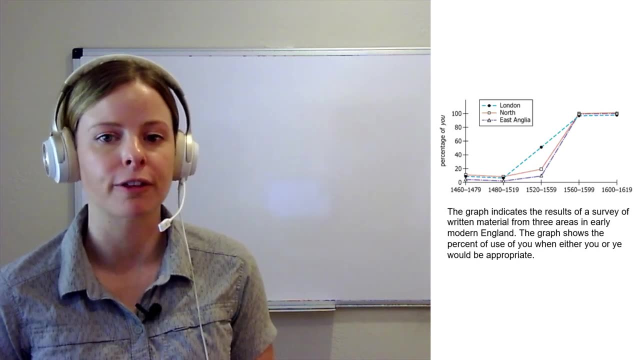 it out. The description says that the graph indicates the results of early written material from. sorry, the graph indicates results of a survey of written material from three areas in early modern England And then, if you look at the key, we've got these three areas London. 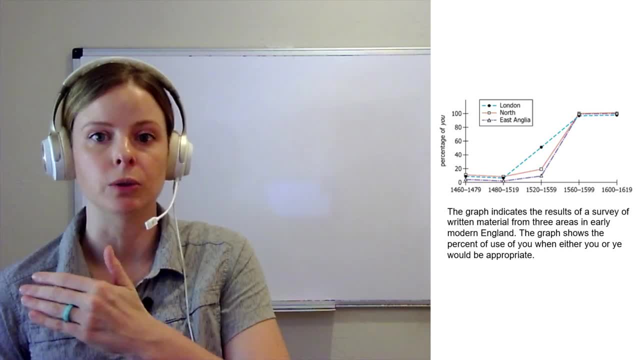 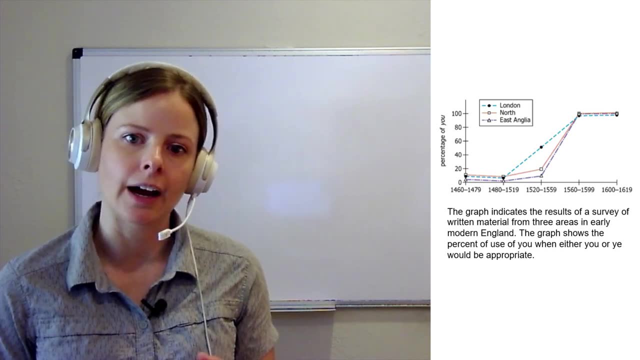 North and East Anglia, And each of those three corresponds to a different line on our chart. So that makes sense. Then we're told the graph shows the percent of the use of you, when either you or ye would be appropriate. So I guess there are some cases in which you could either say you: 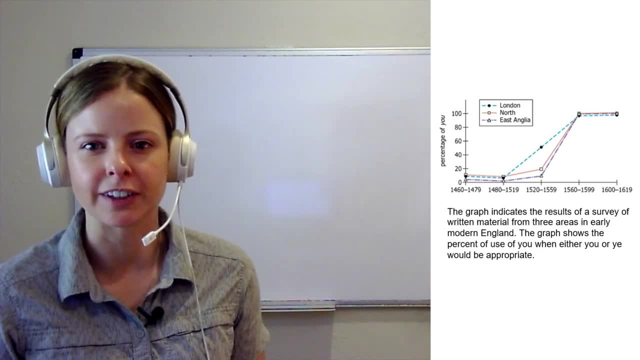 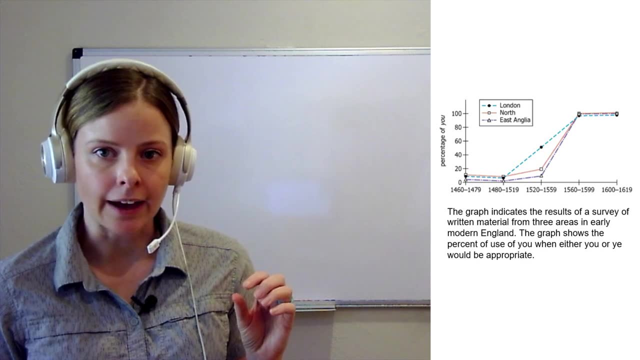 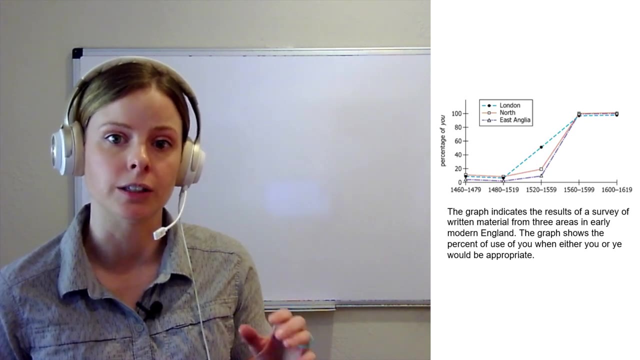 or you could say ye, like ye olde Mary Tavern or whatever, And what we're shown in this graph is: how often are you choosing to say ye? Now, looking at this overall story, then what we see is this shift of very few people using you at the beginning. right, So we're subpoenaing. 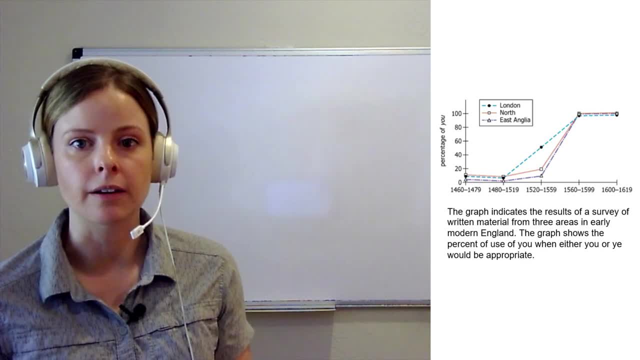 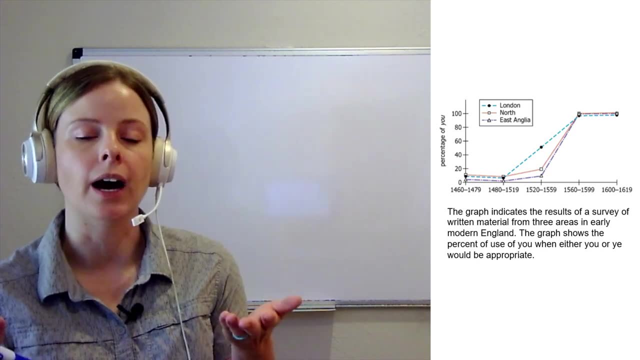 like 20% of the time using you when you could use ye, And then, as the graph goes to the other side, then we see that that percent of you goes way, way, way up, pretty much to 100% by the time you. 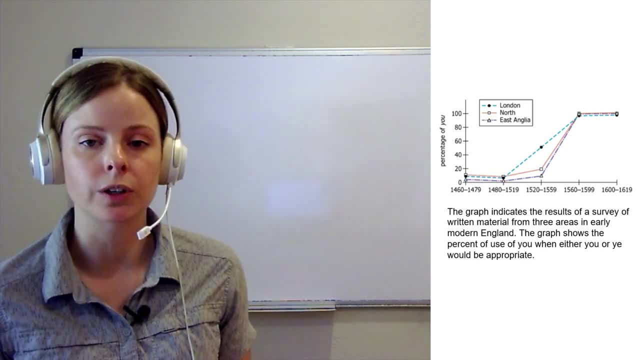 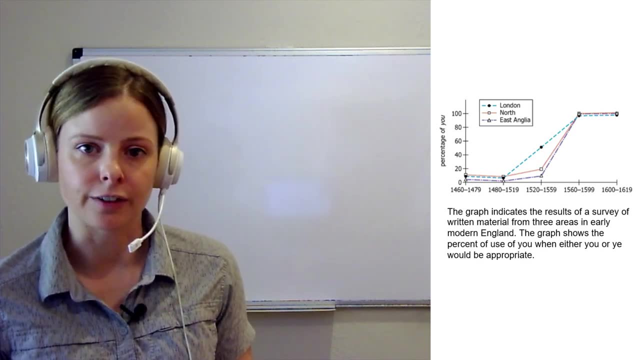 get to the end of the graph. So over time, the story that's being told here is that most people used to say ye, and then things changed And by the end most people use you for about 100% of the times that they could use easier use either. 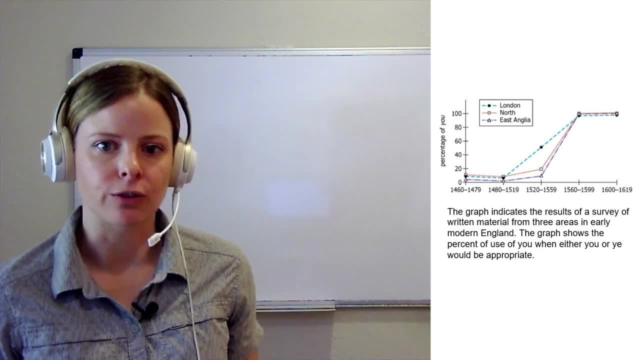 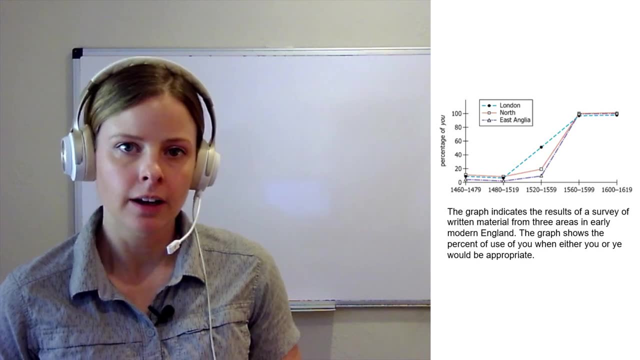 That's the overall story of this graph Seems pretty straightforward, And so now is the time when you can go ahead and dive into the questions themselves. So I'll go ahead and I'll pop those questions up here. There are two questions. I'll give you a couple of minutes to answer those two. 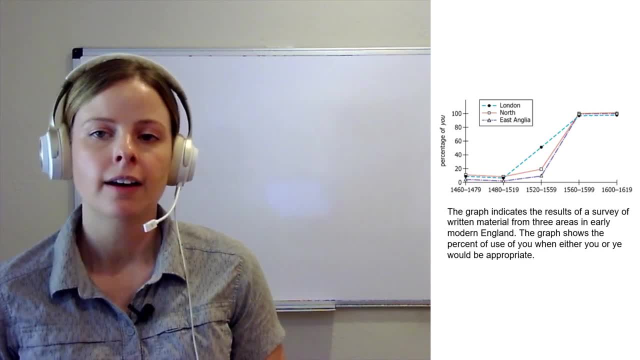 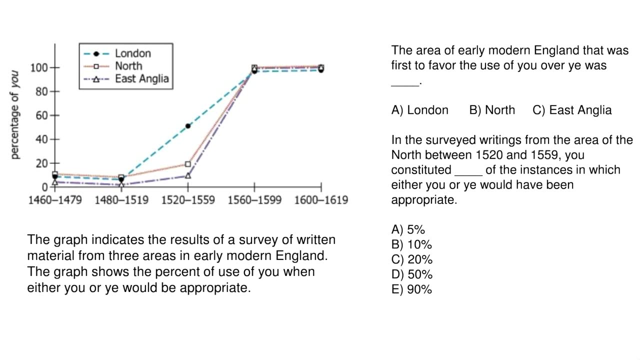 questions And, as always, if you need more time, feel free to pause and then we will chat them through. Subtitles by the Amaraorg community group: wwwamaraorg. Subtitles by the Amaraorg community. All right, let's go ahead and talk through these two questions. So the first question asks: 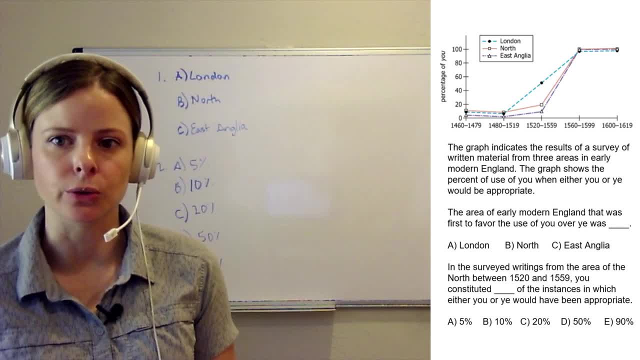 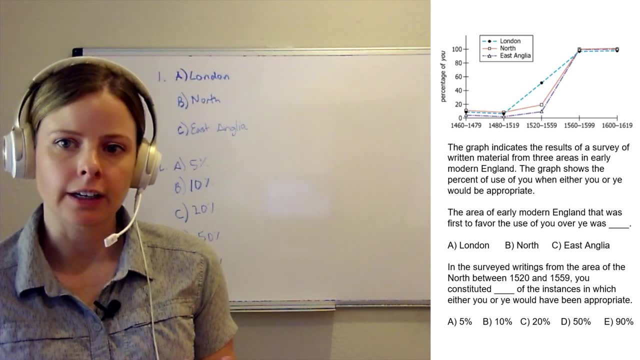 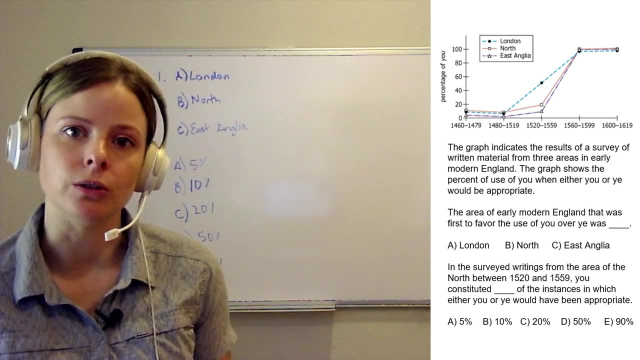 the area of early modern England that was first to favor the use of you over ye was London, the North or East Anglia. which one? So here I'm looking at first to favor the use of you over ye. What does that mean? Well, that means that you're more likely to use you when you could use either. 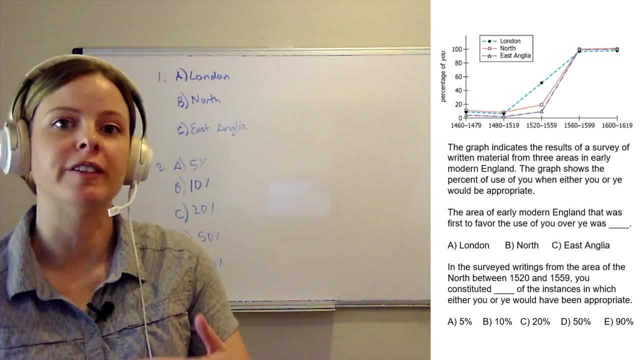 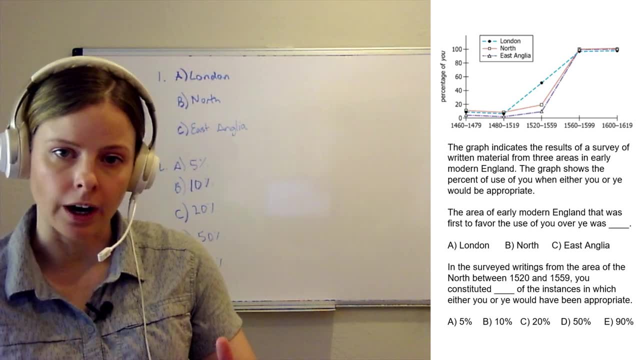 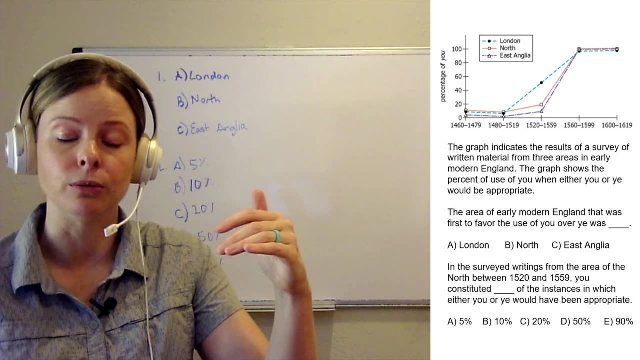 In other words, that percentage of you should be above 50% if you're favoring you over ye. So this is a pretty simple question And all we do is we go up on the y-axis to see: hey, you know where's that 50% mark where we are starting to favor you. 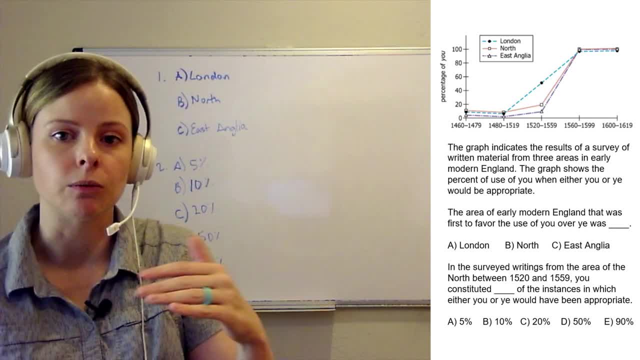 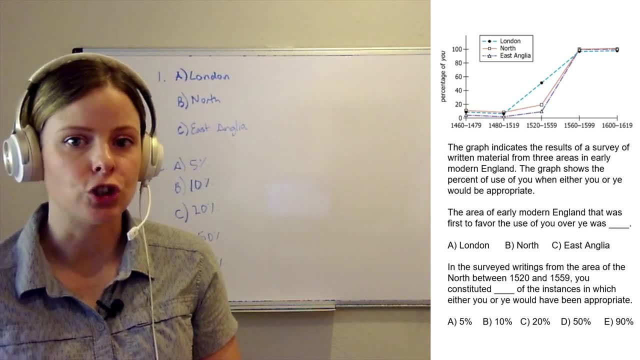 And then just track it along across the line and see, well, who was first of these three lines. which one crosses that horizontal line at 50% first And if you just do that, go up to that 50% mark, which isn't marked but it's just going to be between the 40 and 60. And just trace it across. 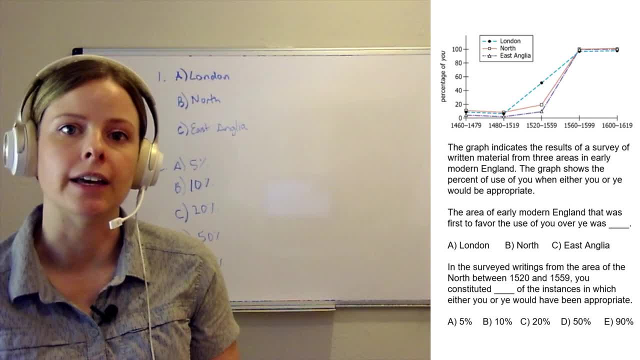 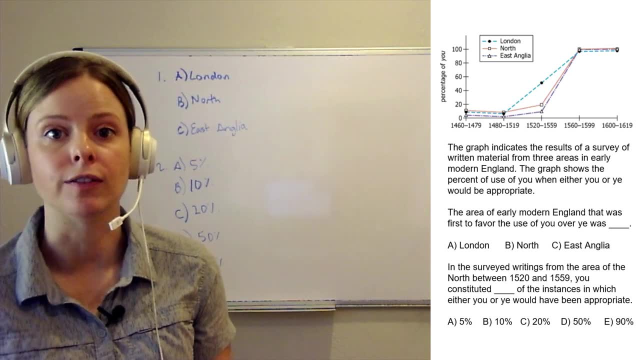 with your eyes, you'll see that very, very clearly. the London line is the first to intercept Subtitles by the Amaraorg community, with that 50% line, which tells us that London was the first area that would favor the use of you over. 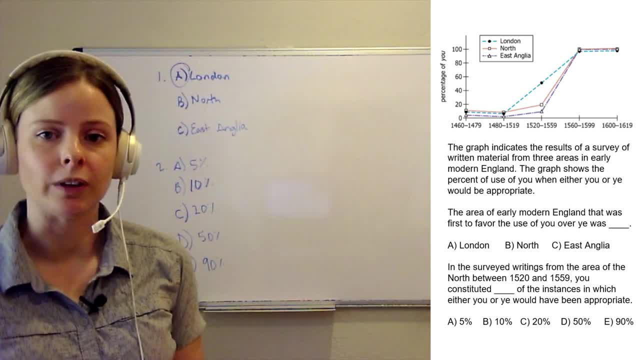 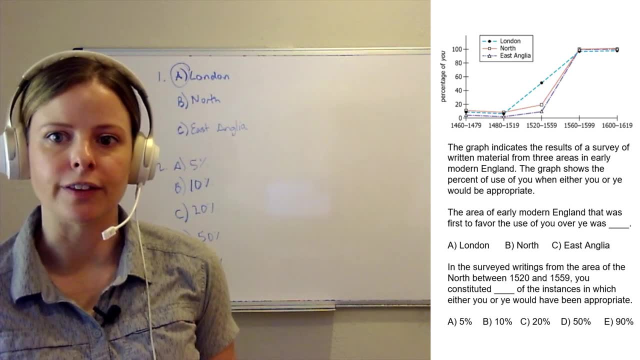 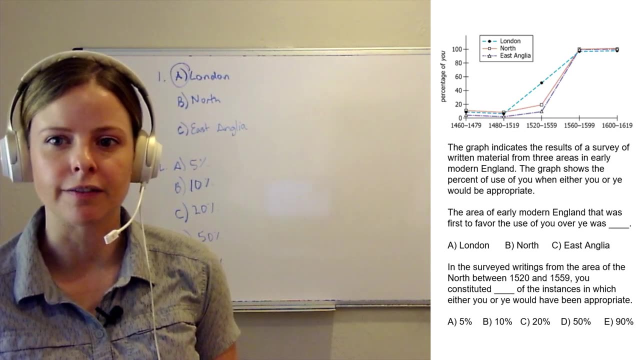 ye. So the answer to question one will be a London. The second question asks: in the surveyed writings from the area of the north between 1520 and 1559, you constituted what percent of the instances in which either you or ye would have been appropriate? So now we know that we're looking at the north. 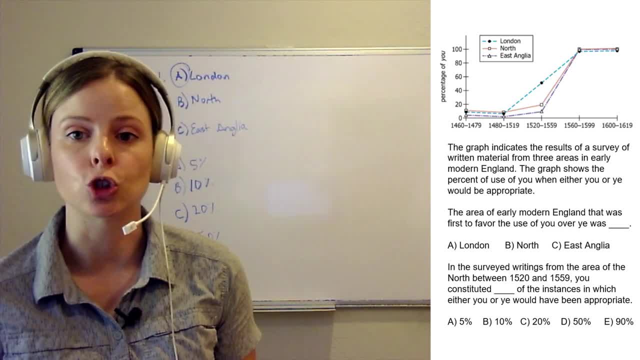 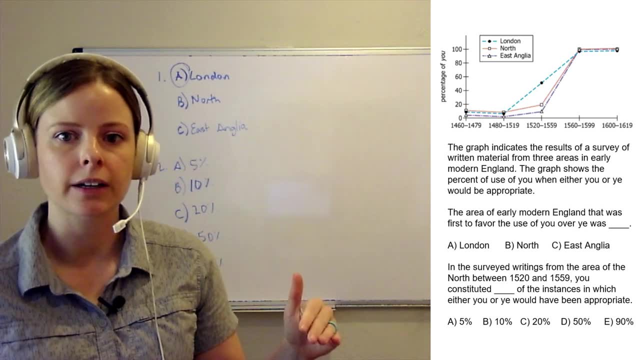 So go to your key, take a look at which line, and we're looking for that orange line And we are looking specifically between 1520 and 1559.. So just look on the bottom axis and get to that point: 1520 to 1559. And we're. 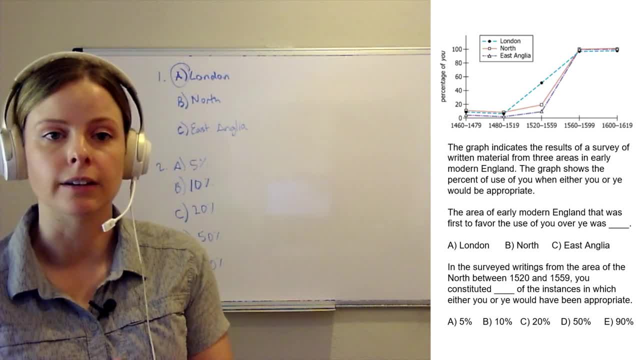 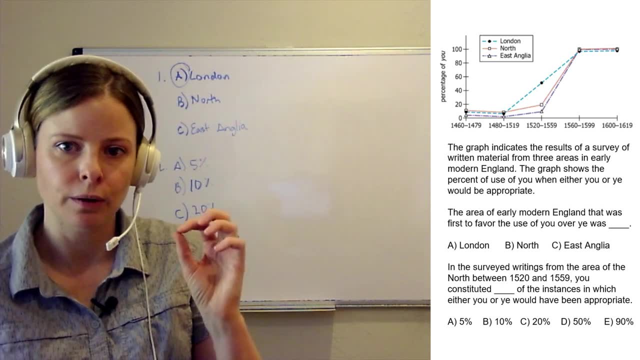 looking just for a percent where you would use you instead of using ye, And that's exactly what we're shown on our y axis. So at that point, orange line 1520 to 1559,, what percent are using you? 20%. 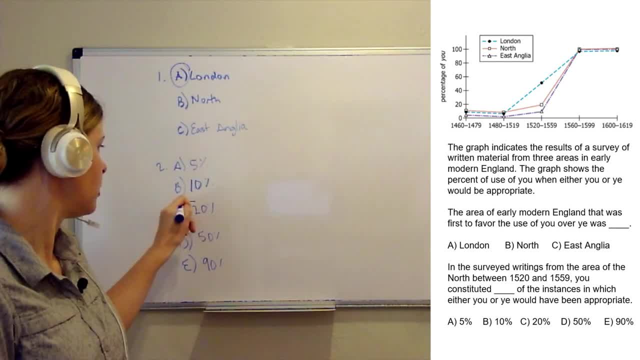 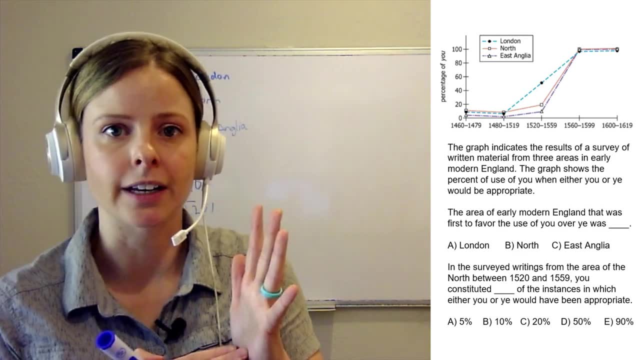 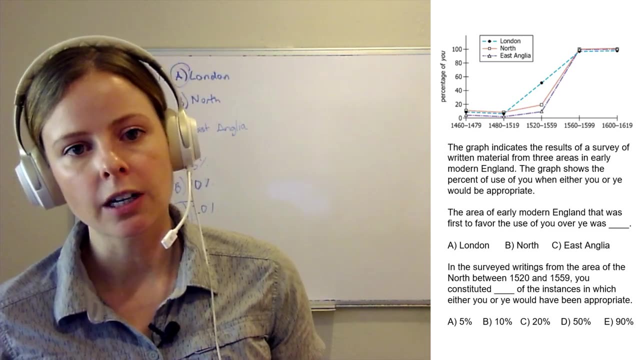 So that is our final answer for question two: see 20%. So that's a line graph. you know, it's just going to show two axes that are related to each other and what happens with your data as you change both of those axes. We will next go ahead and 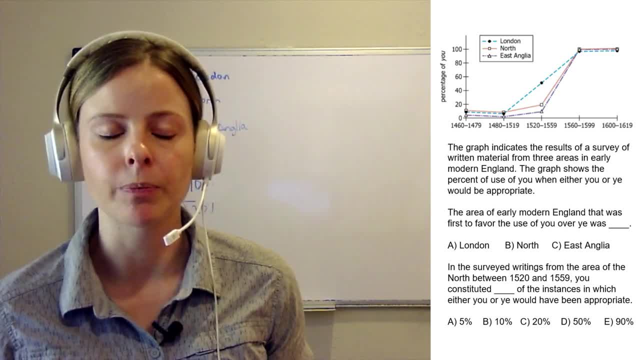 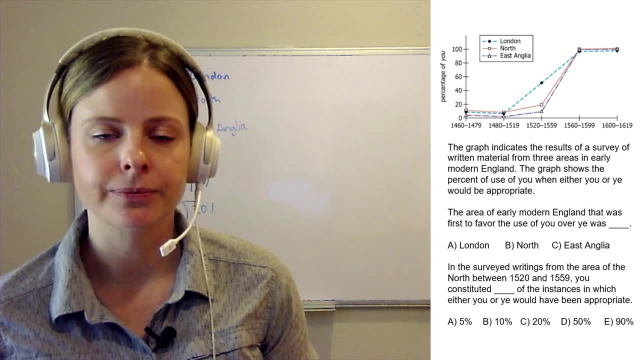 look at a bar chart and the overall approach remains exactly the same. First spend time with the chart itself and orient yourself to the information there before you dive into the questions. So again, I'll give you about 20 seconds to go ahead and read the description of this graph. 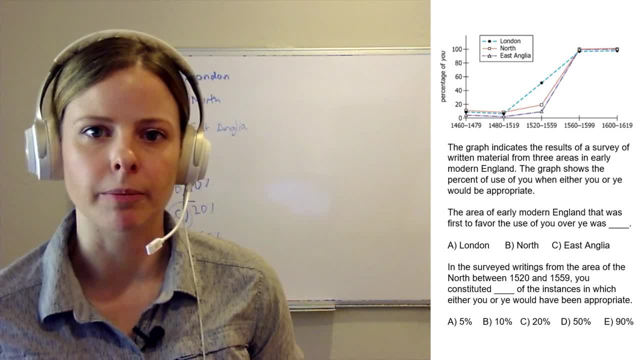 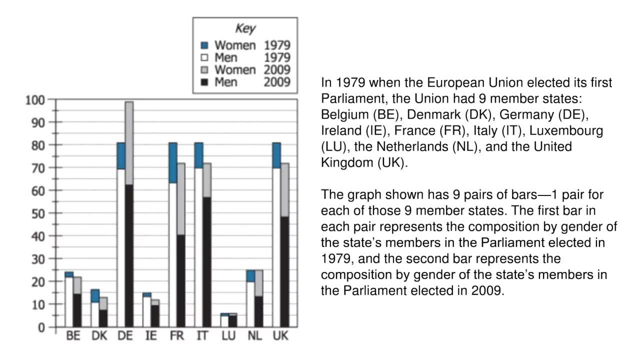 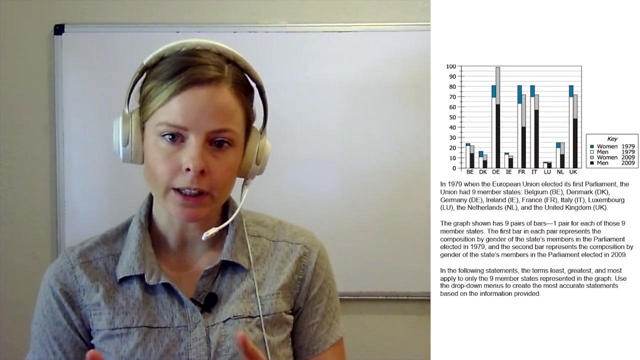 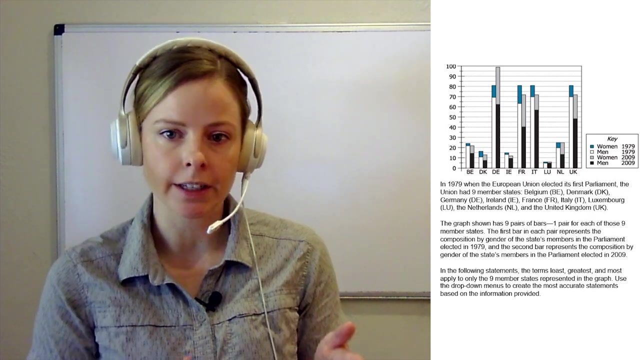 take a look at it And then we will chat about the graph itself, And then we'll go through some of the questions. All right, let's go ahead and discuss this bar chart. So what it looks like is that we've got some letters on the bottom- B, E, D, K, etc. And then with each pair of letters comes a pair of. 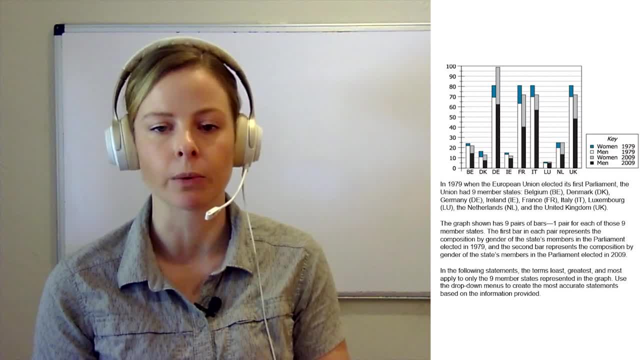 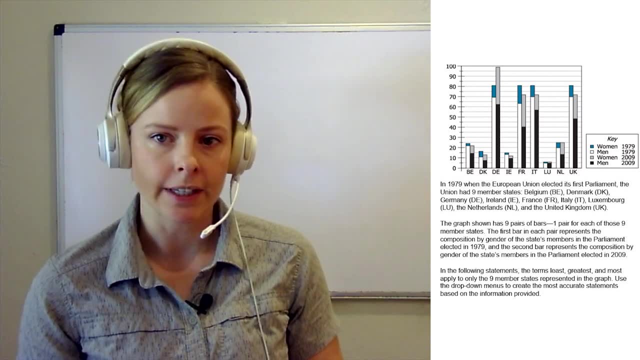 bars. So we've got two bars that correspond with each of these things along our bottom axis. I think it's easiest again to start with the description here. So it says: in 1979, when the EU elected its first parliament, the union had nine member states. So we've got 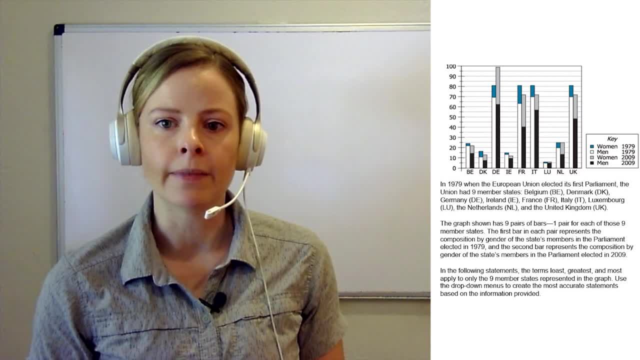 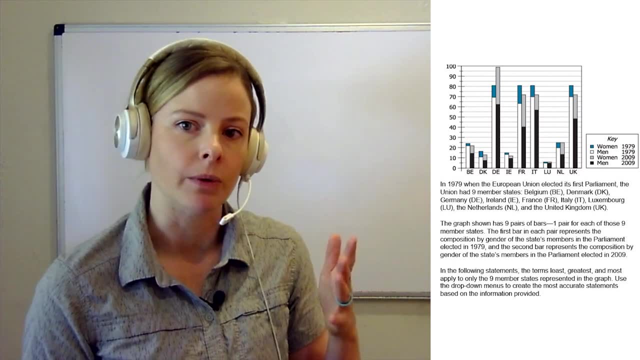 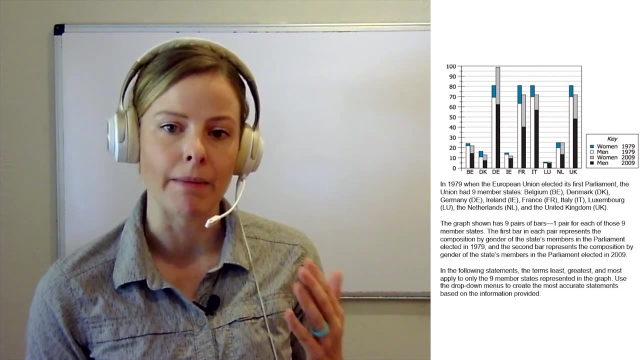 those nine member states listed on the bottom, And then the graph shows nine pairs of bars, one for each of those nine member states, and talks about what happened with that parliament in 1979 and in 2009,, with also breaking down the men and the women in each parliament. 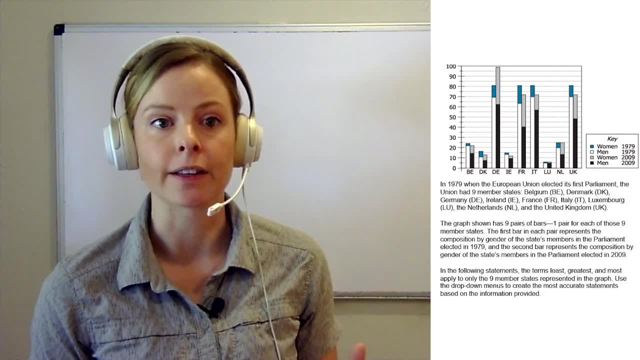 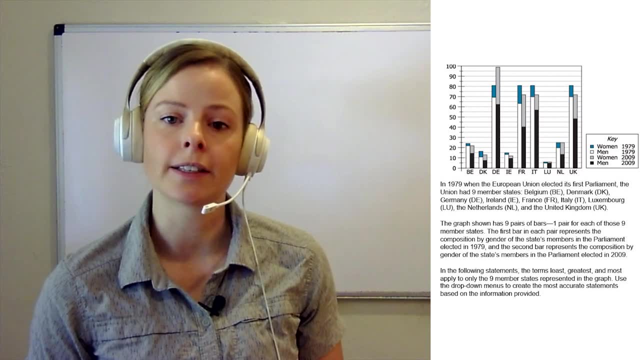 So this is when I might just choose one data point to go in and tell myself that story of what's going on. Let's just start with Belgium, just because it's the first one that is listed. What shows us is that the number of people in the parliament was a bit higher in 1979 than in 2009,. 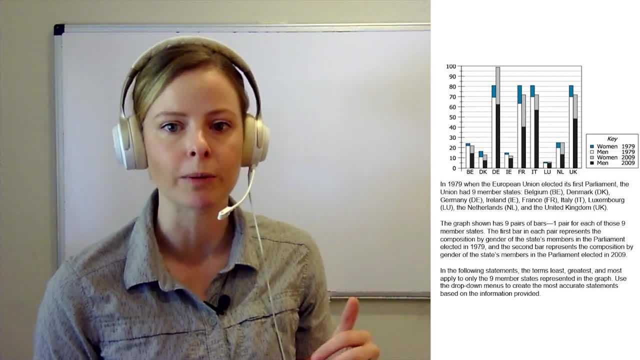 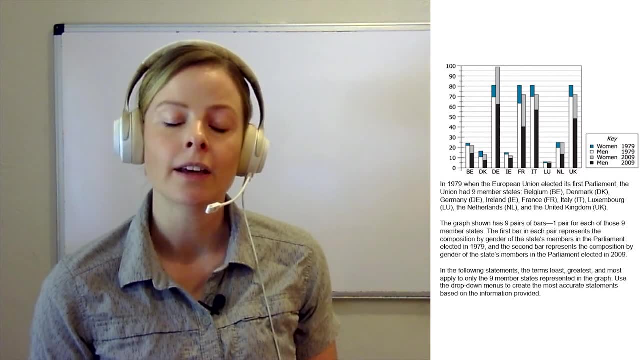 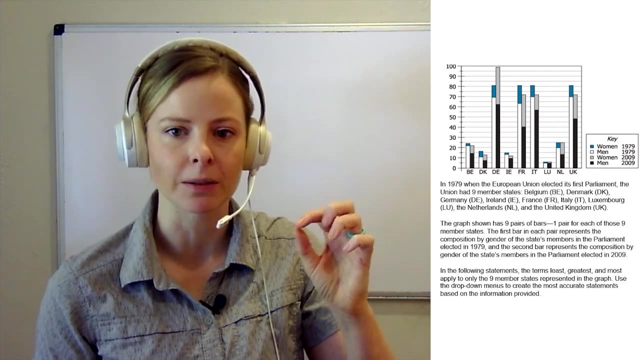 right. So it looks like that blue and white bar goes to about 24 total people and then the black and gray goes to about 22 total people, But that the number of women was much lower in 1979 than in 2009.. You know, that little blue square at the top of that bar is pretty small. 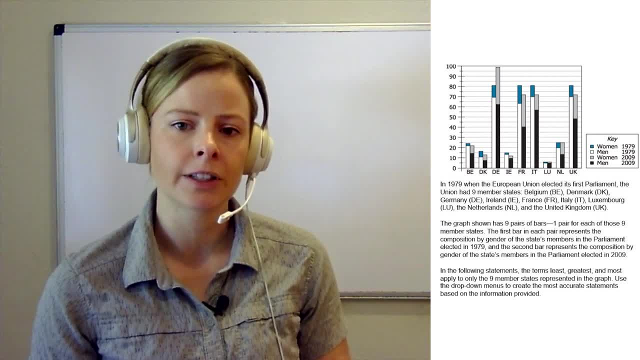 and then the gray square is just a little bit bigger. So you know, overall kind of gives us a sense of what's going on in the parliament, And then of course we have a little bit more of a sense of how many people were in the parliament and how many of them were men versus. 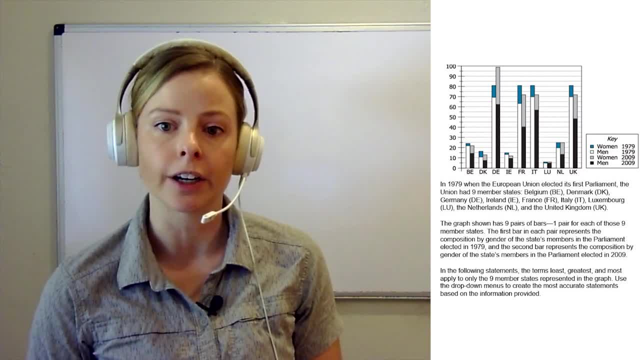 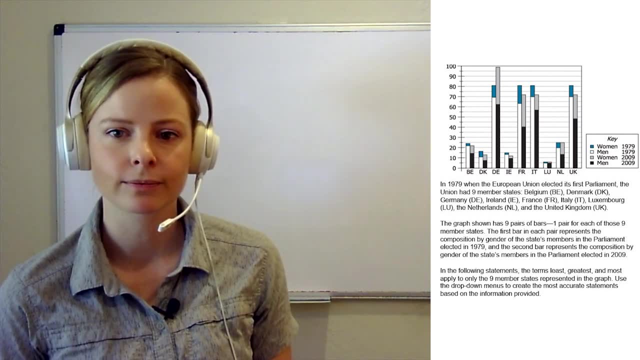 women. And then, of course, you can look across the other nations and see what was happening with them: Same sort of data being presented, but a different story for each one. So now that you understand the graph itself, let's go ahead and answer some questions. 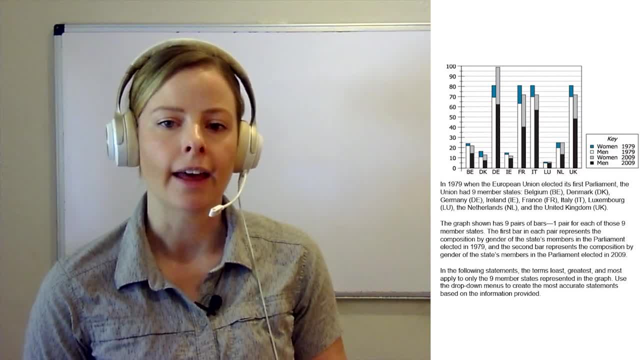 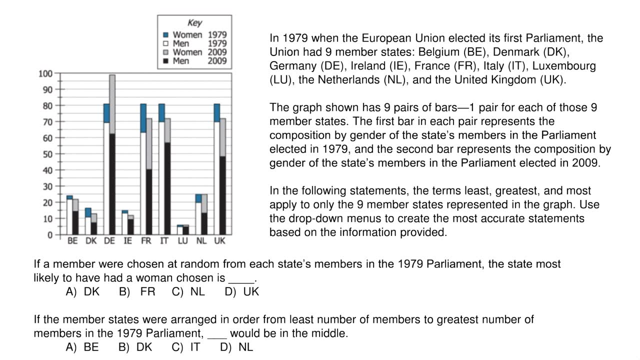 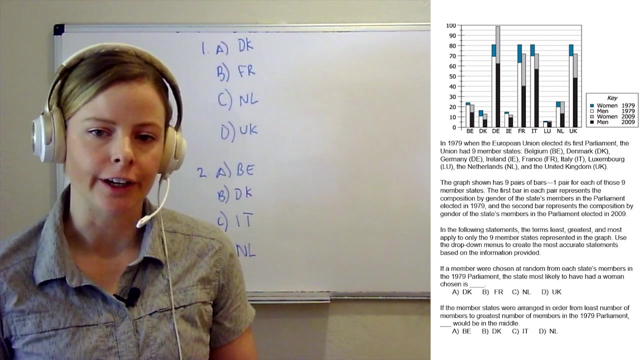 I will put them on the screen. There are two questions this time, And take your time, answer those and then we will discuss after a couple of minutes. All right, Thank you very much, you, you, you. all right, let's go ahead and talk through these questions. so if you need more time, feel free to. 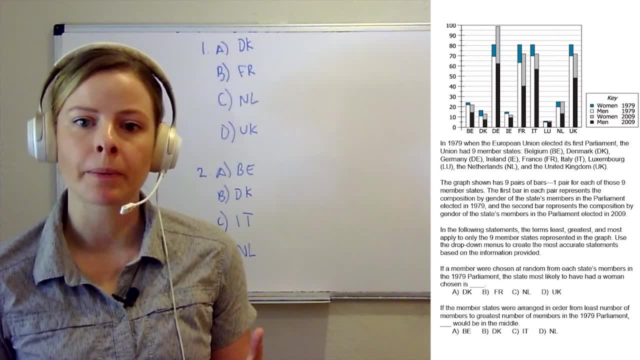 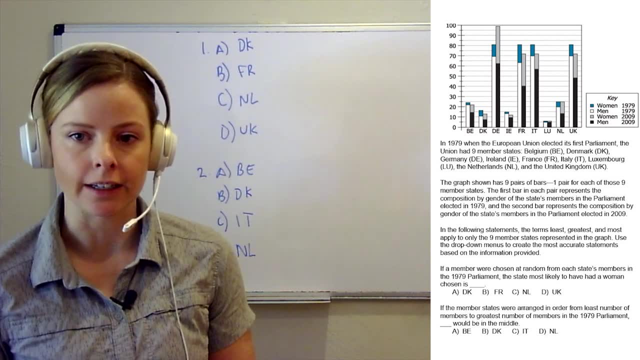 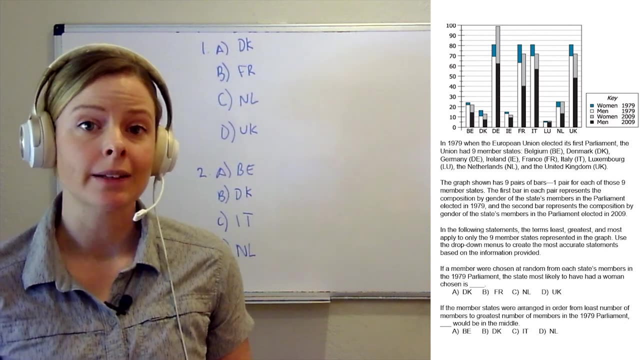 go back to the previous screen and pause for as long as you need, um, but let's dive in. so the first question asks if a member were chosen at random from each state. members in the 1979 parliament, the state with the most most likely to have had a woman chosen is like. so that's asking about. 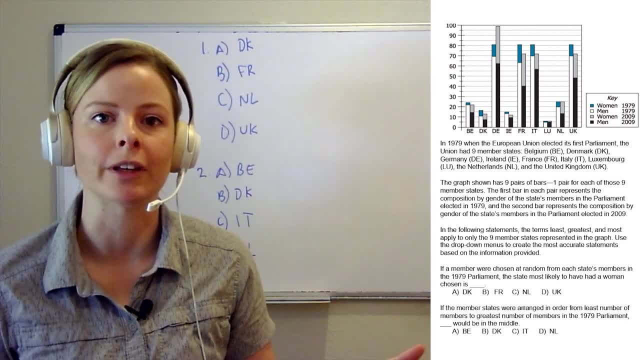 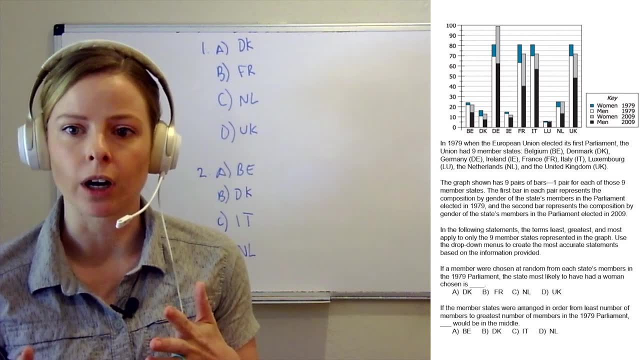 proportionality, right. so it's asking: you know, if i select from this whole population, um, where am i most likely to pull a woman out of that pool? um so, and we're also specifically talking about 1979, which tells us that we're dealing with the white and blue bars and we don't really care about the 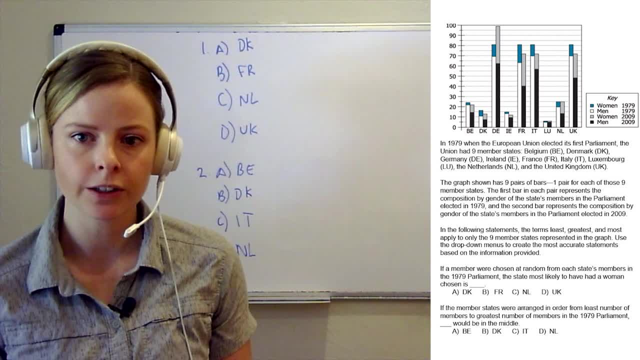 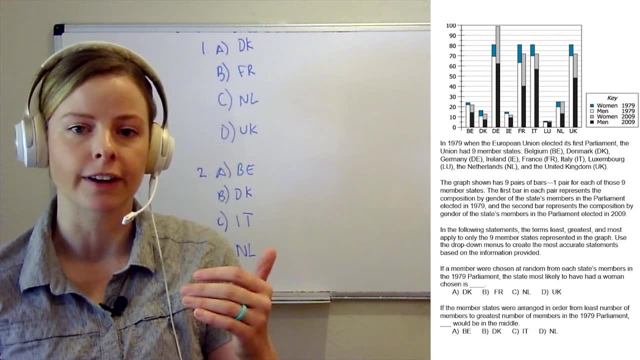 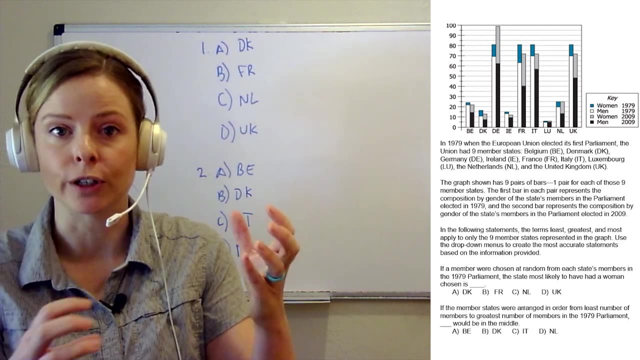 black and gray bars for this particular question, so you could go through each and every one of these options and see what your total number of people is in the parliament and then how many women you had. put those as a fraction right, so you've got your total number of women over your. 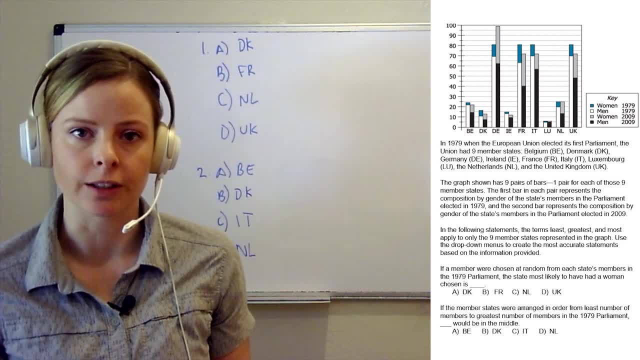 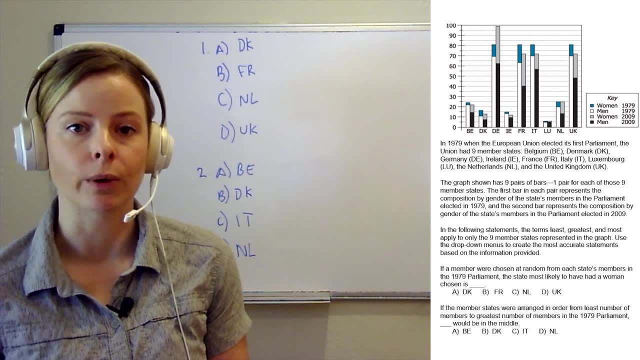 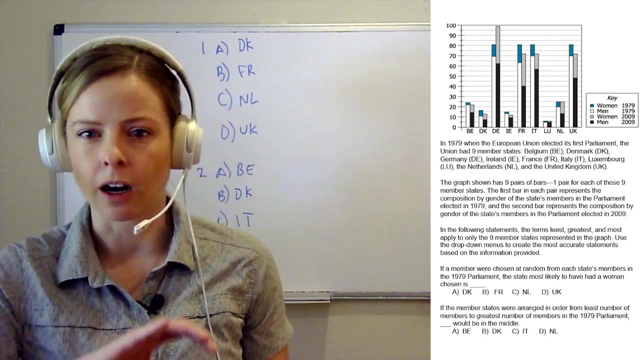 total population, um, and then compare all of those fractions to one another. to me that's just kind of a lot. i don't really want to do that for my four options. so let's see if we can make any quick comparisons just visually using the information in the chart. so the easiest ones to compare for me are those. 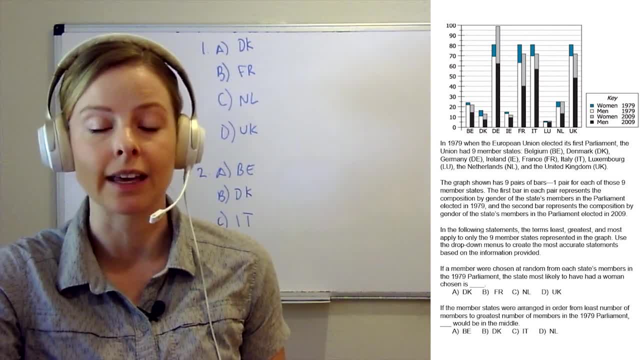 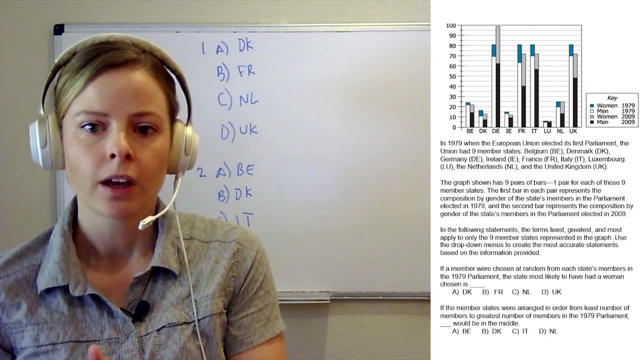 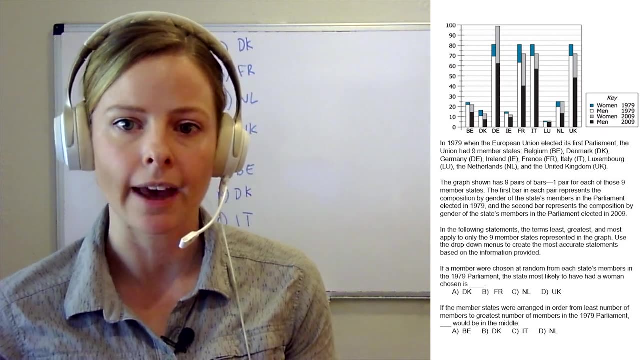 tall ones because they're all, if you see, roughly at that same level, right? so we've got the same total population, roughly, uh, in each of those four countries. um, and then, out of those uh, four countries, it looks like in our options, we have france and we have the uk, so between france, 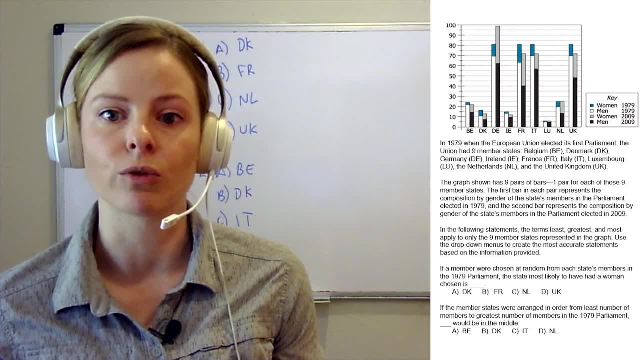 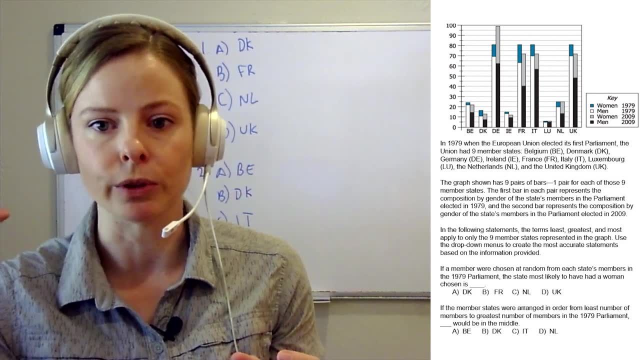 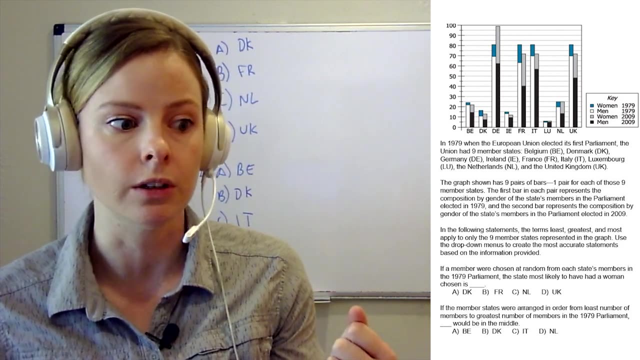 and the uk, which one proportionally has a higher number of women. well, it looks like that blue chunk in the france bar is much bigger than the blue chunk in the uk bar and again, the total population is the same. so we can say, hey, yeah. if i was to choose just between those two, i'm more likely to 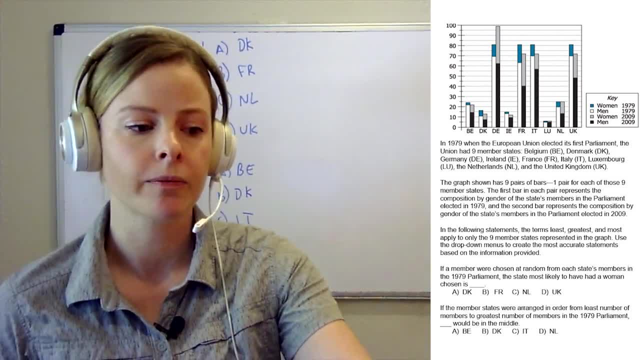 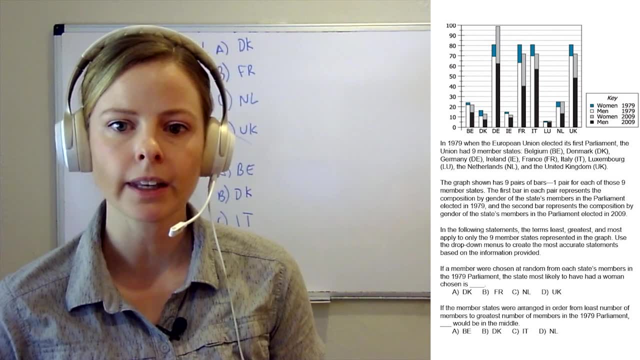 end up with a woman if i choose in france versus in uk. so that means that the total population is higher than the dk population. so that means that i can just go ahead and get rid of uk without really doing uh much math at all. same thing with my shorter bars. now i'm looking to see: hey, can i make? 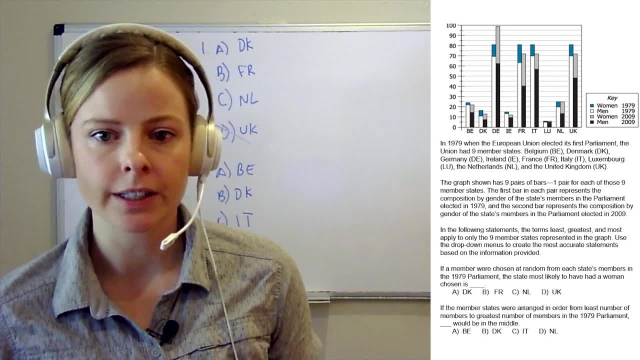 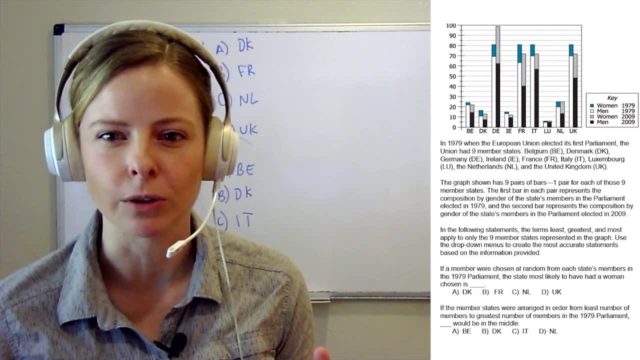 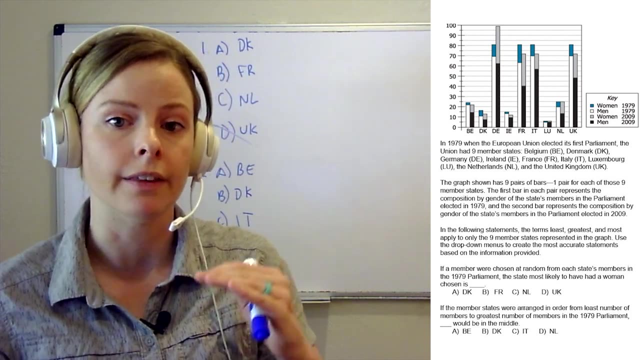 any eliminations, just visually, instead of putting exact numbers in and out of my shorter bars. i'm dealing with dk and with nl, so let's take a look. if i look at dk and then i compare to nl, what happens there is, the total populations are different. right, the nl population is higher than. 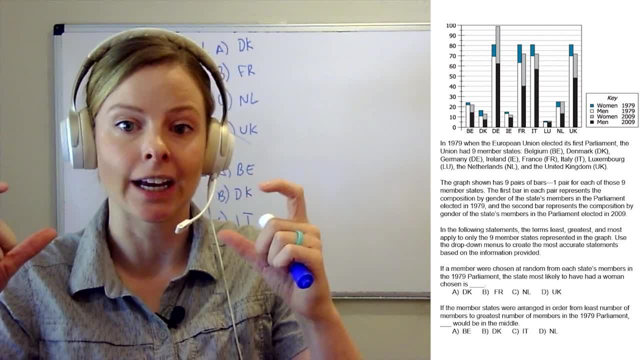 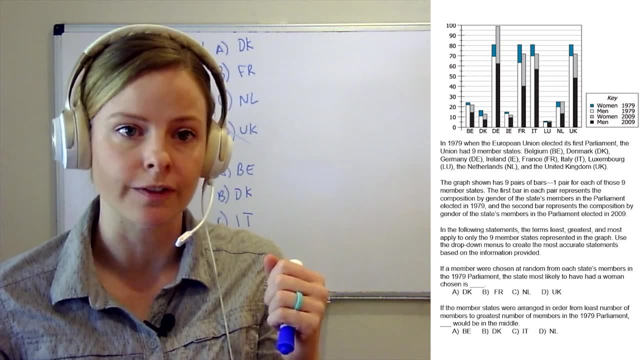 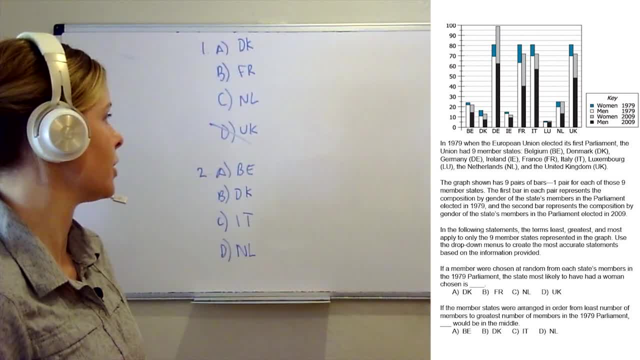 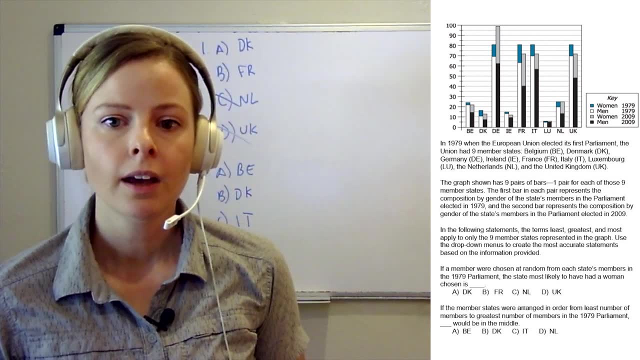 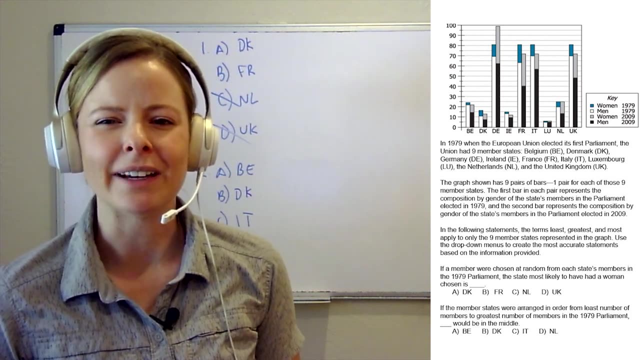 the nl pool. so again, don't have to do any math here. i can just visually see that i'm gonna have a higher proportion in dk than i would in nl. so from there you could do a visual comparison between our remaining options- dk and nl and f? r. but to be honest, i don't really feel comfortable with that. you know. i'm like, oh, if 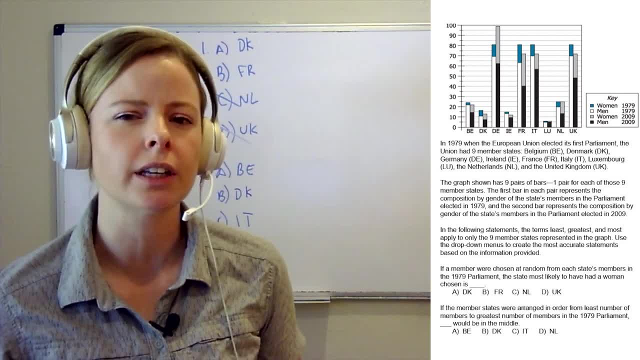 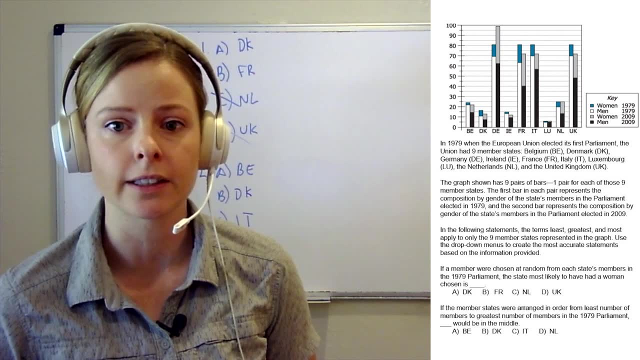 i scale that up, what would happen with my blue bar? to me it feels just a little too wishy-washy. so this is when i would go in and do the actual numbers, just to see if that really clarifies matters. so what i'm doing is i'm just going to see, like hey, what's my total population in the? 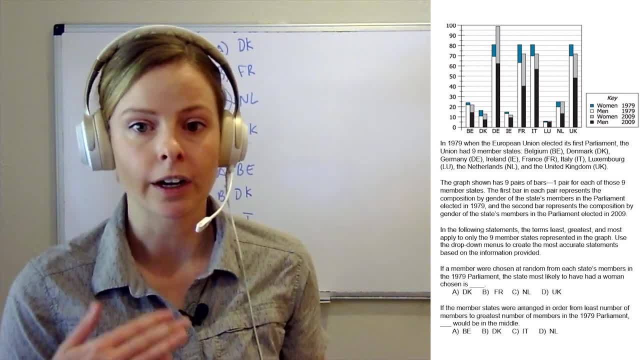 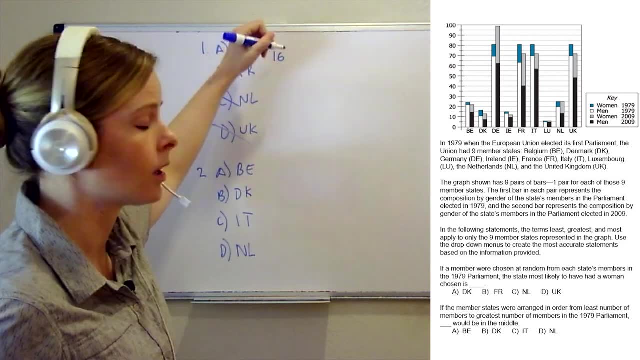 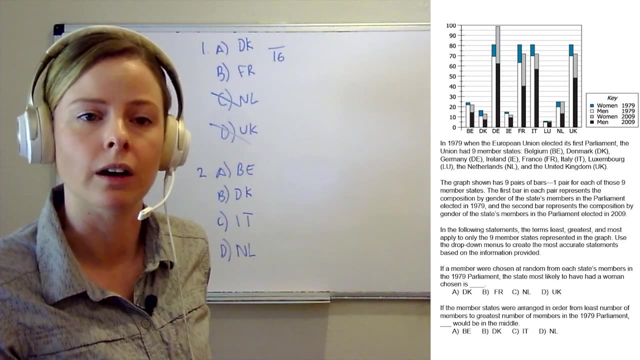 parliament, and then how many of those are women? starting with dk, our total population looks to be around 16.. and then our number of women, and again, it doesn't have to be totally, totally accurate here, because we're not given you know one by one on this scale, but to me it looks like six, um, so i'm guessing. 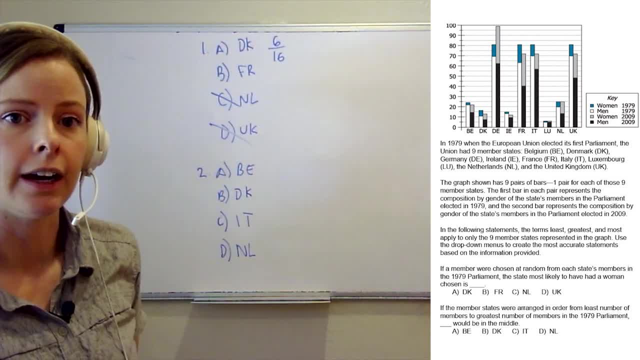 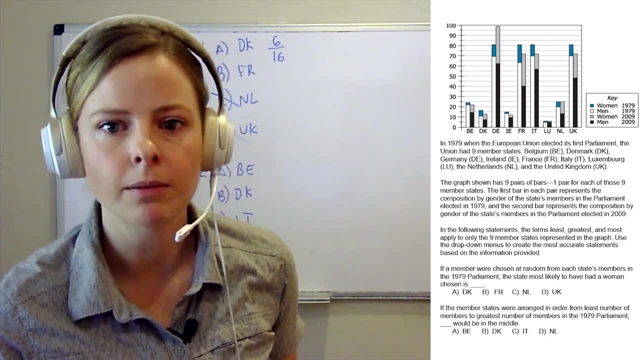 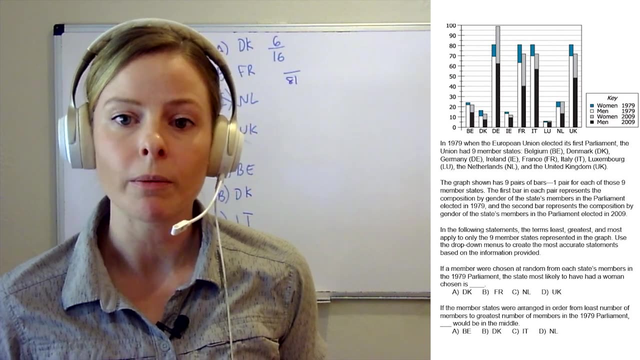 that, uh, we've got about six out of 16 uh women out of our total population. same deal for france. what's our total population? to me it looks like about 81, um, and then for the number of women within that population, you know the total population. 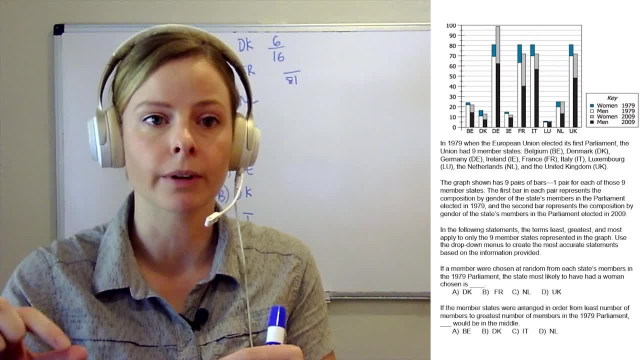 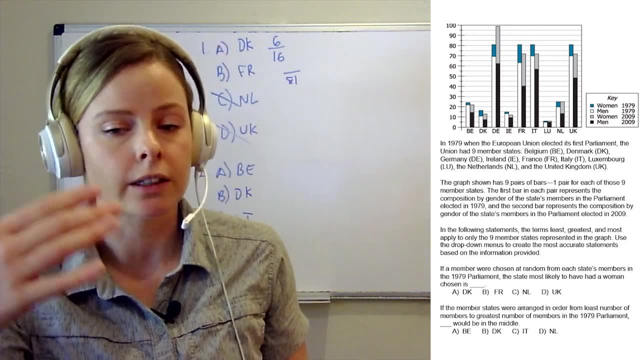 we span across three of our bars, right, so you know you, and each bar is five, so you know we've got at least 15.. um, to me it looks like we go a little bit below that and a little bit above that, so i'm going to go ahead and say that we've got around 18 out of 81 women out of our total. 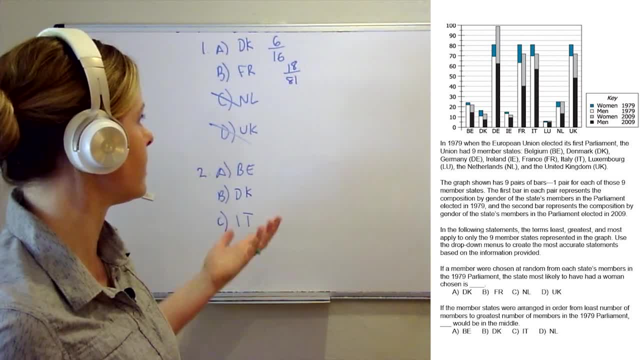 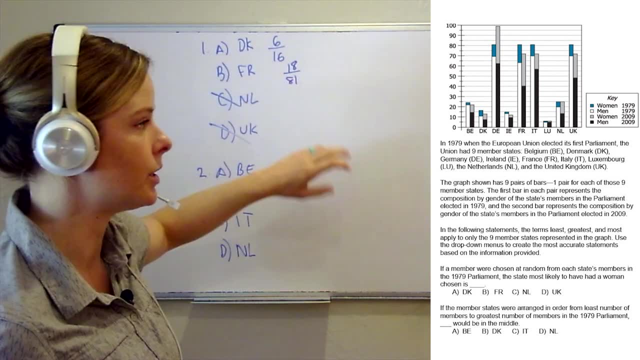 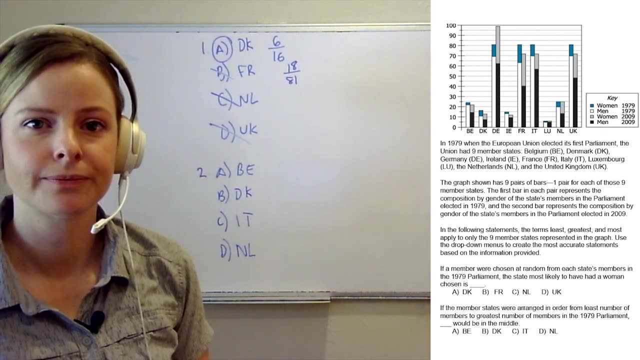 population for france. now, looking at these two and comparing them, this is a bit over one-third and then this is a bit under one-fourth. so very clearly, dk is going to be higher than fr and that is our winner for question one. moving on to question two, if the member states were arranged, 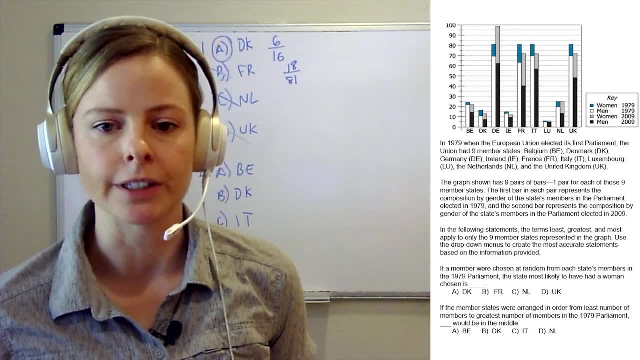 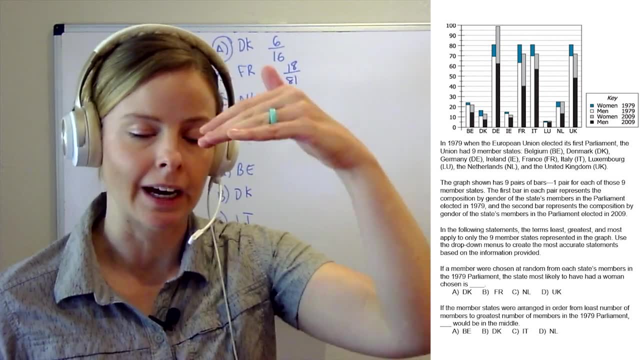 in order from the least number of members to the greatest number of members. in the 1979 parliament, blank would be in the middle. so we're just talking about the total number, so just the height of the bar. we don't really care about that split between men and women. 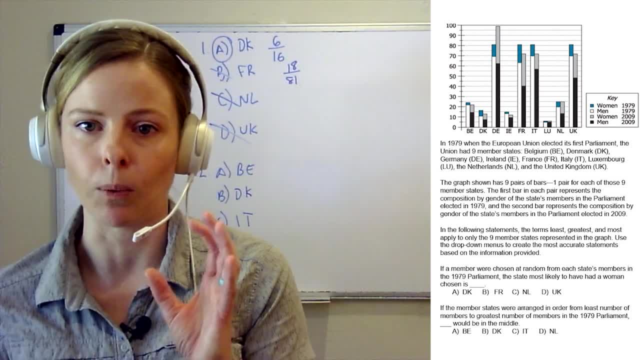 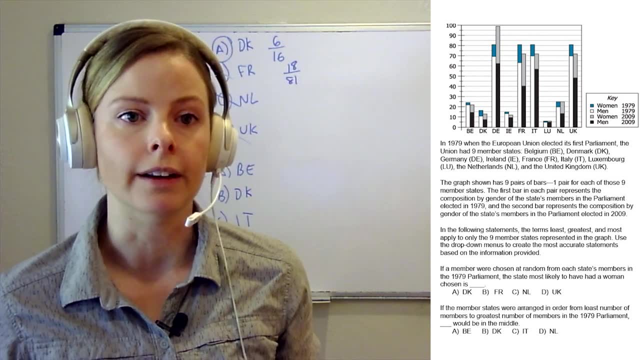 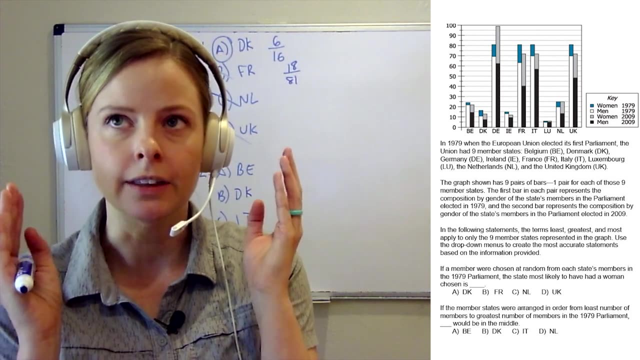 and again we are talking about 1979, so we are dealing with the white and blue bar, not with the black and gray bar. um, now, you could rank order all nine of these, but that again is kind of inefficient. don't really want to do that, um, so instead i'm going to think carefully about what the middle one means. we've 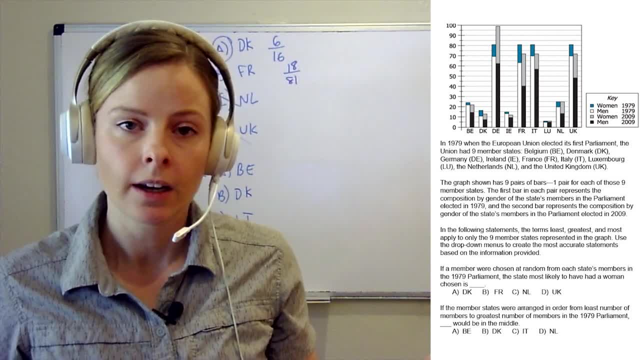 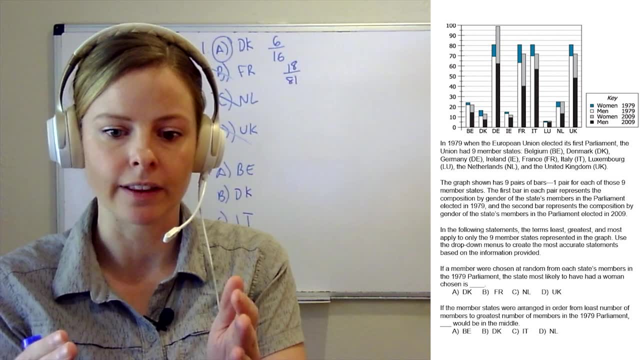 got a population of nine total states. uh, so which one is going to be smack dab in the middle? it's going to be the fifth one, right? so you'll have four smaller ones and then you'll hit the fifth one and then you'll have four larger ones. so number five is the one that's right in the middle. 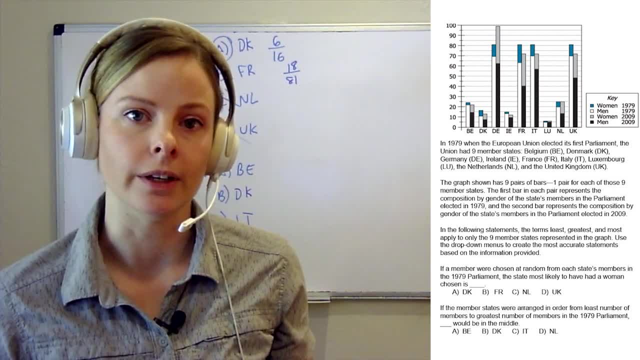 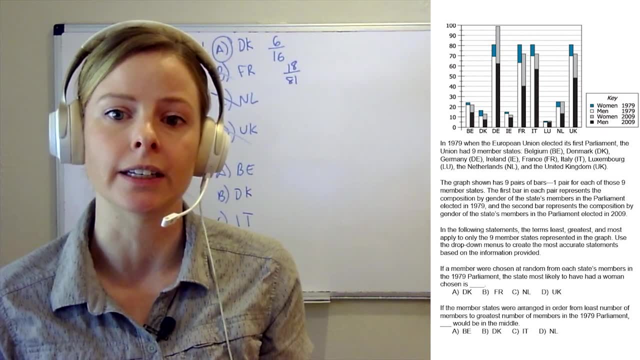 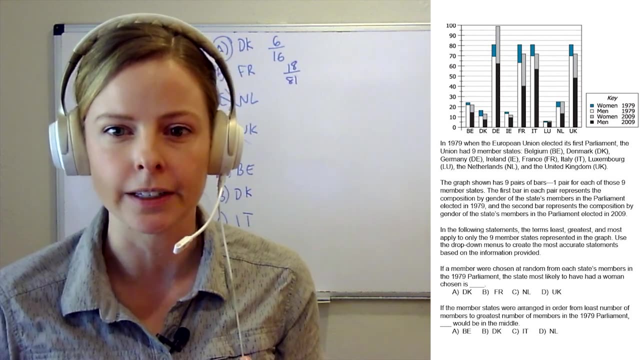 so i don't have to count all nine. all i have to do is determine, hey, which one has four below it or four above it. here i think it's easiest to see the four that are the highest right. so we can just like immediately get rid of, uh, those tall four, right? so we've got de, we've got fr, we've got it and we've got uk. 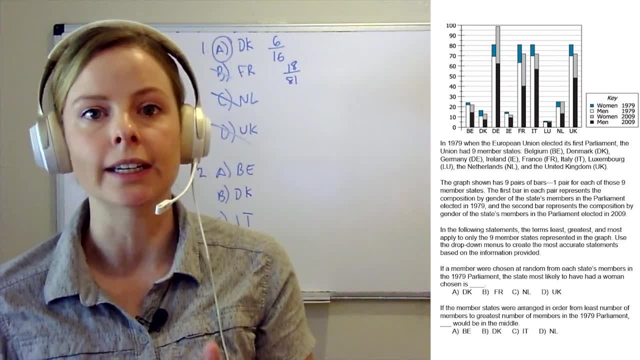 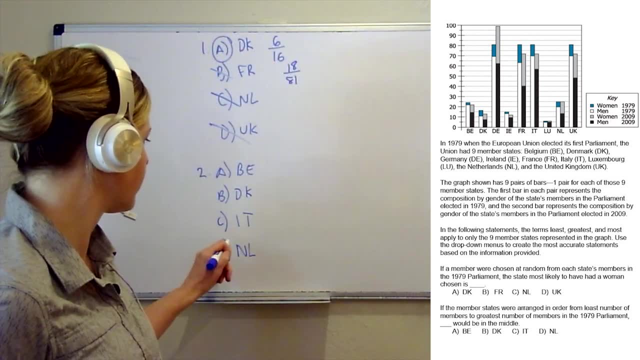 those are our top four, and then what we're looking for is: well, what's the next tallest one out of our remaining options? and you can see that the next tallest one is going to be nl. so that is our answer for question two. so that's the basics of a bar chart. again, you. 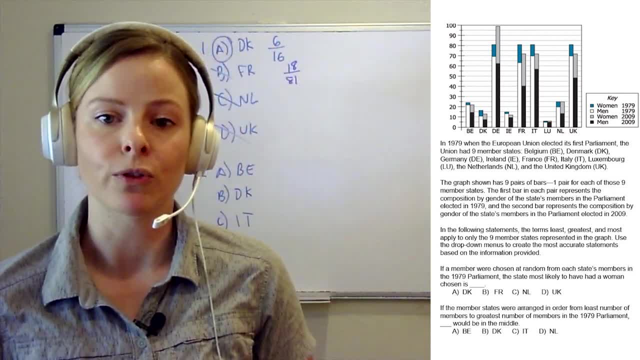 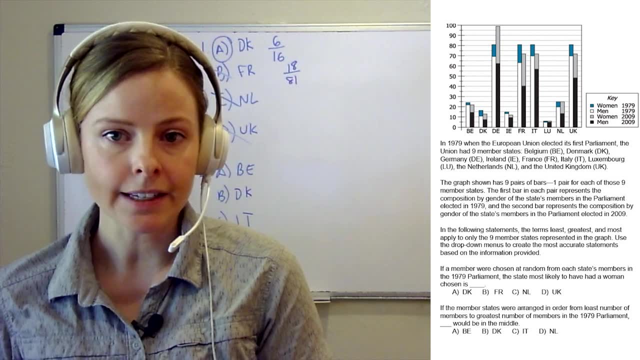 just want to give yourself time to really understand the data that's being presented before you dive in uh to the questions, and then just be careful as you go through the questions themselves. next up, we will go through a pie chart and it is the same exact punchline. so we're gonna 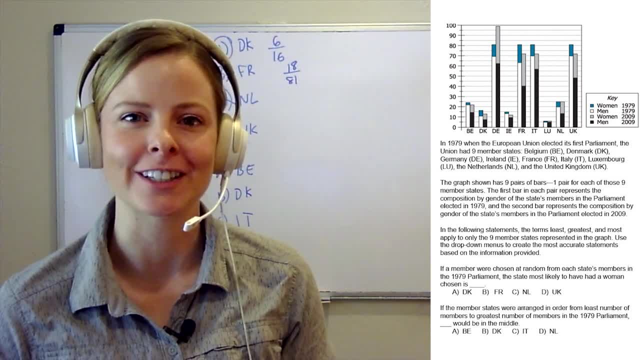 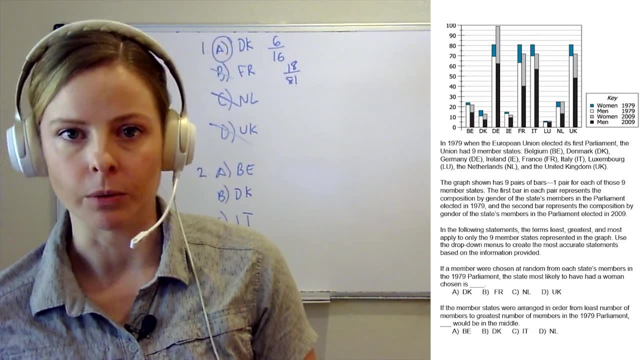 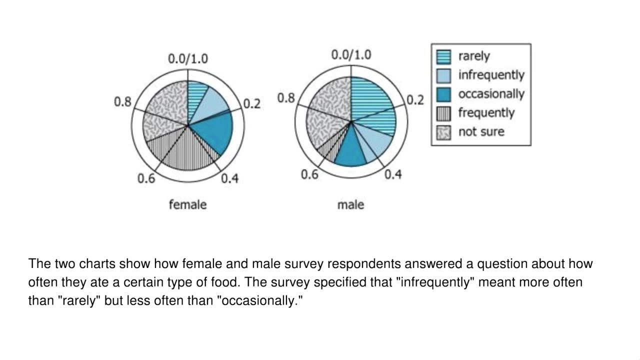 go ahead and give you maybe a bit longer here, maybe 20, 30 seconds, to just look at the chart itself given to you, And then we will go through the chart and then add some questions in as well. All right, so let's talk about these pie charts. We're given two different pie charts. They're 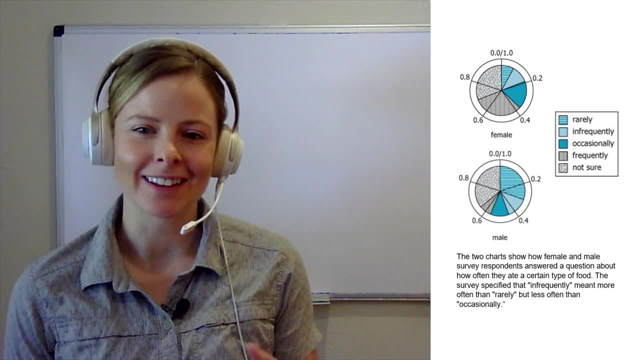 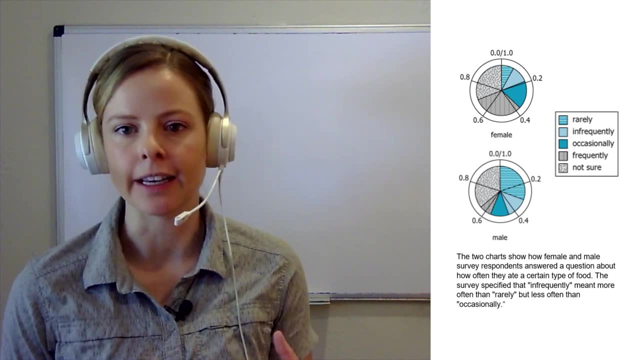 called pie charts because they look like slices of pie, And the nice thing about pie charts is that they're going to add up to 100% of your population in some way, So you can just look at this and get a sense for what piece of the pie falls into each category. So for this particular 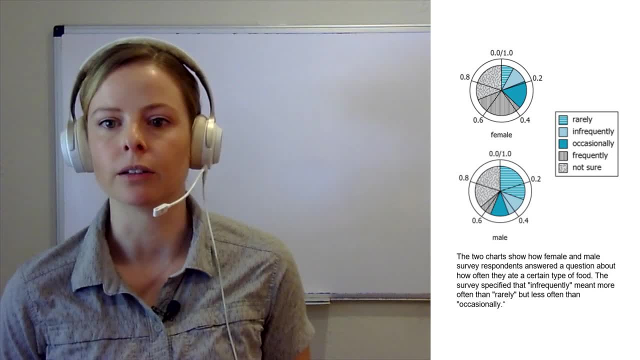 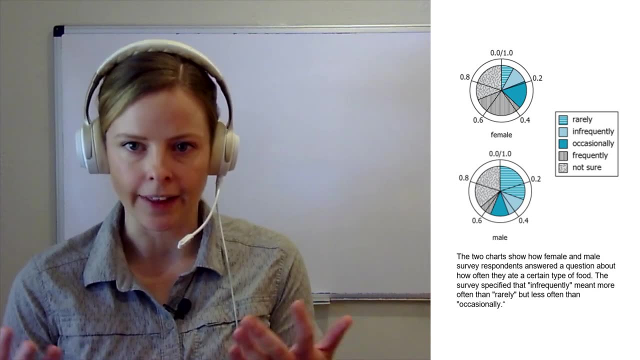 one. we're told that the two charts show how female and male survey respondents answered a question about how often they eat a certain food, And then we're told that the two charts show how certain type of food. So just taking that and looking above, one thing that pops out to me is 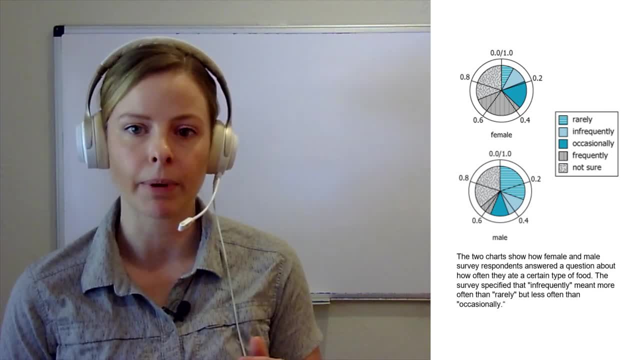 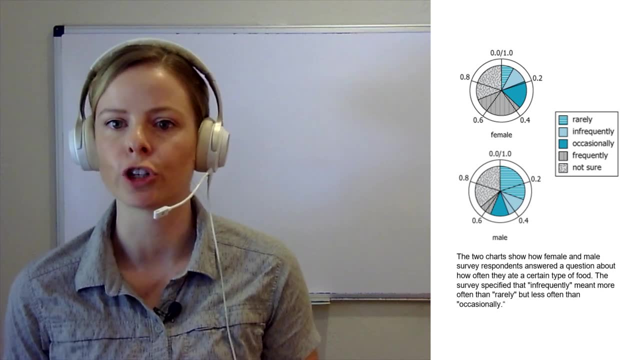 that we don't have any hard numbers at all. Our pie chart just adds up to 1.0.. So what we're given here is more about percent or about proportion than it is about actual numbers. right, We don't know how many people they surveyed. They could have surveyed, you know, a thousand men and women. 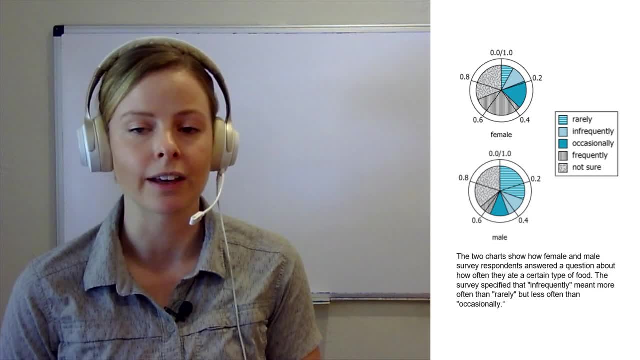 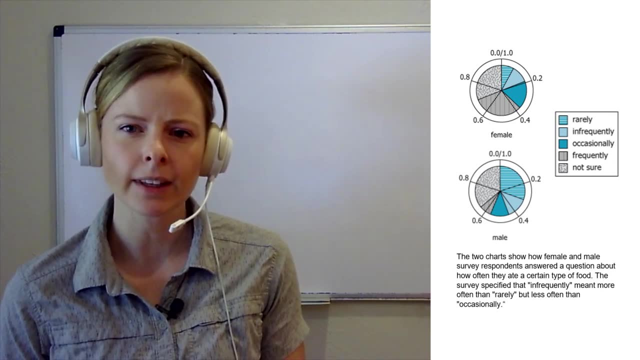 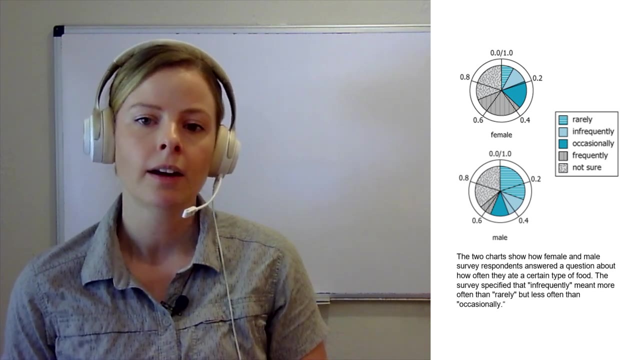 They could have surveyed a million, right. That kind of thing. We have no idea how many people actually fall, We just know what chunk of the pie they take up. The other thing that pops out to me is that they've marked this: 0.2, 0.4, 0.6, 0.8 around the pie, which just gives you a really nice visual cue for 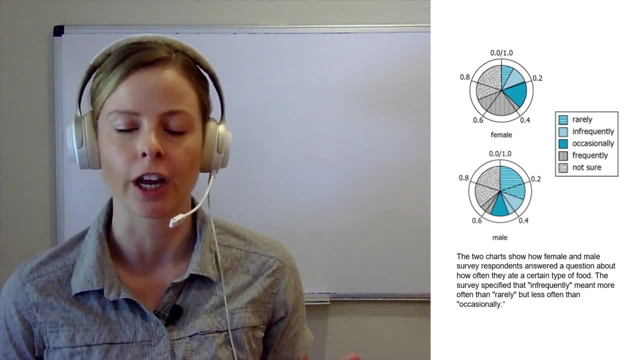 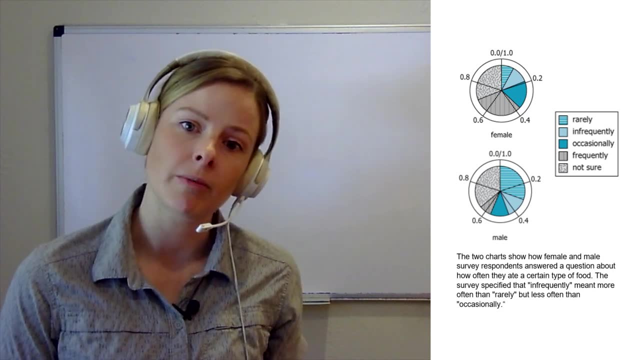 kind of you know what percent falls in each area. It would just be a little bit trickier to see that without those additional guiding points. So for instance, on the female pie chart we see that 0.8 cuts right through the middle of the not sure. So that's a little bit tricky to see. But 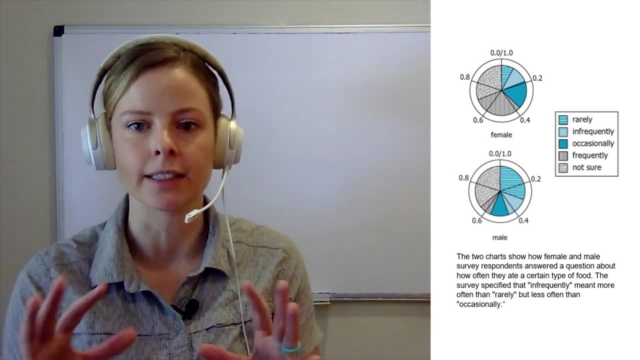 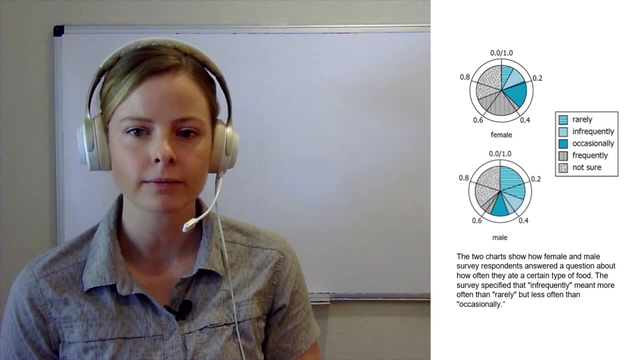 that's a little bit tricky to see. So that's not an actual line that cuts the data in half. It just tells you that, hey, the 80% mark falls, you know, kind of in the middle of that chunk. The next: 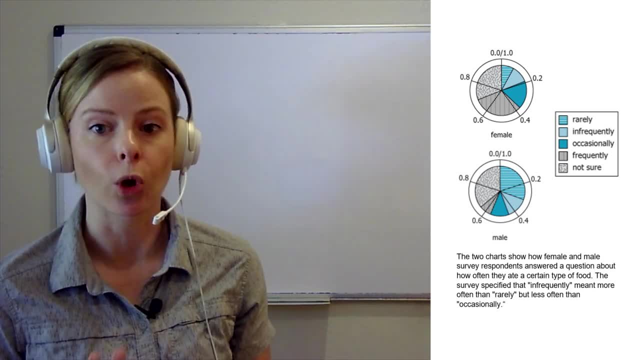 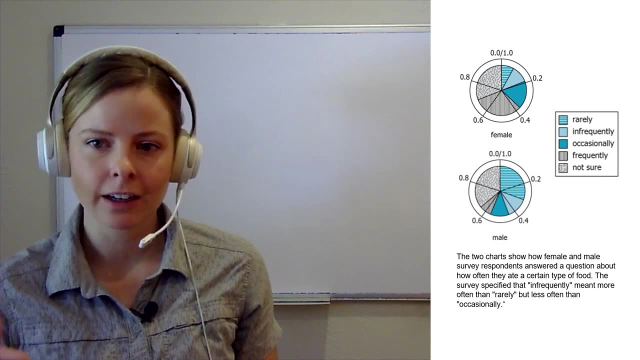 little detail that we get in the description is that infrequently meant more often than rarely, but less often than occasionally. That's kind of a mouthful, to be honest. But here I'm just looking at the key and I'm seeing that it's written in a way that makes sense. So it is going. 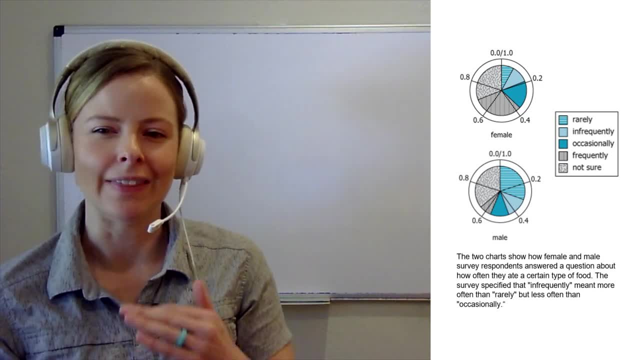 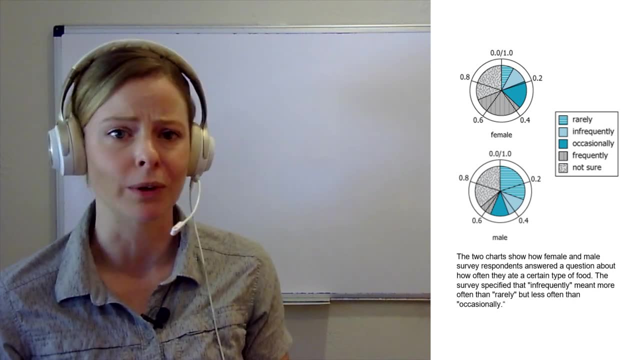 off into I eat it the most frequently. And then it's just that those particular words, you know, are a little confusing, right? Just without that additional context. what does rarely mean versus infrequently? Well, this just tells us that, hey, it's in order. So that's good to know, That's nice. 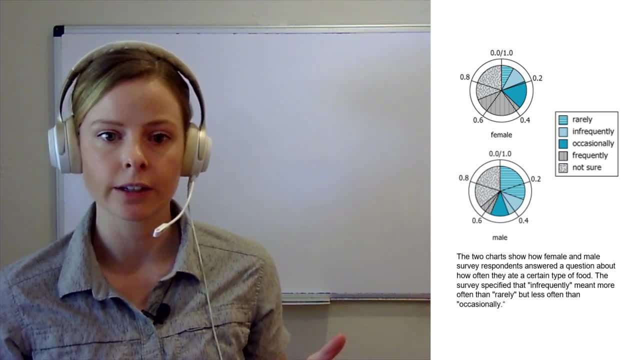 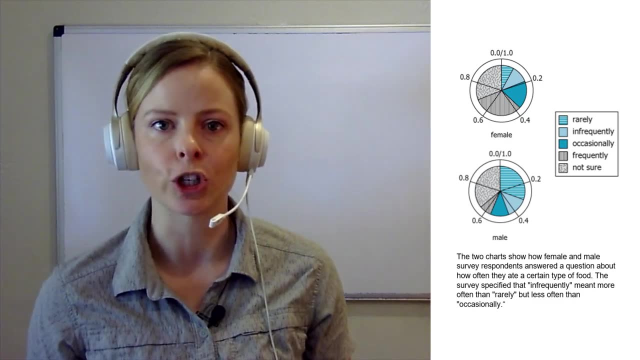 So that's really what there is to get out of these pie charts. We'll go ahead and throw a question up on the board- It's just one question for this one- And take your time, answer it, and then we will chat it through. So that's really what there is to get out of these pie charts. So that's really. 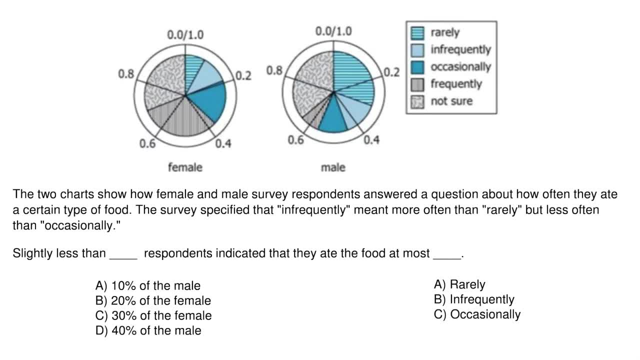 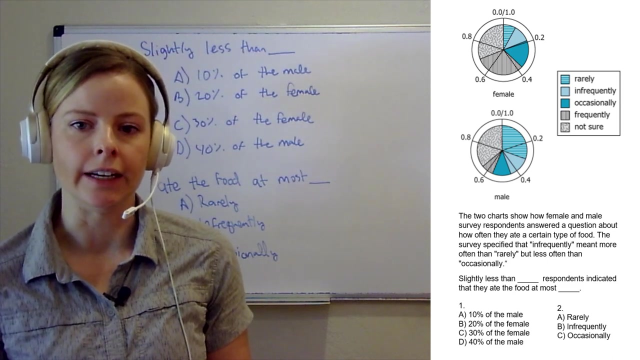 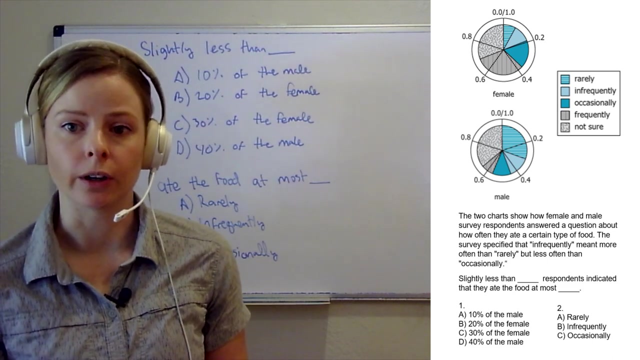 good to know, Thank you. Thank you, All right, let's go through this. So the question asks slightly less than what percent of certain respondents indicated that they ate the food at most rarely, infrequently or occasionally. So what we have here are two blanks in one sentence. Those two blanks depend on one another, So I can't. 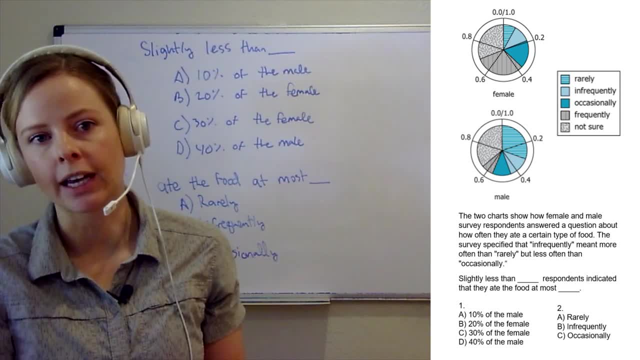 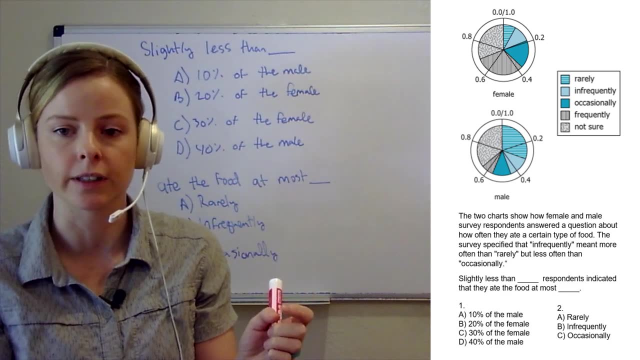 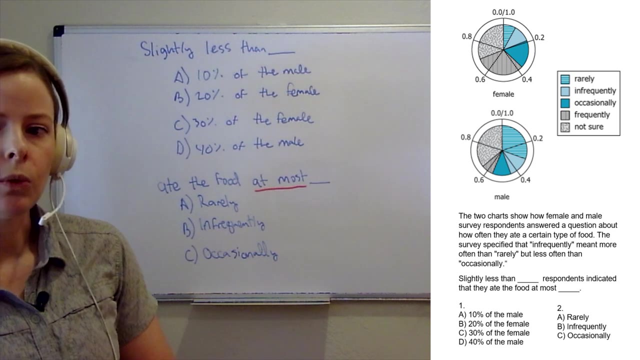 independently choose an answer for the first blank and then independently for the second blank. it really depends: what goes in that first one will change what goes in the second one. To me, what stands out here language-wise are these words: at most. So what does it mean to say at most rarely? Well, that would be just 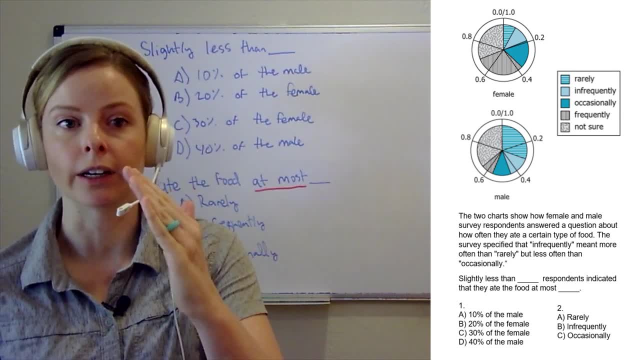 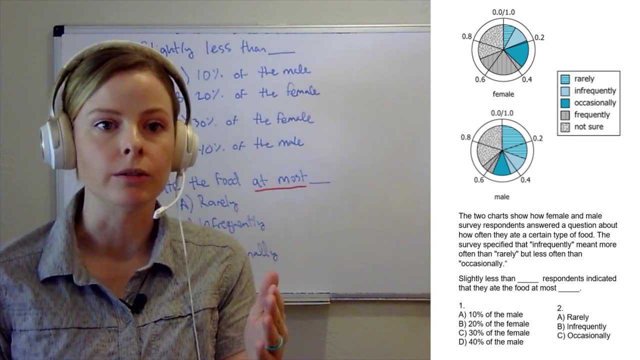 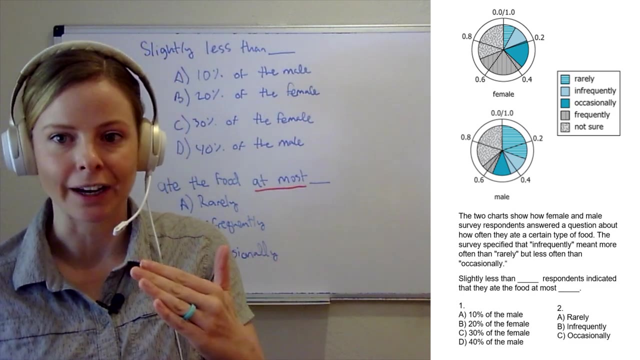 starting from zero and then going to wherever rarely ends right Versus what does at most infrequently mean. Well, that includes that earlier portion. rarely Right, Because both my rarely people and my infrequently people fall into that bucket of at most infrequently. So I'm 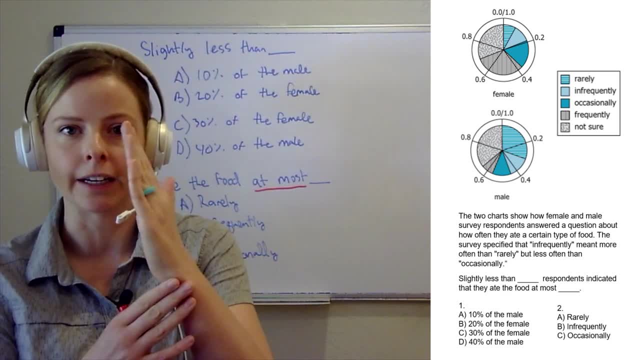 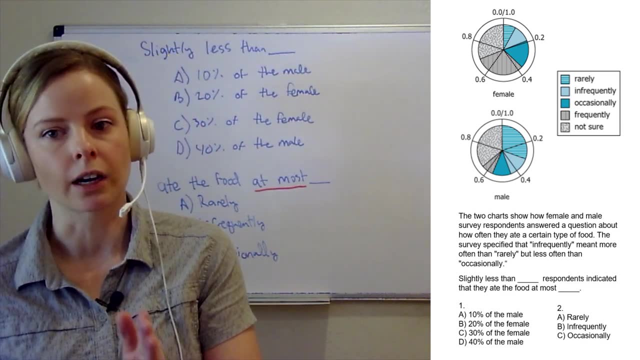 always going to be starting at the top of the pie chart and then kind of seeing like, where does this end up, And then is there an option that works for that. So here I do think it's easiest to start with the second blank and then look at my. 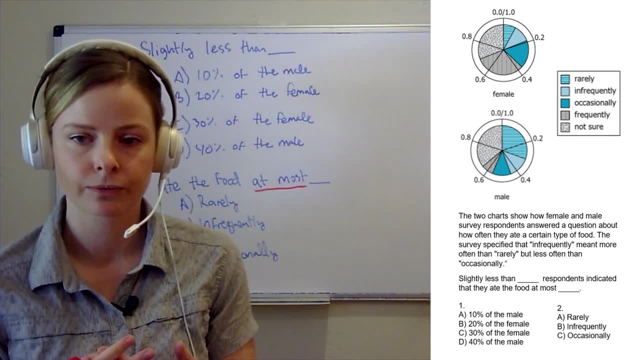 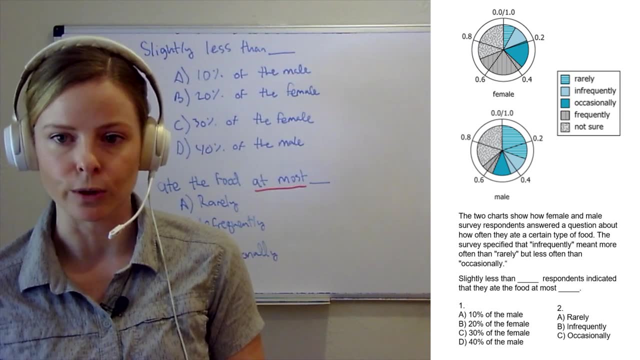 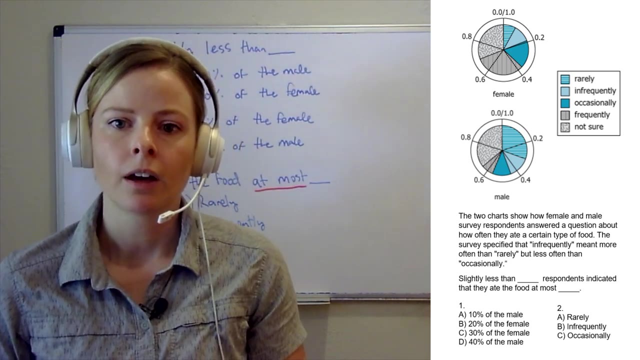 options for the first blank to see if there is a pair that actually makes sense. So let's do that and we'll just start with rarely So slightly less than some percent of respondents indicated that they ate the food at most rarely So for our women. if you look at that chart, we get what eight percent maybe said that they ate rarely. 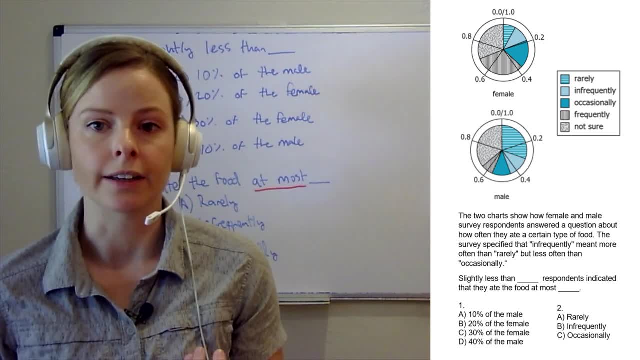 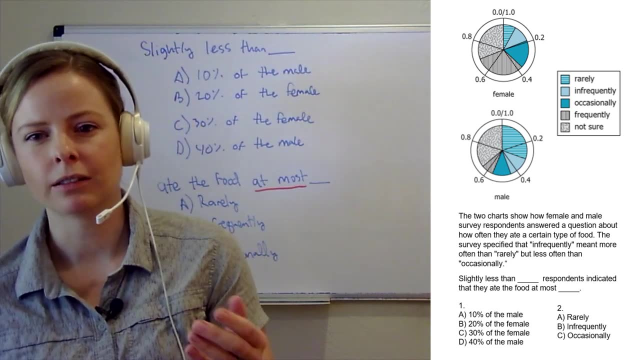 And then for our men, we see that we've got about 30% saying that they ate at most rarely. So a 10% of the male eating at most rarely- Nope, Way more than that Eagle. so that doesn't work. 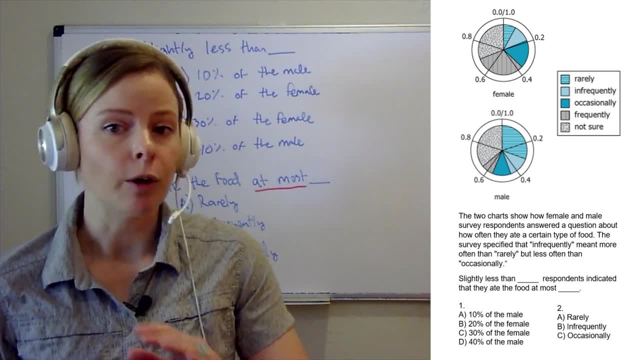 20 percent of the female- Nope Way less than that. Eagle two percent ate at this class added, which isn't behatoscopic, all that food says, and they decided that they ate at most rarely. Oh, that's crazy. And she said to us I was saying they ate at most rarely because they made a really good job. 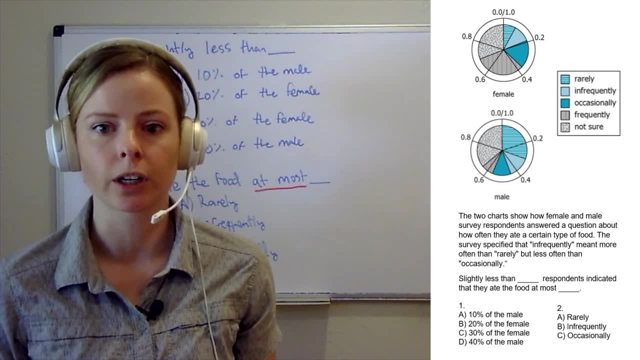 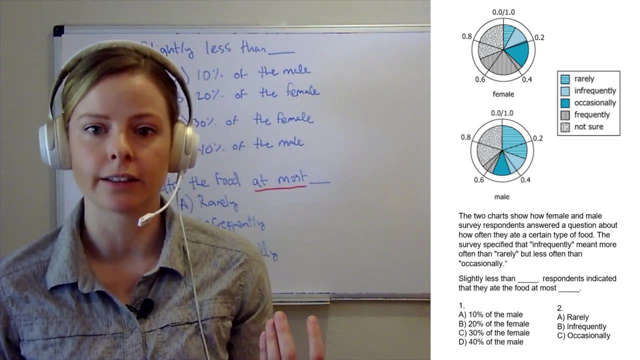 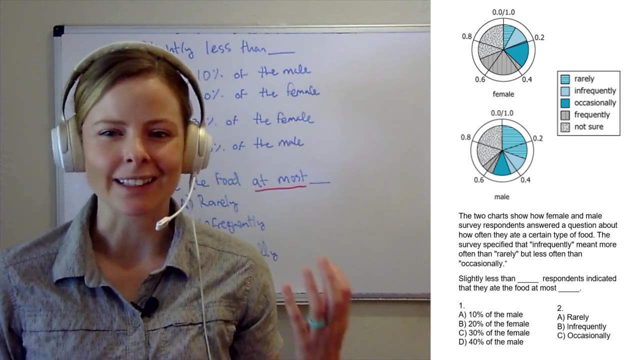 So that's the best answer here and I feel good about utilizing your maybe. maybe people getting the up ate rarely, so B doesn't work. For C, we've got 30% of the female- Again way less, so same reasoning as the previous one can get rid of it. And for D, 40% of the male. So it says slightly. 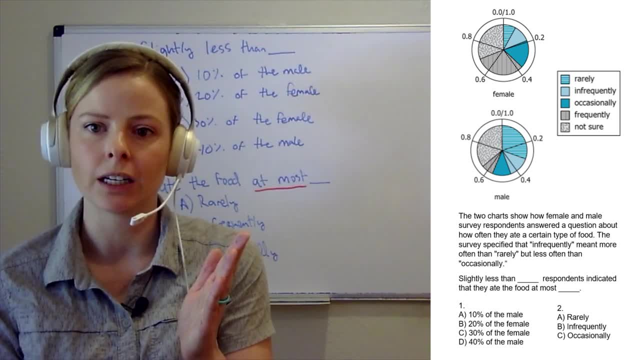 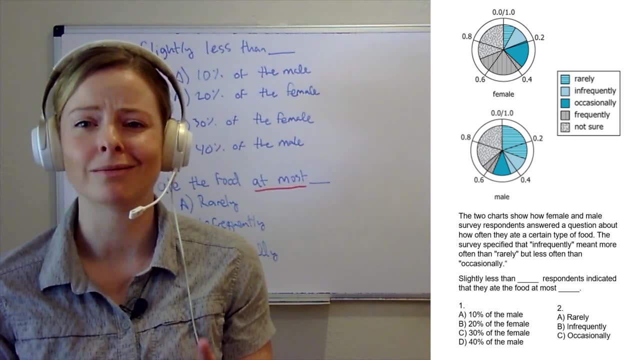 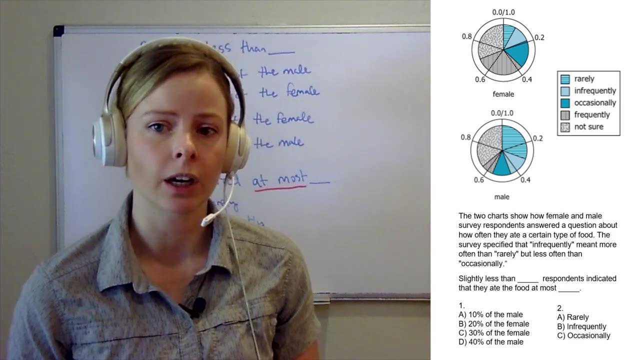 less than, and again we've got about 30% of our men eating the food at most rarely. That's a pretty significant chunk below. So maybe if there's no better options, I would keep it, but for right now I'm going to say that's pretty far off. So I would go ahead and get rid of rarely, because 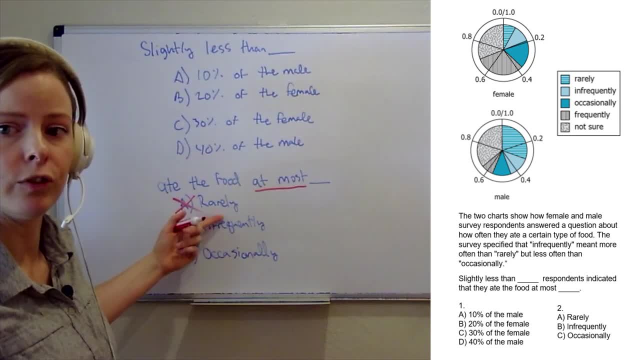 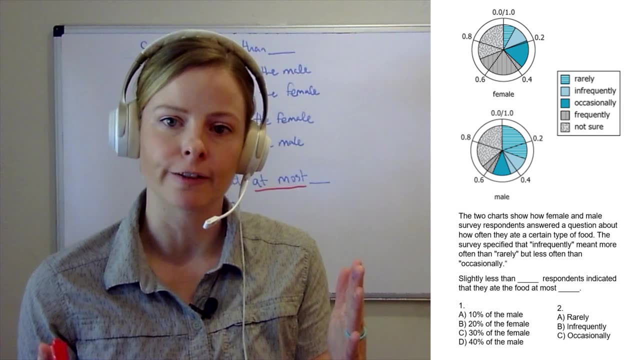 there's really no option that fits well for that being our second blank. Let's do the same thing for infrequently So eating at most infrequently. if you look at the female chart, we've got about 19%. If we look at the male chart, we've got about 19%. If we look at the female chart, we've got. 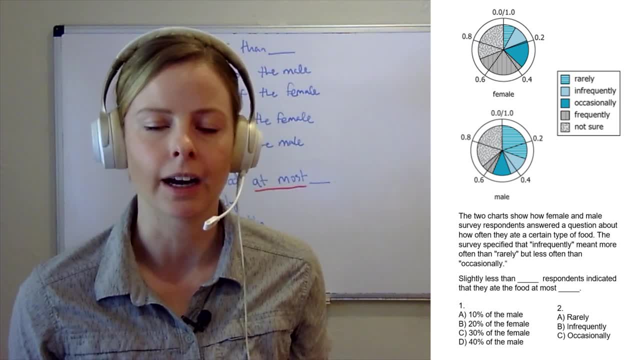 19%. If we look at the male chart, we've got about 19%. If we look at the female chart, we've got about maybe 45% that are eating at most infrequently. So slightly less than 10% of the male for. 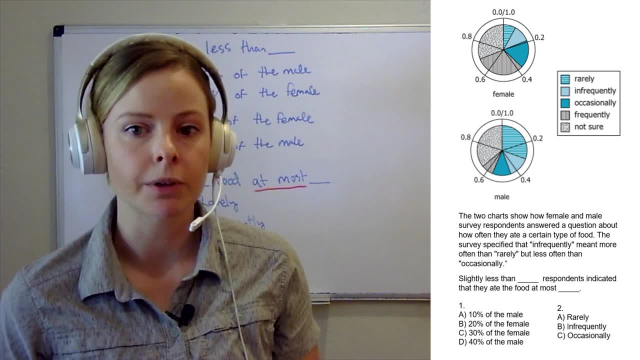 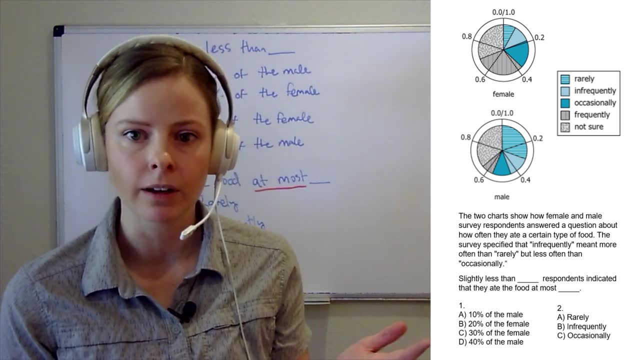 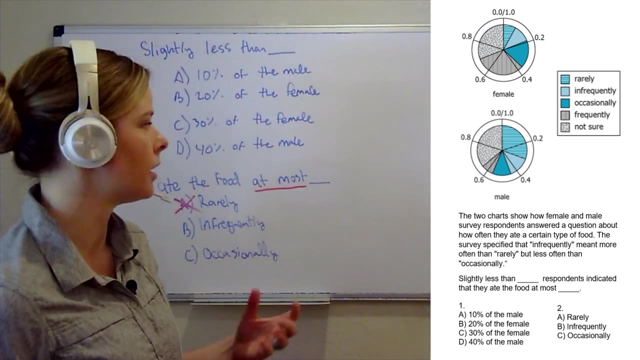 infrequently no way more than that- Slightly less than 20% of the female. there we go. We said that about 19-ish percent of our female respondents ate that amount and that corresponds really nicely with slightly less than 20%. So the pair here that works is slightly less than 20%. 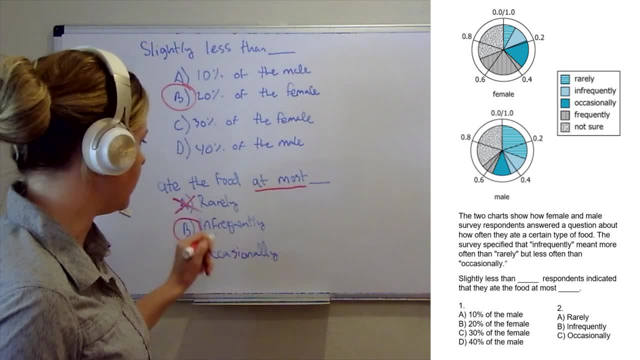 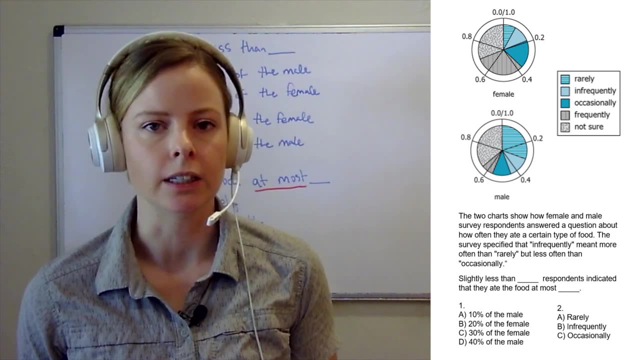 and that corresponds really nicely with slightly less than 20% of the female respondents ate at most infrequently. So that's a pie chart Here. we've got some small quirks that you might not see in other pie charts, but that's the name of the game on the GMAT. There's always some slight twist. 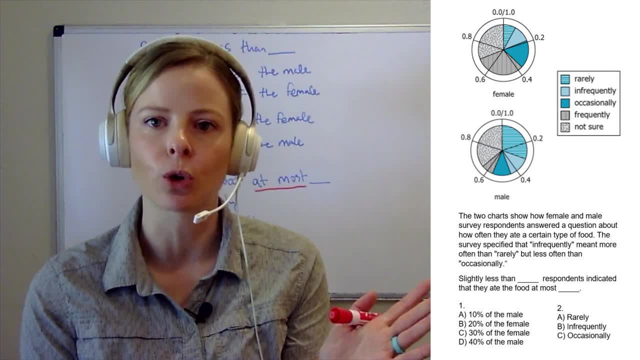 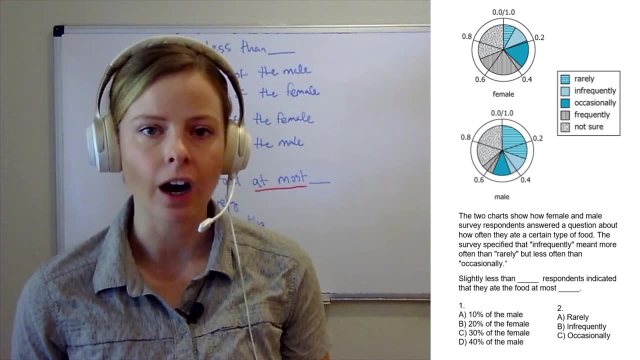 But at the end of the day, what a pie chart is is just showing you what wedge corresponds to what thing in your key. So we will go ahead and do one more kind of common chart type. It's going to be a flow chart. This is going to be a flow chart. It's going to be a flow chart. It's going to be a flow. 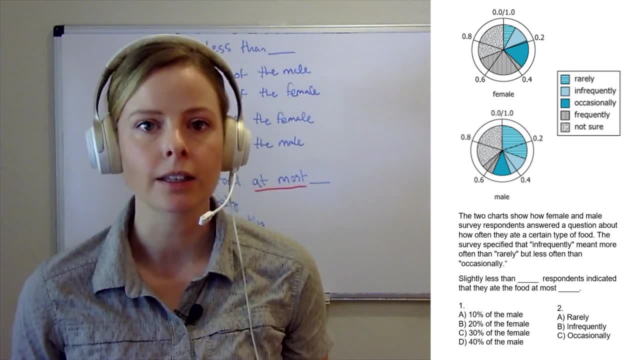 chart. This one is a little bit more convoluted, so we'll give you a bit more time, maybe 30 seconds, to go ahead and kind of see what's going on with the flow chart. Then we'll talk about it. 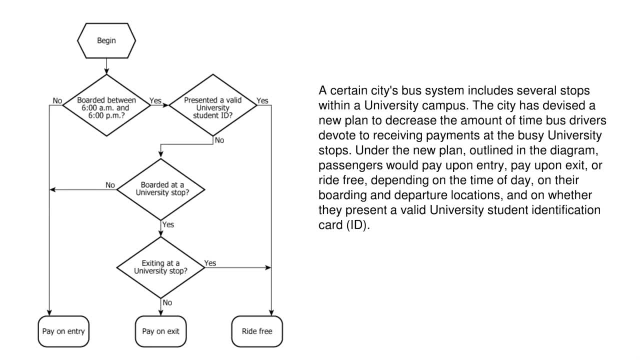 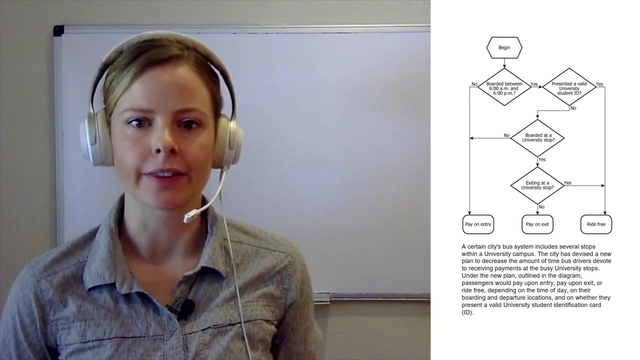 and finally, we will finish up with some questions. All right, let's talk about this flow chart. So first thing I'm doing is just taking a glance at the chart itself. It looks like we've got a begin, so something is starting, and then we've got a whole 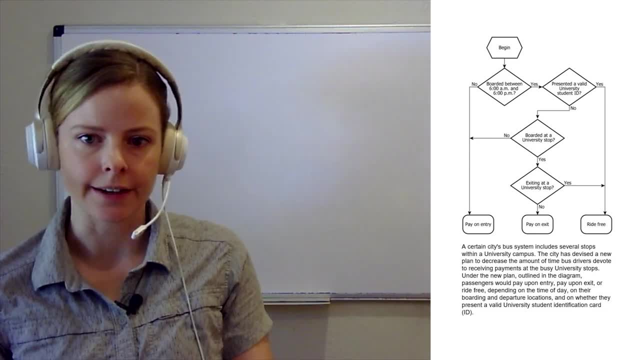 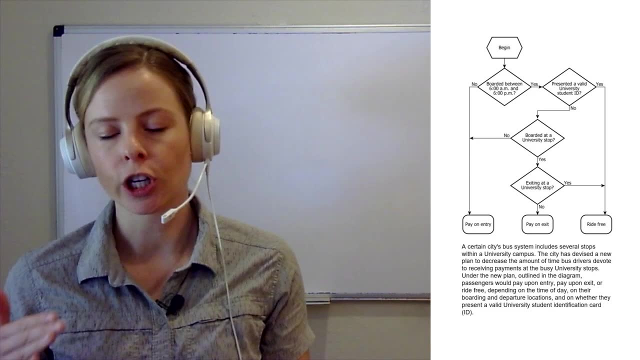 bunch of different options that happen And then at the end of the day you can end up in one of three buckets. You either pay on entry, or you either pay on entry, or you either pay on entry, pay on exit or ride free. So that's intriguing. Let's go look at the description to see what. 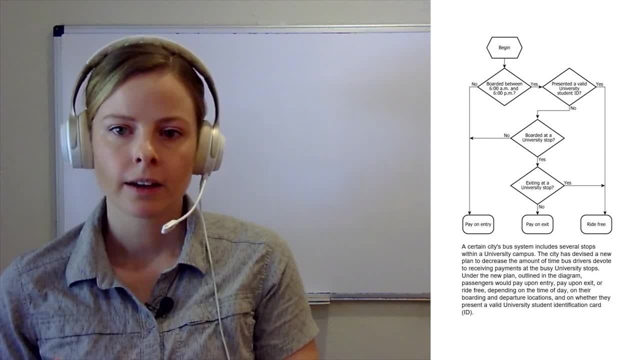 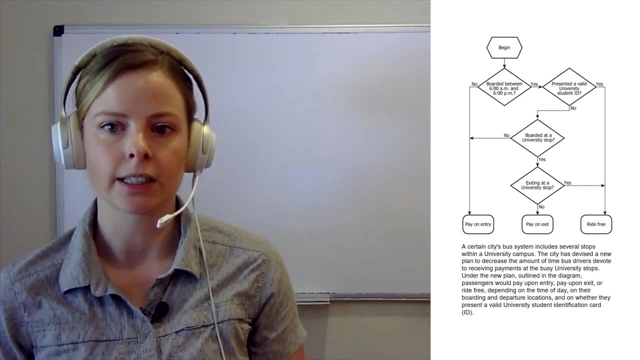 exactly we are paying for or riding free on. The description says a certain city's bus system includes several stops within a university campus. The city has advised a new plan to decrease the amount of time bus drivers devote to receiving payments at the busy university stops Under the. 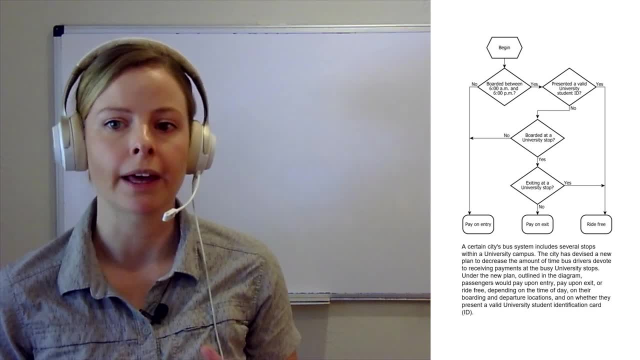 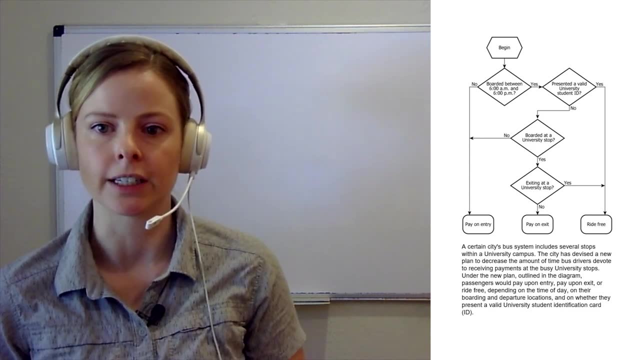 new plan outlined in the diagram, passengers would pay on entry, pay on exit or ride free, depending on the time available, And then, at the end of the day, on their boarding and departure locations and on whether they present a valid university student identification card. So what I'm getting out of this is just kind. 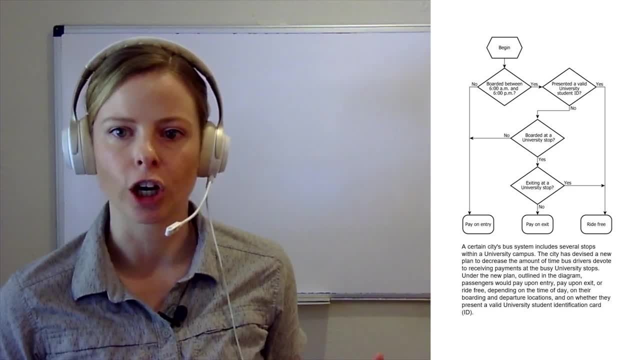 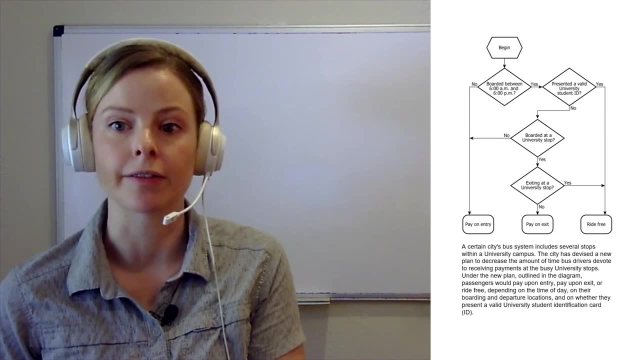 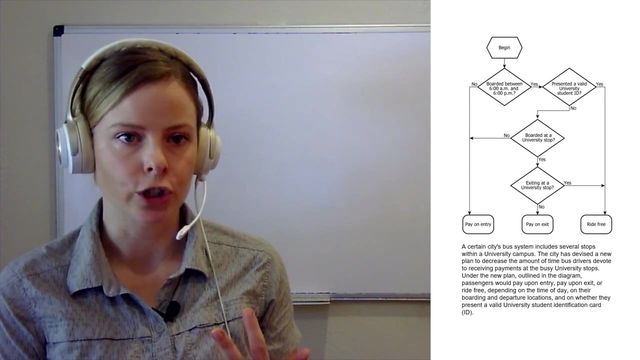 of a nice rundown of what all is located in that chart, And particularly I'm interested in these criteria that decide which bucket you end in at the end of the day. So it looks like the criteria are the time of day that you enter the bus, their boarding and departure locations, and then whether 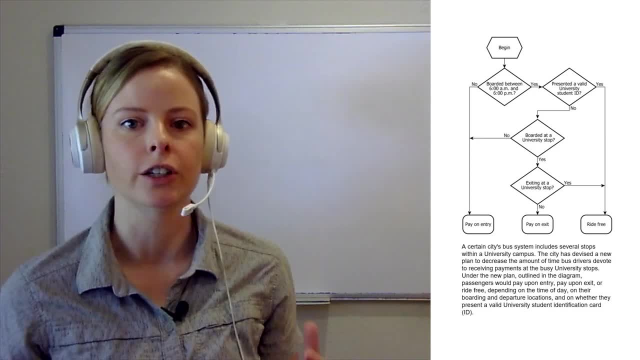 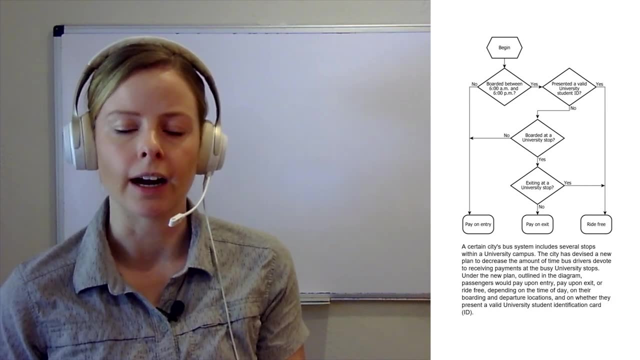 they're going to be able to get to the bus at the end of the day. So what I'm getting out of this is where you present a student ID card right. So, based on those three factors, you will end up in one of these three outcomes. I think that's a good place to leave it for now, And then we'll go ahead. 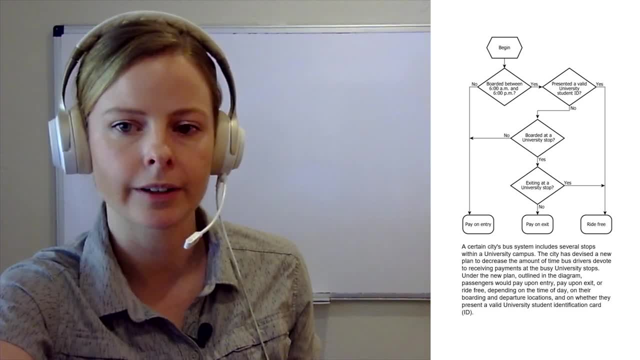 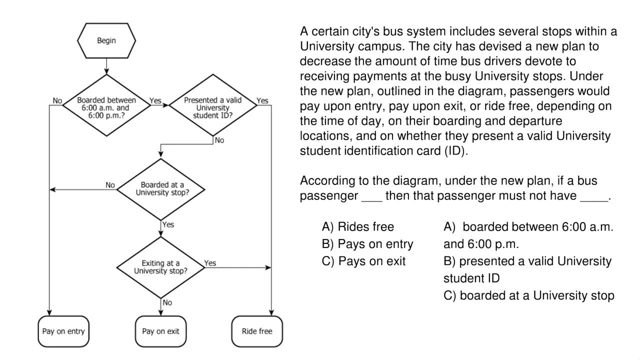 and look at the question and see what we can get out of it. Again, I'll throw it up on the screen for a couple minutes, take your time and then we'll go through it. Okay, so we'll go ahead and look at the question and see what we can get out of it Again. I'll throw it up on the screen for a couple minutes, take your time and then we'll go ahead and look at the question and see what we can get out of it. 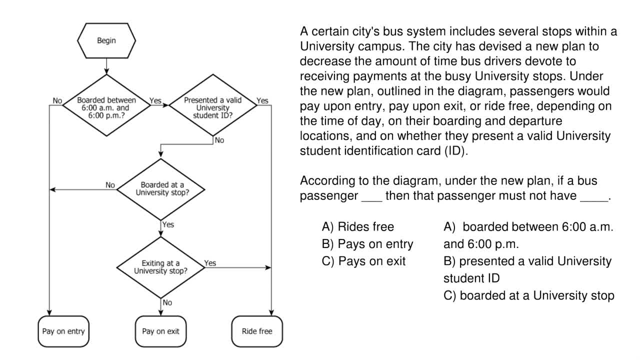 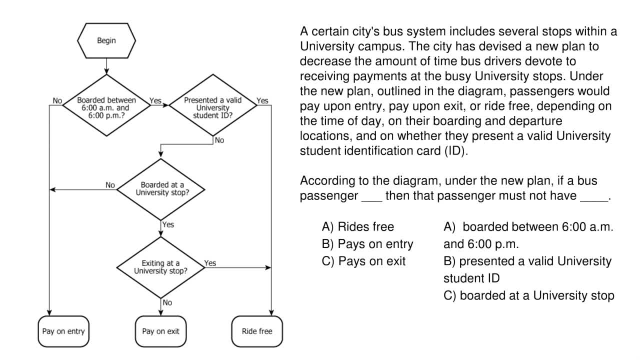 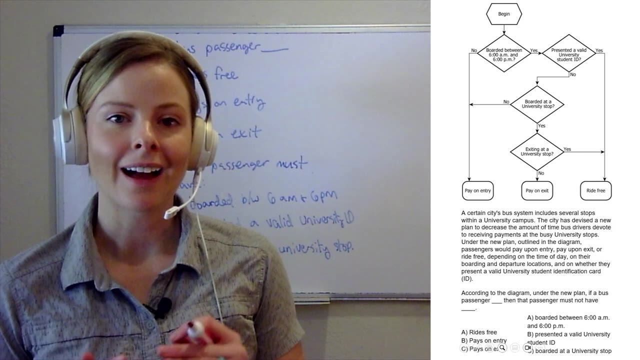 Again. I'll throw it up on the screen for a couple minutes. take your time, and then we'll go ahead and look at the question and see what we can get out of it. All right, let's go ahead and talk through this question. 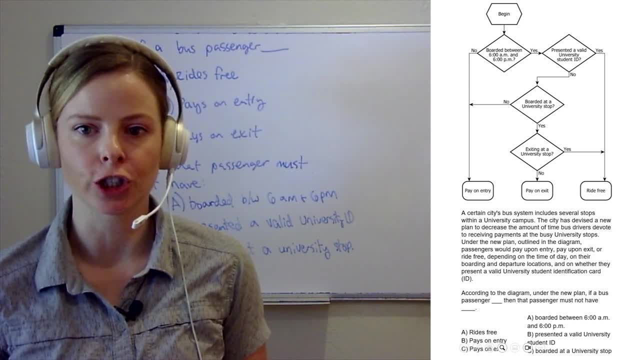 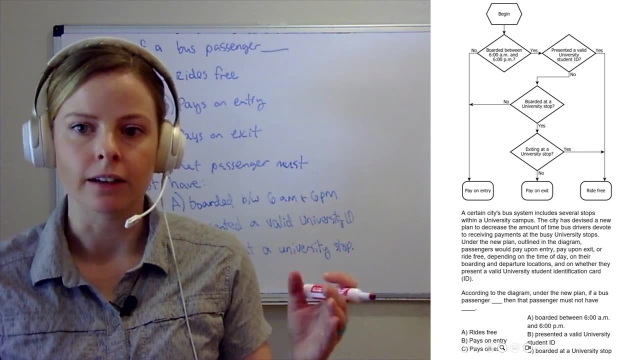 We have. according to the diagram under the new plan, if a bus passenger does something, then that passenger must not have done something else. So these blanks again are dependent on one another. We can't just look at them in isolation and decide on the first one and then on the second. 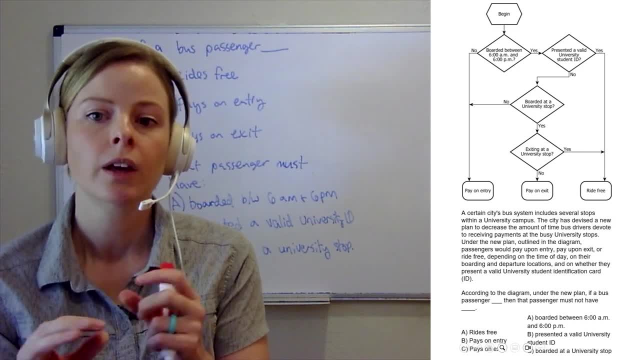 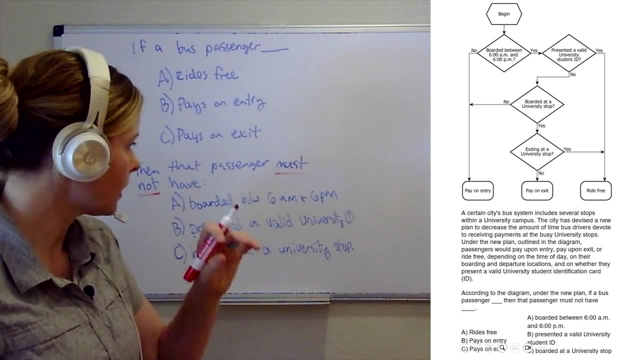 one, We have to look at both and see if there's a pair that works for both. The other thing that really stands out to me here is this word must and this word not. So must not means it just can't happen, right. 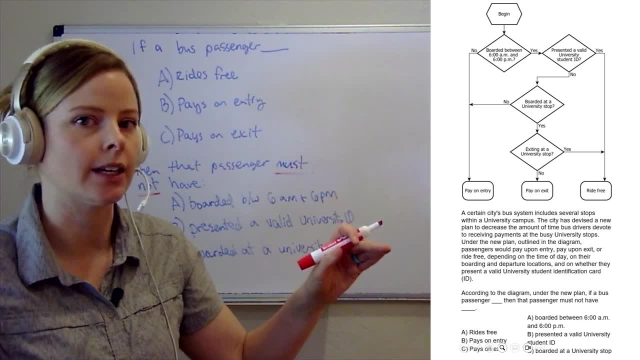 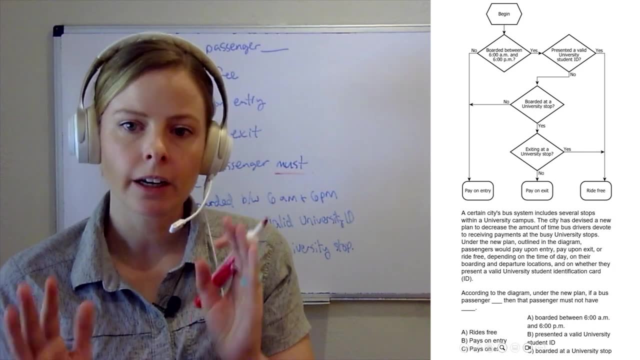 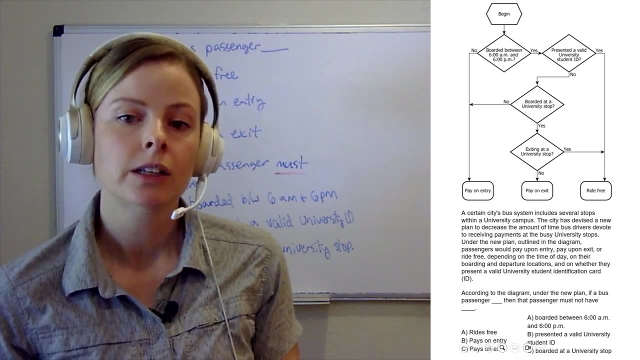 So if this first thing did happen, then the second thing just can't have happened. That's what we're looking for to correctly answer this question. So here I think it's easiest to start with the first blank, because we have these buckets that you end up in at the end of the day. 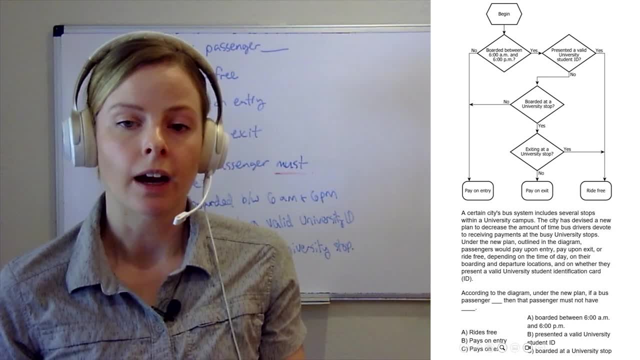 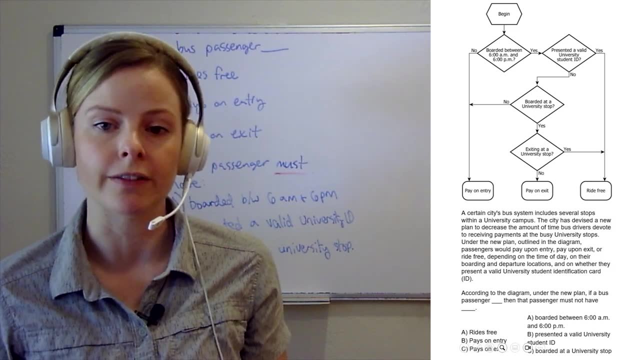 So what we can do is: we'll start with A rides free and just see- well, how could you end up riding free? And then is it true that you must not do one of these things to end up, in fact, riding? 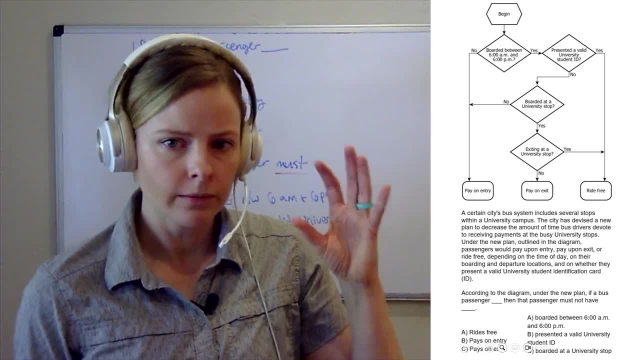 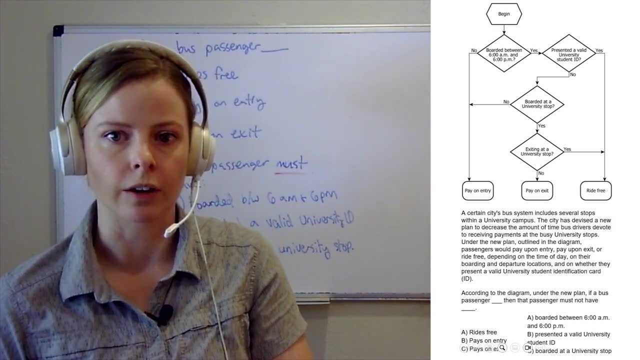 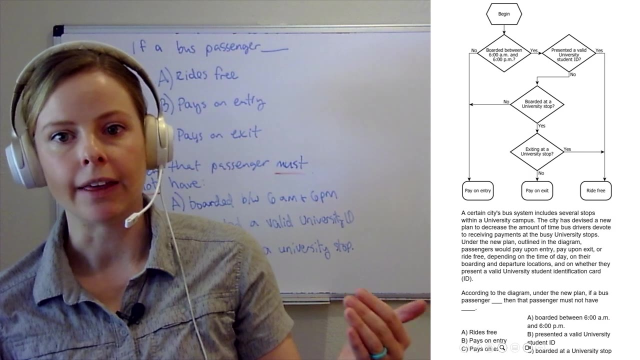 free. So let's do that To end up in that bucket of riding free. to me I see two pathways. The first pathway is pretty simple. It goes along the top and the side. So if you board during the day, so between 6 am and 6 pm, and then you present your, 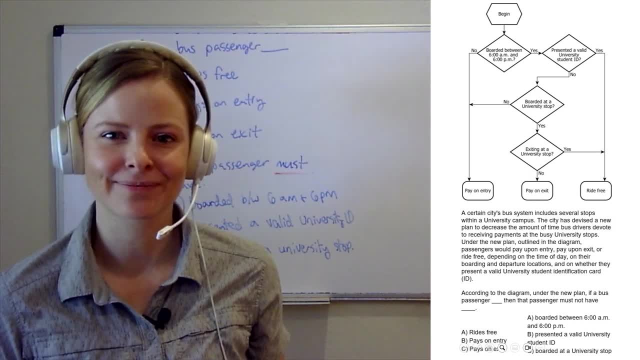 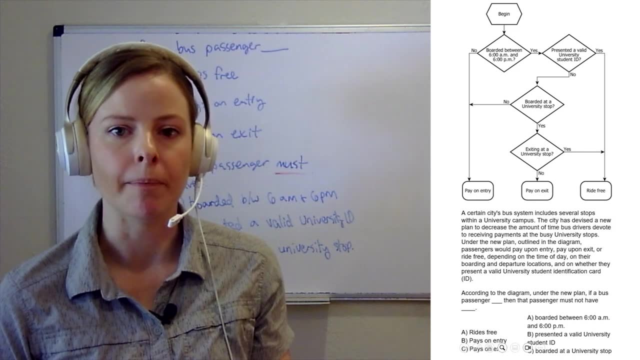 student ID. guess what You get? to ride for free. That's very nice. The other thing that ends up in the rides free bucket is if you board between 6 am and 6 pm but you don't present to students. 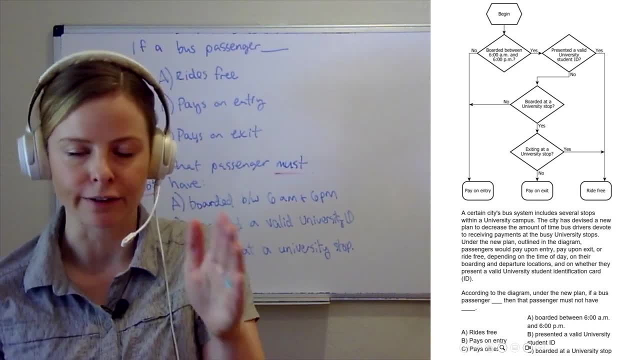 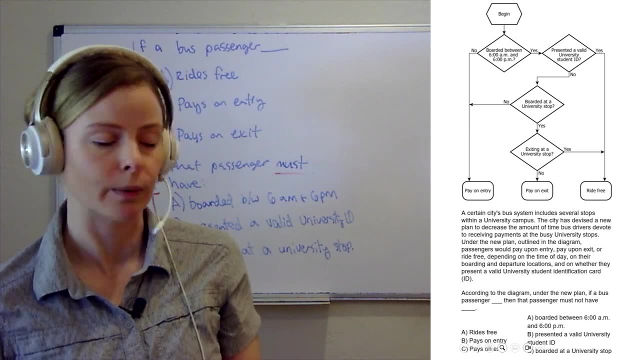 There is a way to make yourself kind of come back to that rides free bucket. That's where I'm going to leave it for now. I don't want to get too in the details until it is relevant to the option that I'm looking at. 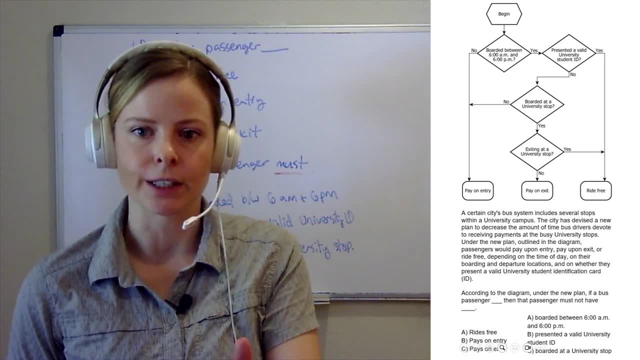 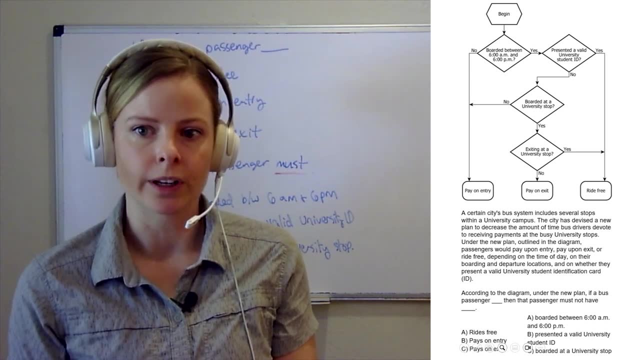 So again we're looking for, if they end up in the rides free bucket, what must not have happened. And let's go through our options. A: you must not have boarded between 6 am and 6 pm. Well, we just said that to end up in the rides free bucket, you have to board. 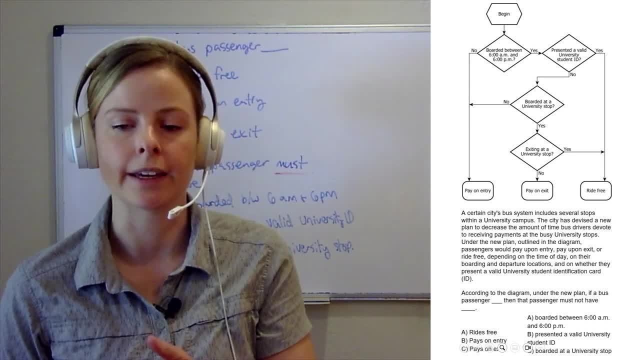 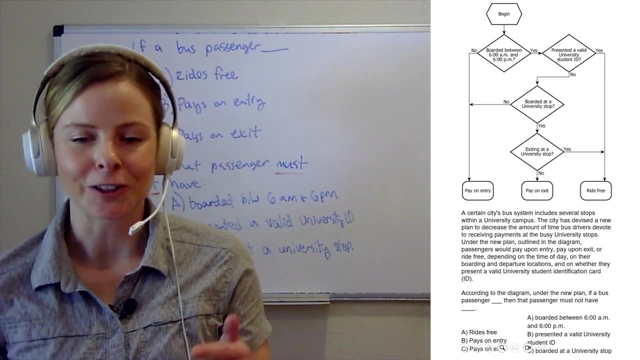 In that time, right. So this is the opposite of what we're looking for. So A is out B: you must not have presented a valid university student ID. Actually, on that first path, that pretty simple path it is, if you do present the ID. 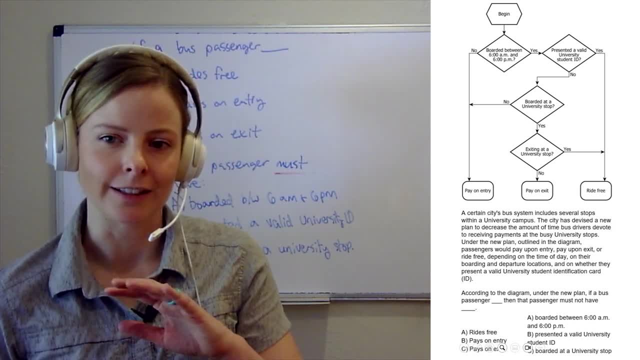 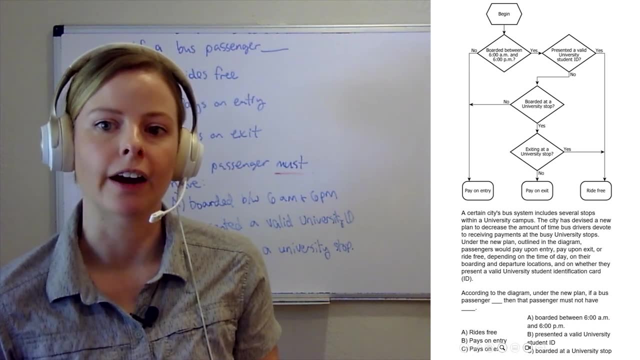 then you end up in the rides free bucket. So B is not, A must not. We can get rid of B. And then finally C: the passenger must not have boarded at a university bus stop. So this is where we kind of look in those weeds. 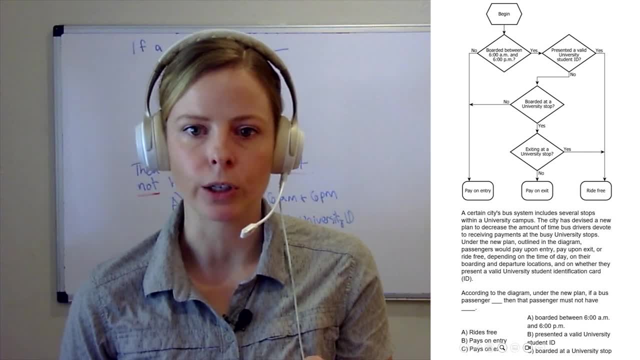 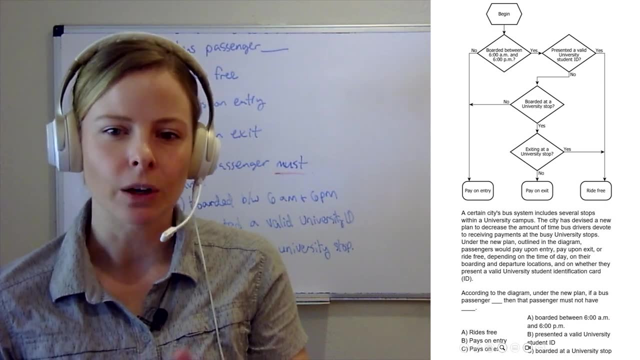 In those weeds, In those details? The boarded at a university bus stop is in the middle column, That first flow bucket thing. So let's answer yes to that question in C. Hey, can we actually ride free when we board at a university bus stop? 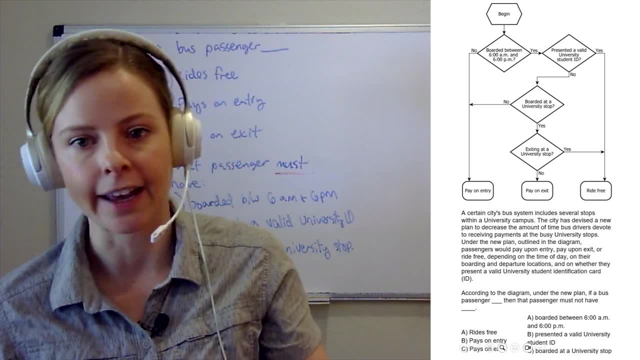 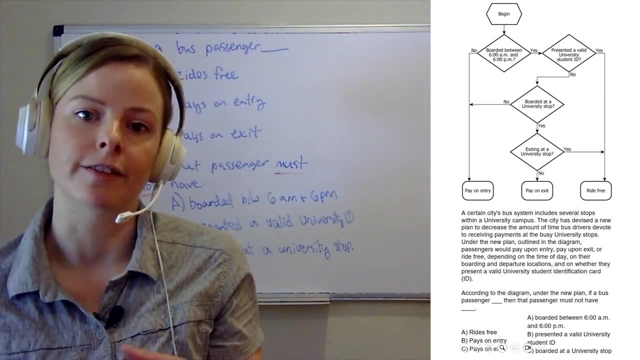 So if I answer yes, then I go down to the exit at a university bus stop. If I answer yes to that, I end up riding free. So again, we're looking for something that must not be true. And because there is a way for that to be true, then C also does not work. 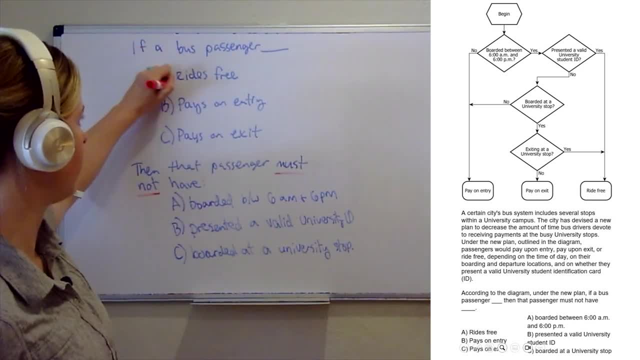 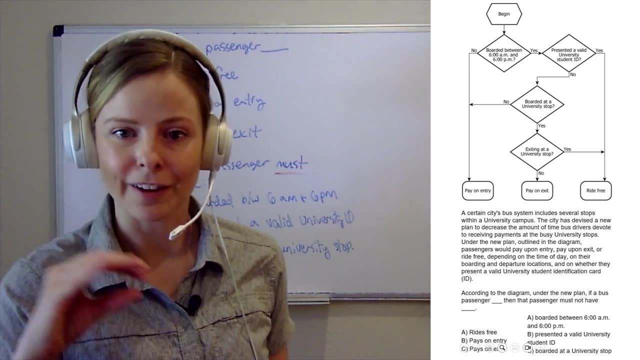 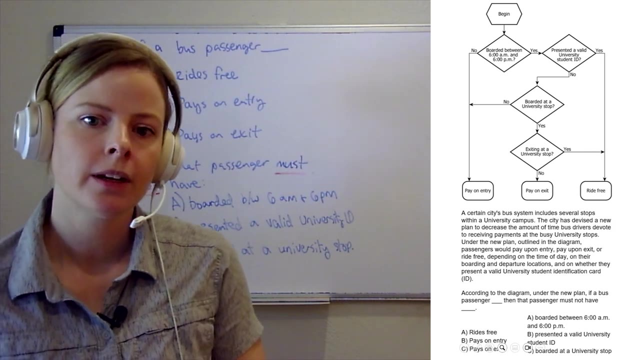 In other words, we have zero things that work with the rides free option, So we know for a fact that the rides free is incorrect. Let's look at our other kind of like end of the day outcome, buckets, So pays on entry. Let's again look at the chart. 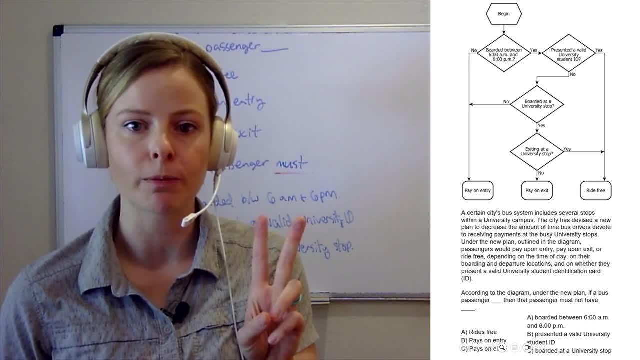 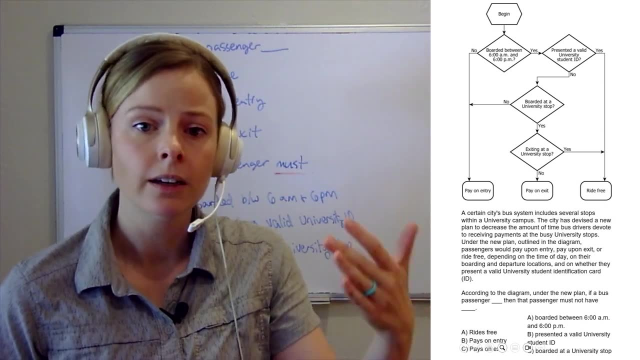 So to end up paying on entry, it looks like again we've got two paths. There is one path that says that you don't board between 6 am and 6 pm, So you board sometime at night. You've got to pay on entry. 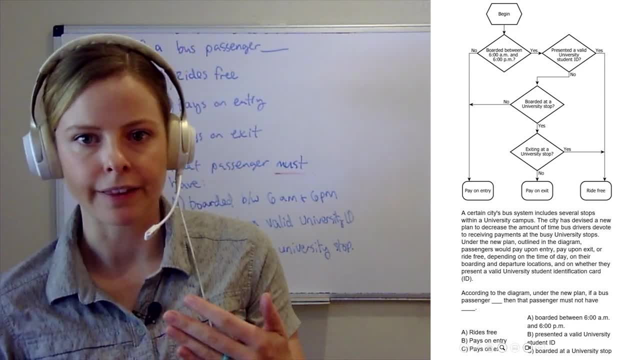 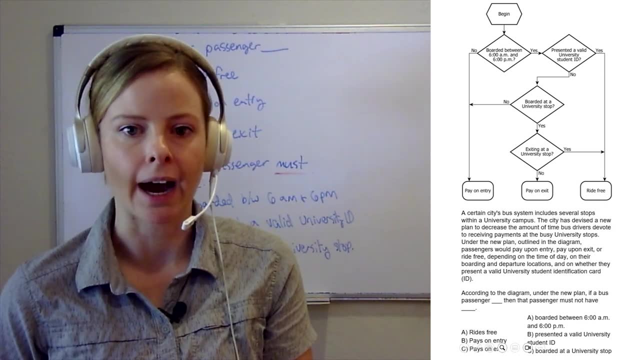 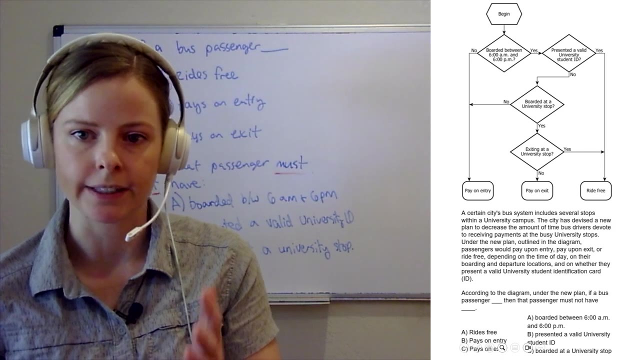 And then there's another path that goes all the way through this convoluted thing, you know, with the ID and with kind of where you're entering and exiting, and it's possible to make your way back to pay on entry. So with that in mind, let's see if there are any things that work for the second blank. 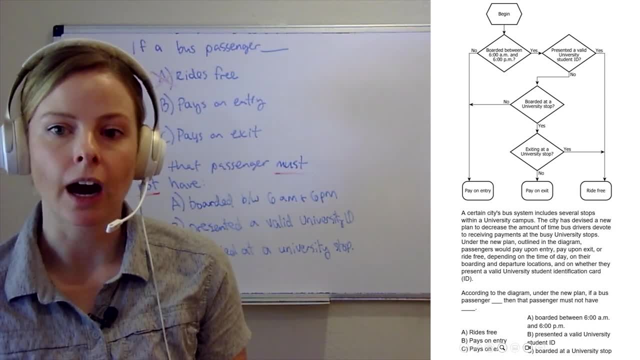 with pays on entry. So passenger must not have boarded between 6 am and 6 pm. Well, we just said there's two pathways, right? One is, if you answer no, you're not going to be able to board between 6 am and 6 pm. 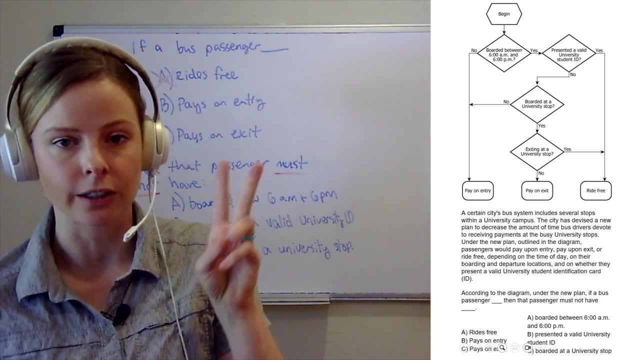 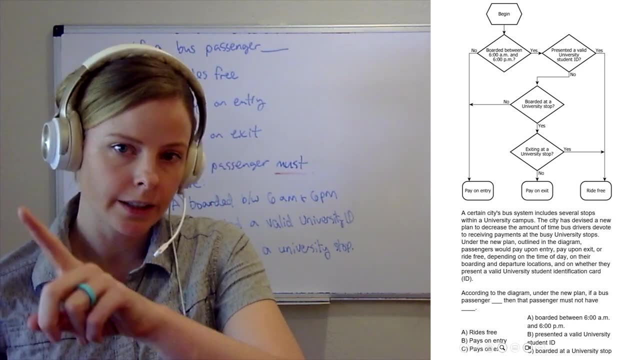 Right, So you answer no to that question. But the other is: you answered yes, right, So you did enter between 6 am and 6 pm and you make your way back to the pays on entry bucket. So because there's a pathway back, then we know that A is an R1,, right? 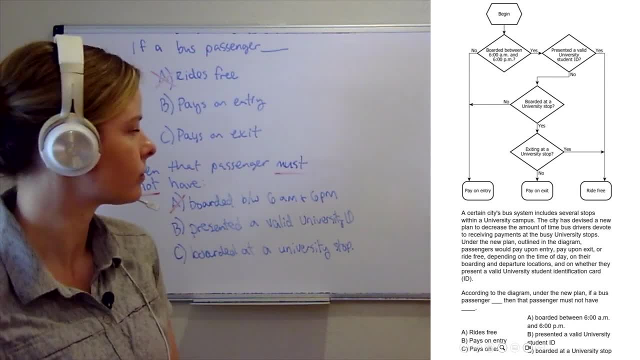 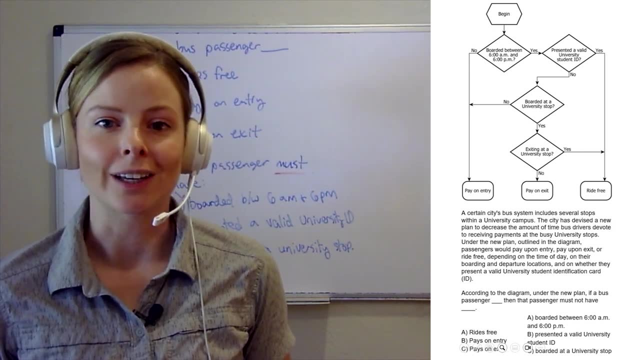 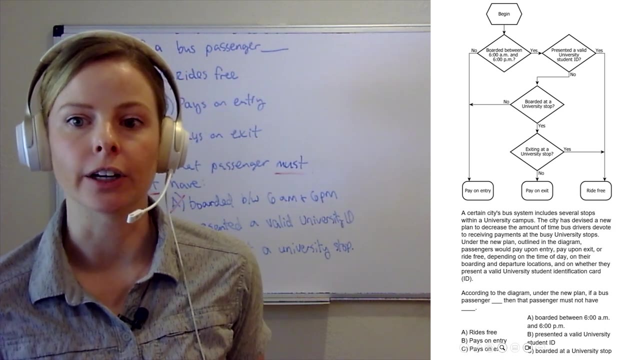 You can board between those times and pay on entry B must not have presented a valid university student ID. This one's a little tricky, I think, because that first path that we talked about, where you board at night, it just doesn't talk at all about your university student ID. 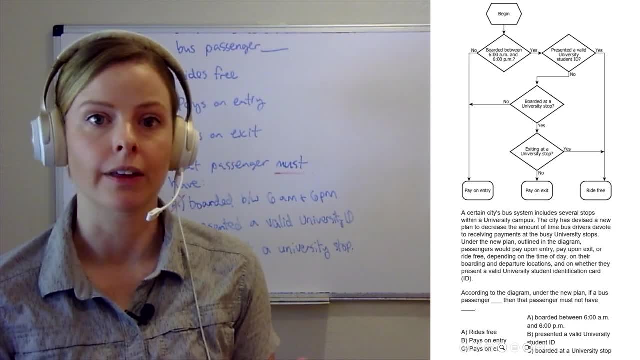 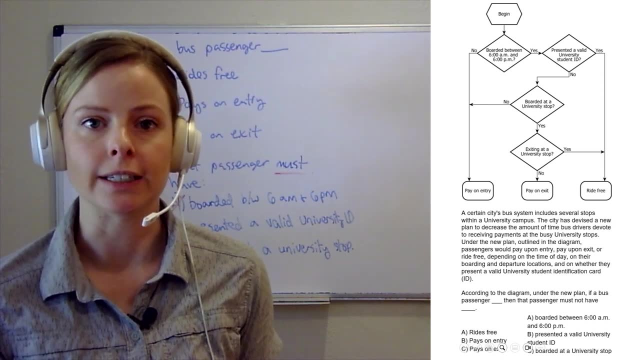 So for those people we just don't know, Are they presenting it, Are they not? It's just irrelevant. They all have to pay on entry, So you could imagine a student getting there at 7 pm. they show their student ID. 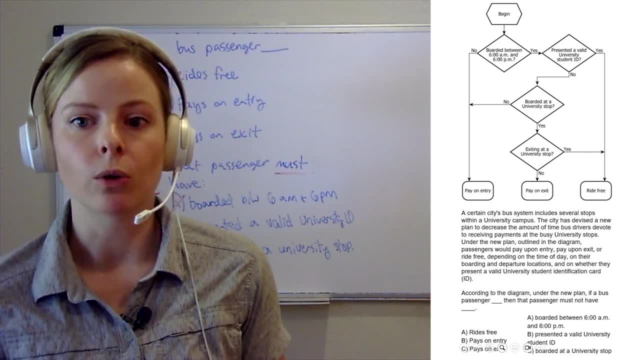 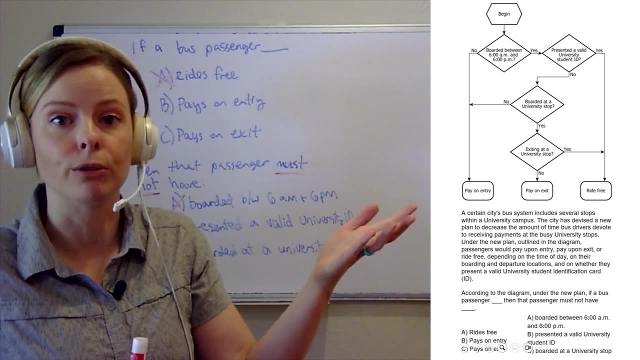 Guess what They still have to pay on entry. So this one is out because it could be true or it could not be true, We just don't know for those night riders, because it just doesn't go through that bucket at all. So that doesn't work. 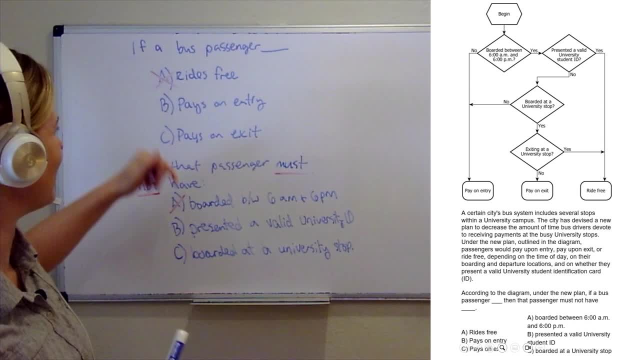 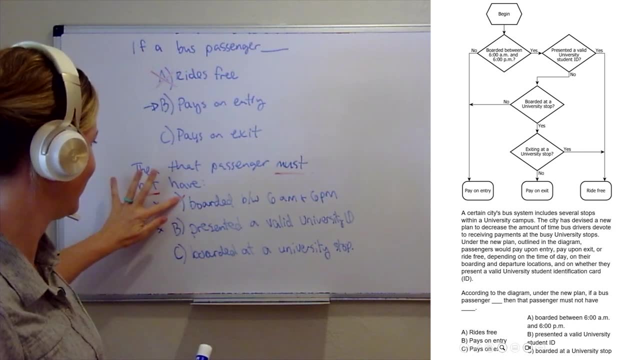 I'm doing this in a confusing way. Right now, we're talking about pays on entry. We know that A is not going to work. We know that B is not going to work. I'm going to, for clarity's sake, get rid of that. 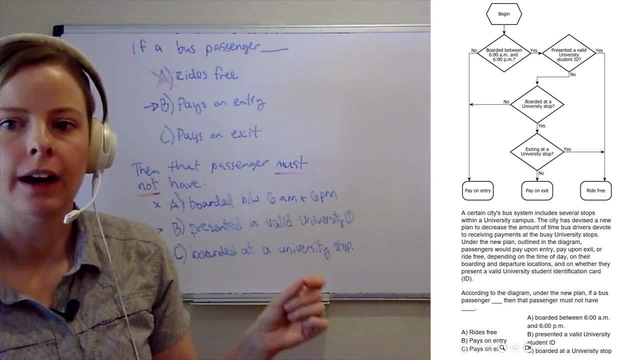 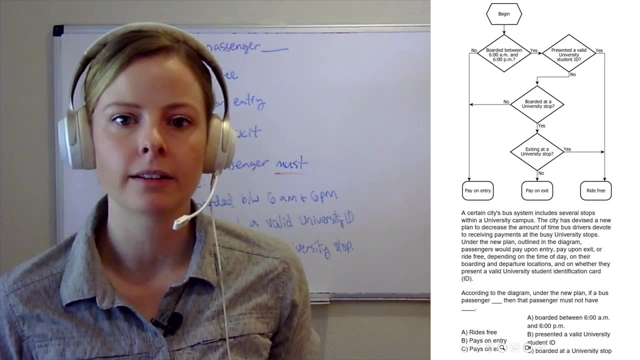 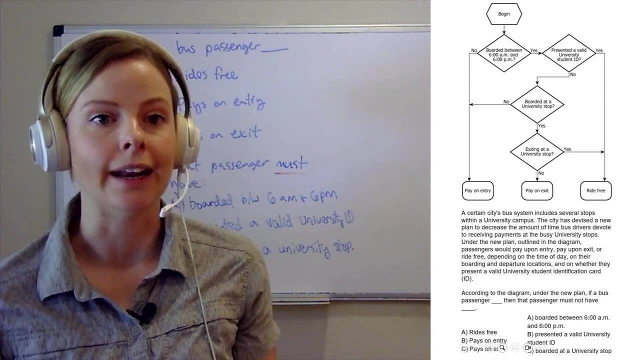 Let's look at C. So to end up paying on entry, the passenger must not have boarded at a university stop. Well, let's again go to our pathways. This falls into that same category as B, So for the people who are boarding at night, 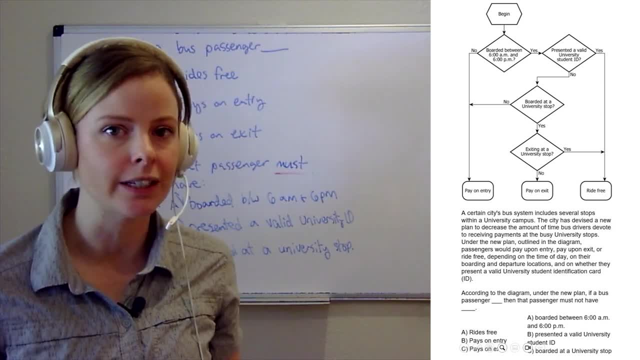 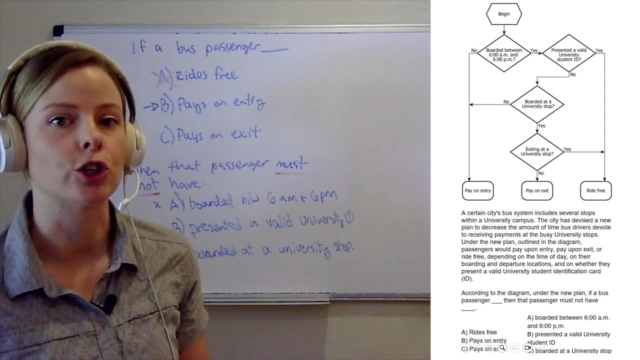 where are they boarding? I don't know. I don't know. It could be at a university stop, It could be at a non-university stop. We simply don't know where they are boarding and yet they're having to pay on entry every. 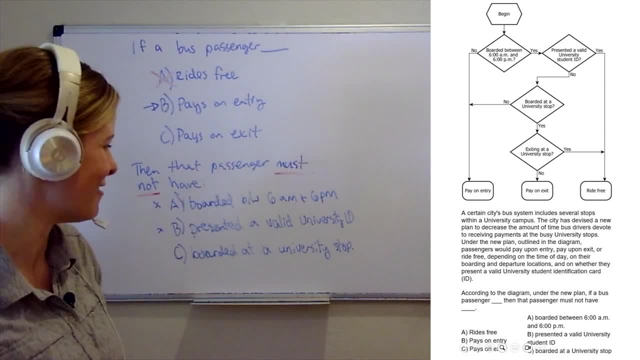 time. So it's not true that they must not have boarded at a university stop. We don't know where they're boarding if they're boarding at night, So C is out, which means that there are no options that work with the pays on entry. 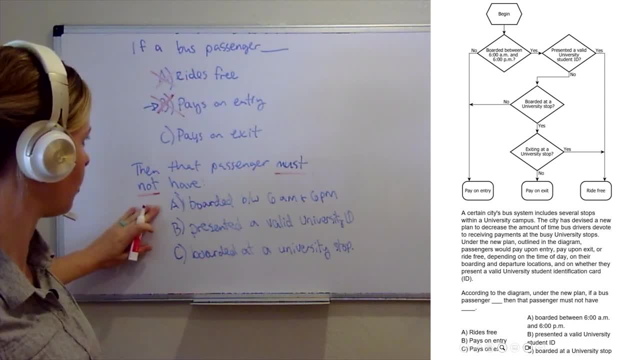 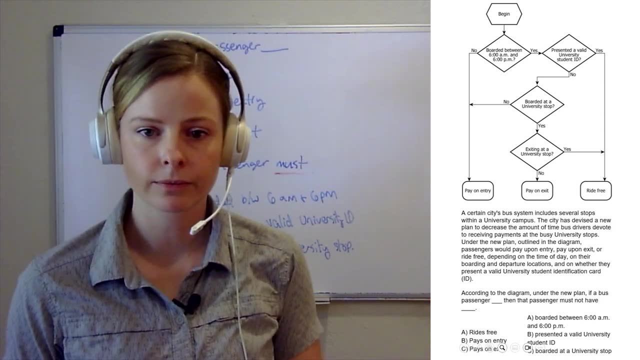 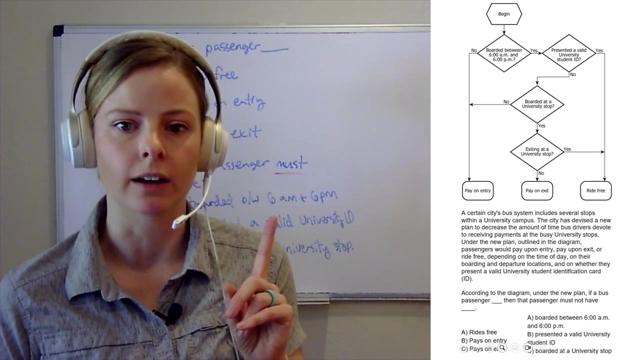 Pays on entry blank for one. So hopefully there is something that makes sense for pays on exit. Let's take a look Again, going back to the flowchart. Looking at this flowchart, there's actually only one path to get to pay on exit, which? 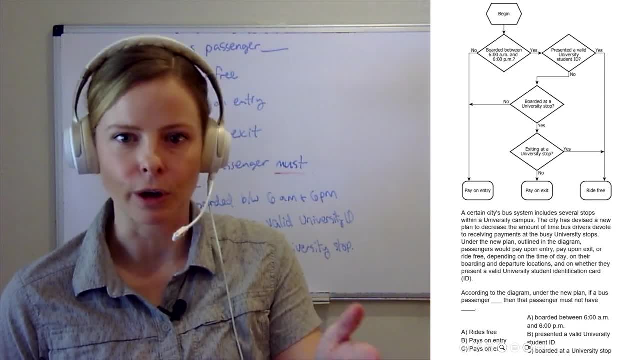 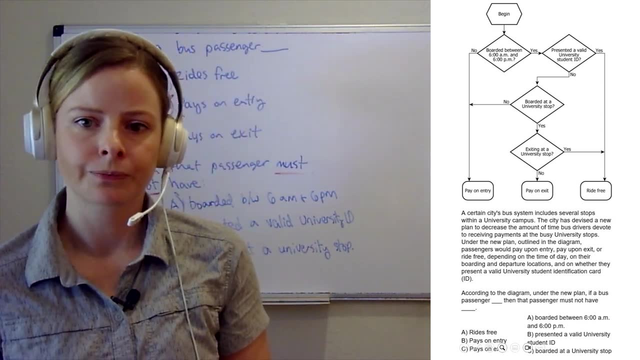 is nice. It makes your life a little simple. You have to go through a very specific set of events- yeses and nos- to get to that pay on exit. So To pay on exit, the passenger must not have boarded between 6am and 6pm. 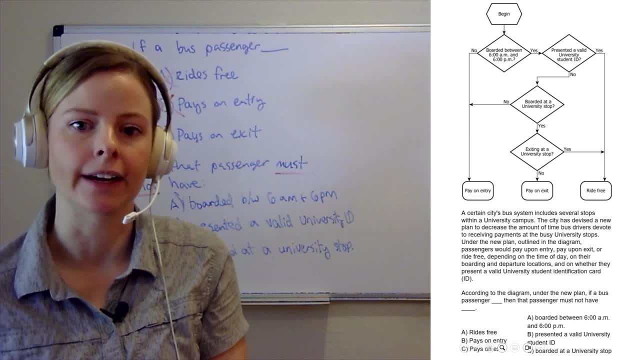 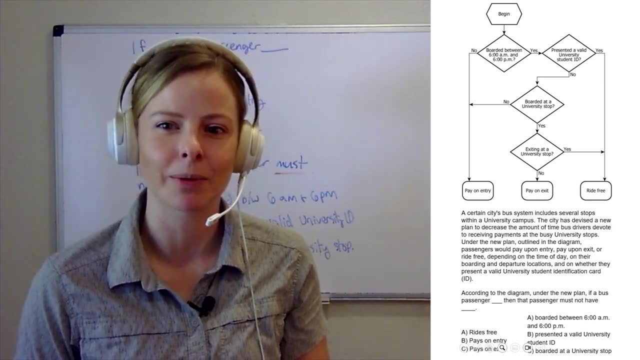 Well, if we look at this one path, the only way to get to pay on exit is if you do board between 6am and 6pm, So the must not really messes up here. it's the opposite of what we want. 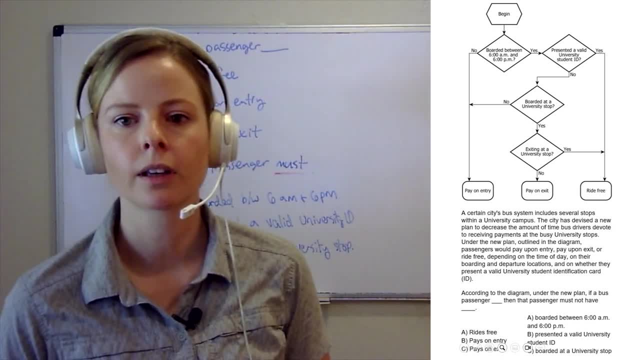 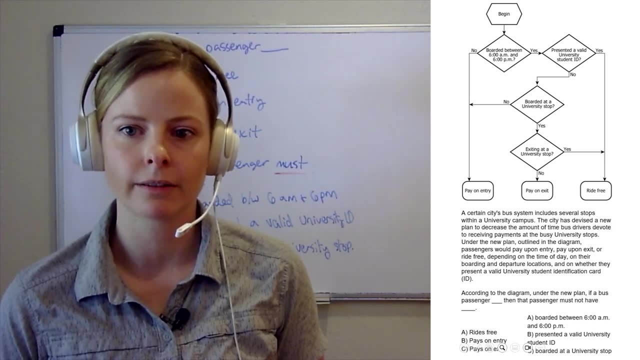 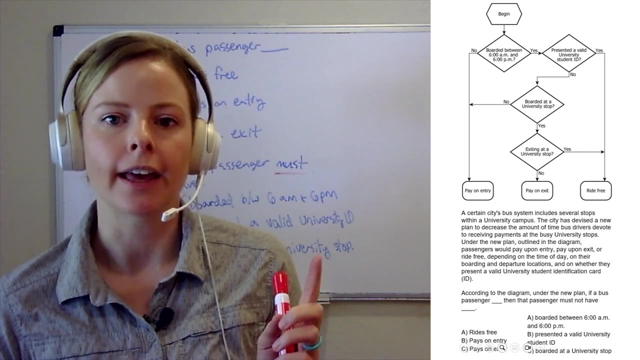 So that cannot be true. To pay on exit, the passenger must not have presented a valid university student ID. Well, let's go ahead and look at our one pathway, the only thing that possibly works, and see what happens with the ID situation. 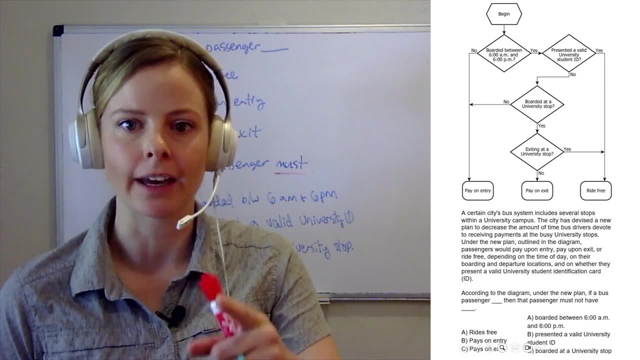 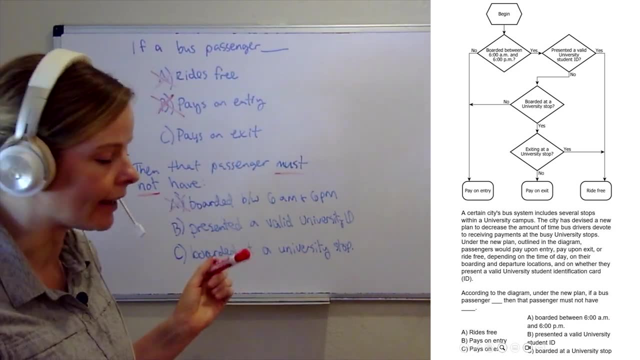 You have to answer no. That's the only pathway. and it's a no on that university ID question. So in order to end up paying on exit, you just cannot present a student ID. So that is why B is going to be our correct answer. 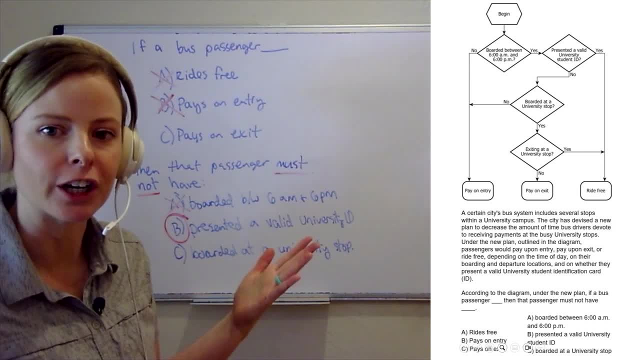 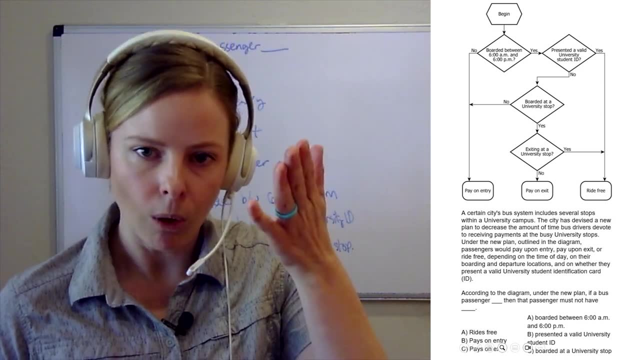 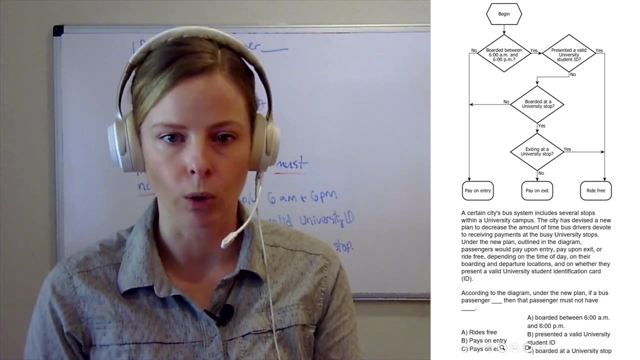 And if you just want to, you know, just make sure. Is it that the passenger must not have boarded at a university bus stop? Well, again, the only pathway says that you have to answer yes to that question, right? So you actually do have to board at a university bus stop in order to end up into the pay on. 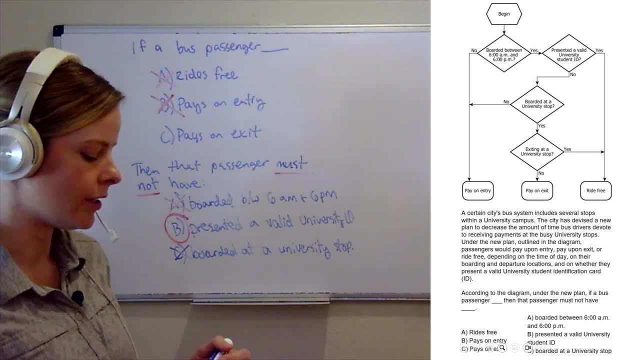 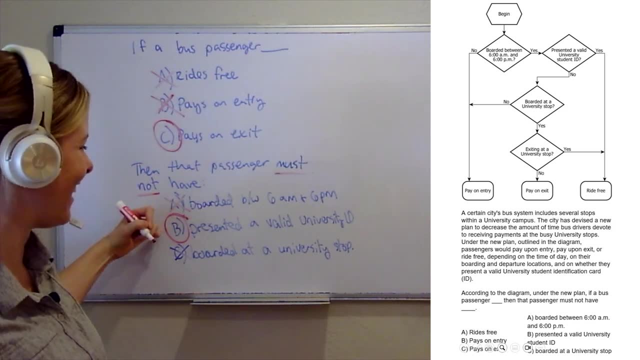 exit bucket. So C is out, And what we get here is that you must answer B for your first sorry, C for your first blank and B for your second blank, And that is the correct answer to this question. So that's the answer. 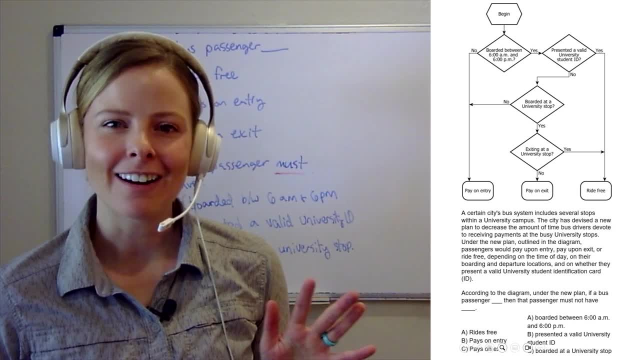 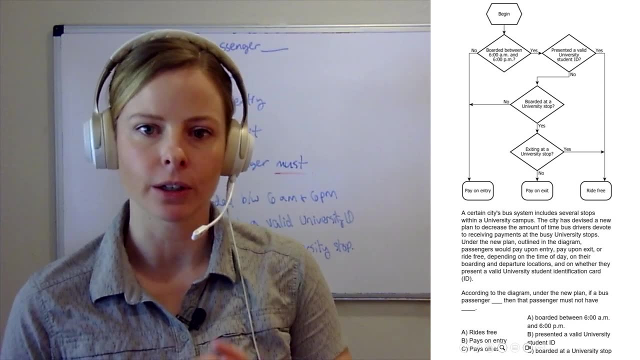 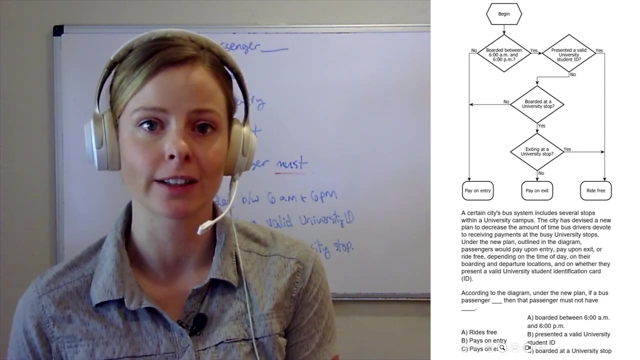 So that's the answer to this question. So when a graph or a chart pops up on the screen on your data insight section, all you want to do is give yourself time to really understand the big picture of that data before you go ahead and dive into the exact questions. 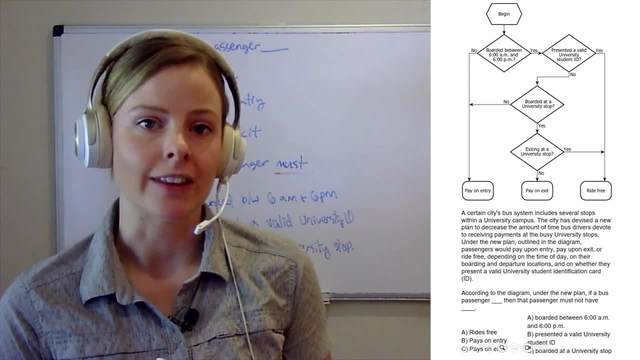 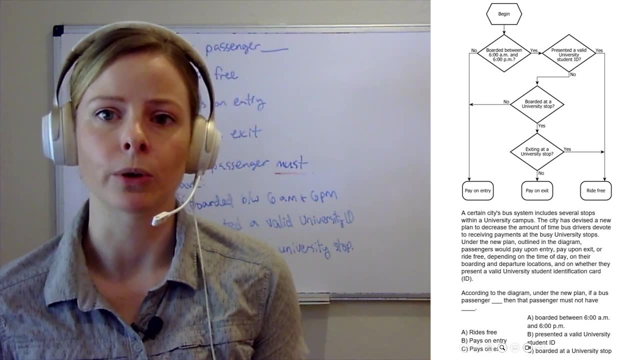 So that's going to involve looking at the description of the graph, looking at the axes on the graph, any keys, that kind of information, and then maybe tell yourself a bit of a story. Pick a data point to see if you can. 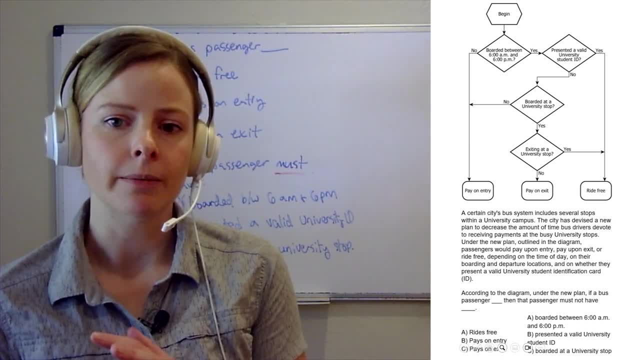 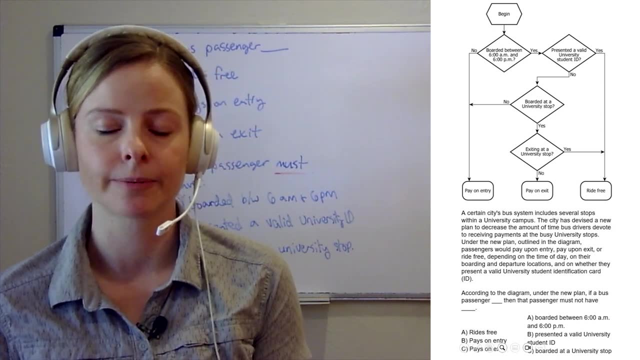 Understand what's happening at that data point, just to make sure that you're really grounded in what that information is telling you before you dive into the specific details of the question that is asked. This is Dana with GMAT Ninja, and I hope you have enjoyed this video and I will see you.